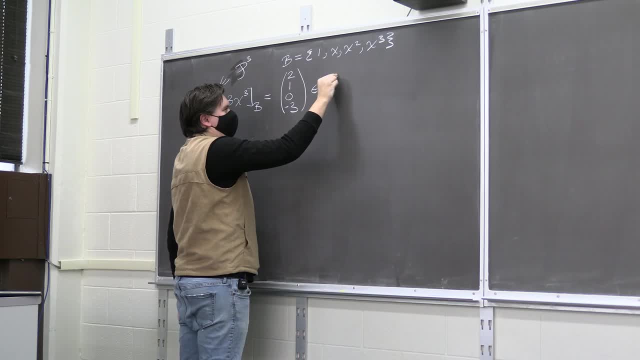 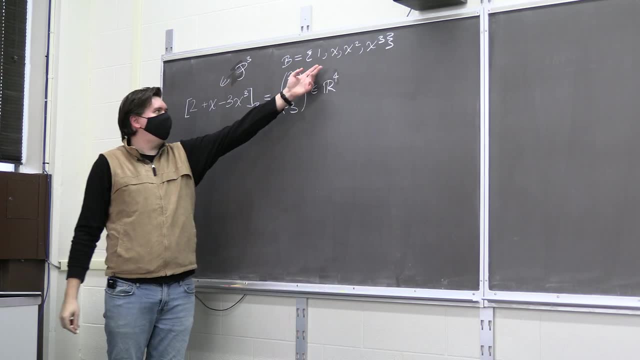 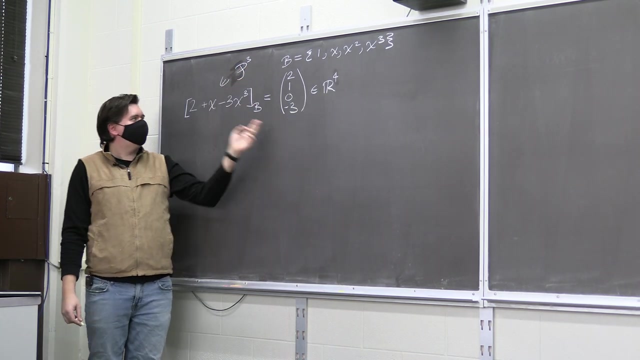 that lives inside of R3.. No, it doesn't. It lives inside of R4. This is a four-dimensional vector field, And P3 is a four-dimensional vector field over the ground field of R, And so when you express it with the coordinates, the coordinates are just going to live in R4.. If this was the polynomial, 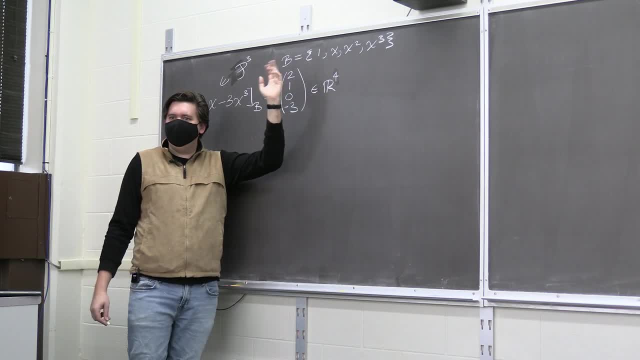 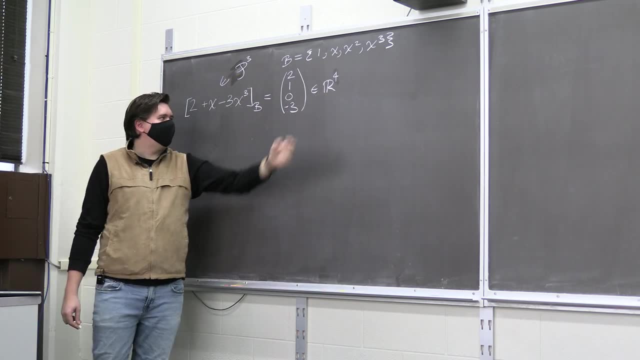 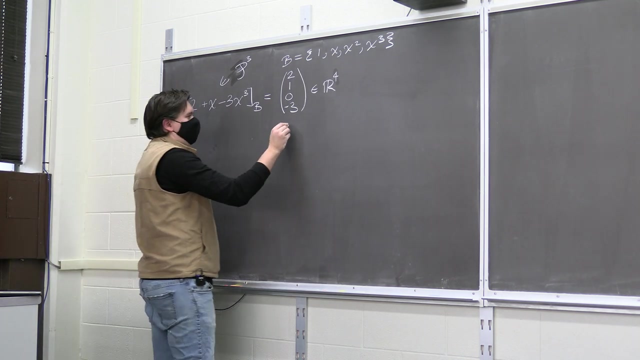 of complex coefficients. it would just live in C4, right, So that's not a problem. Whatever your ground field is, whatever your scalars are coming from, that's where this guy is going to live. But then we did last time. we continued and we said, well, there are other bases we could have. 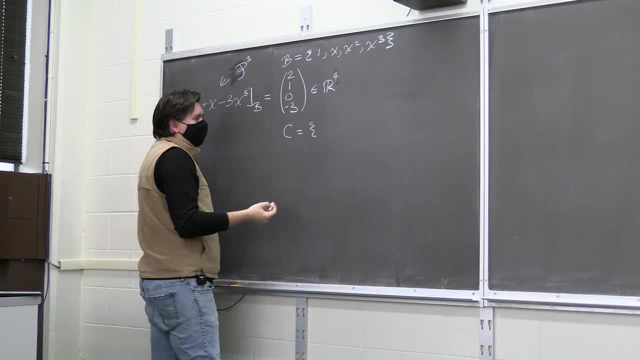 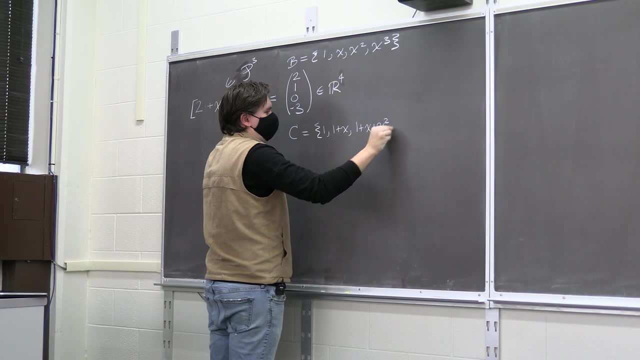 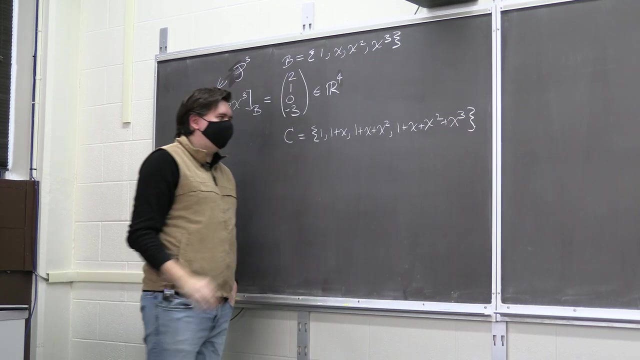 chosen. So another basis, for example, that we could have chosen is the one that's 1, 1 plus x, 1 plus x plus x squared 1 plus x plus x squared plus x cubed. And in previous lectures, 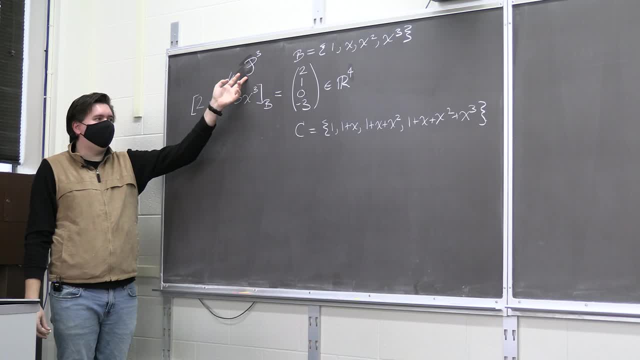 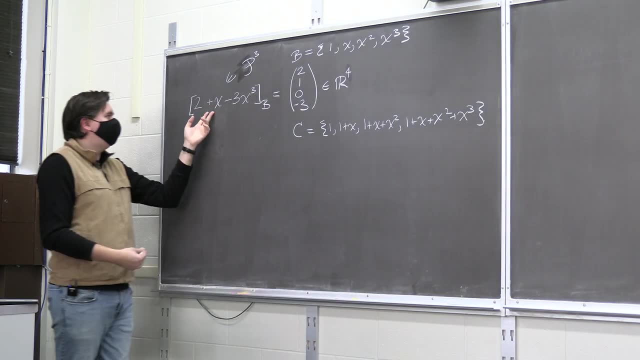 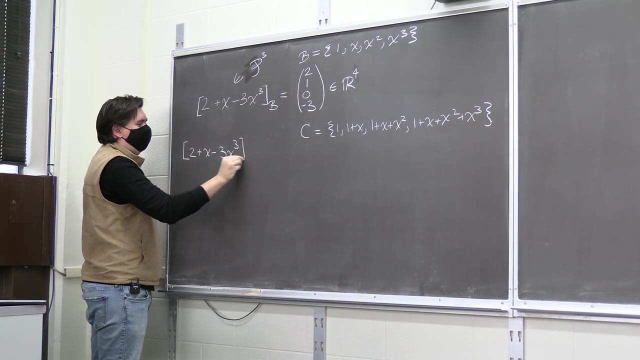 we verified that. In fact that is a basis for P3.. Any polynomial of degree up to 3 can be written as a linear combination of these guys. And we did that. We took this vector, we took the vector two plus x minus three, x cubed, and we figured out what it would be if you write: 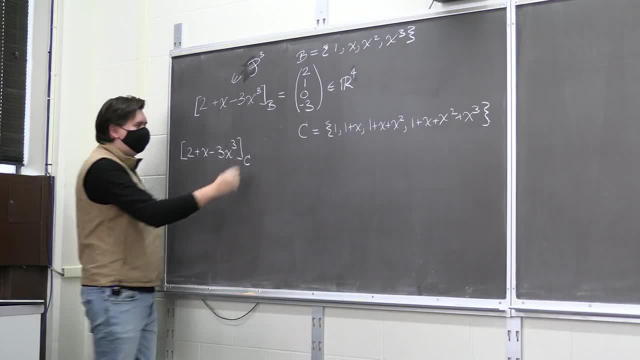 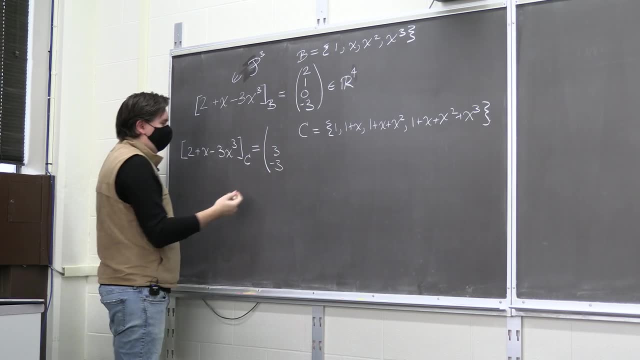 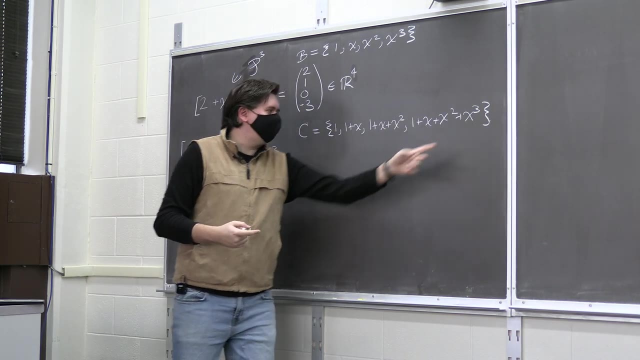 it as a linear combination of these guys and we read off the coefficients and those coefficients came out to be: oh, let's try remember, a negative three, three. um, you need a negative three here in order to get- uh, this coefficient of this guy has been negative three in order to get negative. 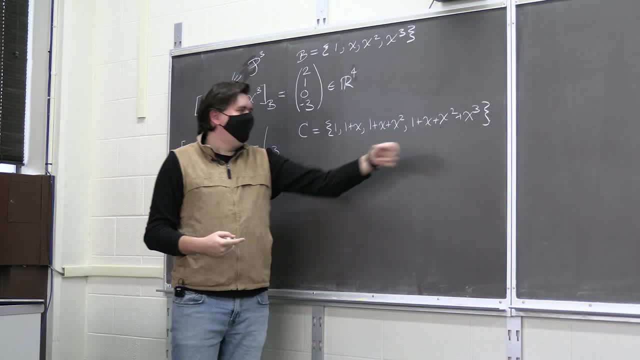 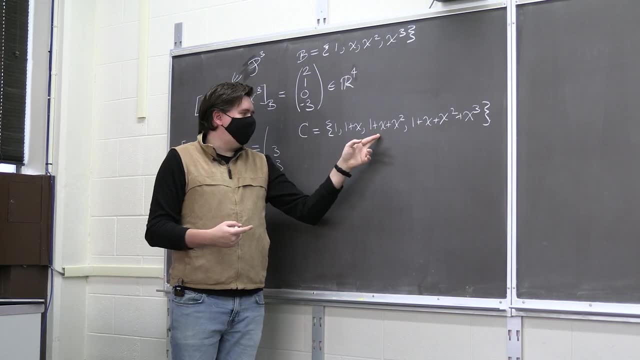 three x cubed, but then also gives you a negative three x squared which you cancel by making a three the coefficient of this guy. so then you get three x squared and now you have negative three x's and three x's, so zero x's. so you want one more x, so this should be a one, but now you have negative. 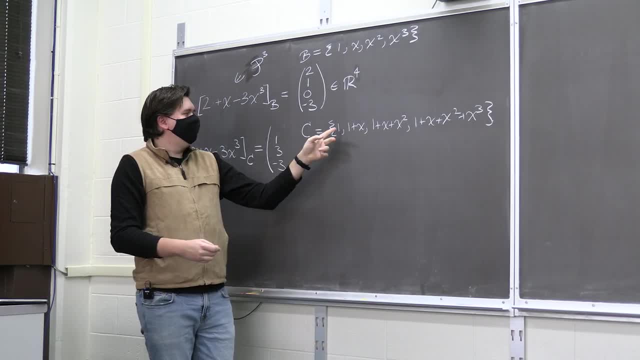 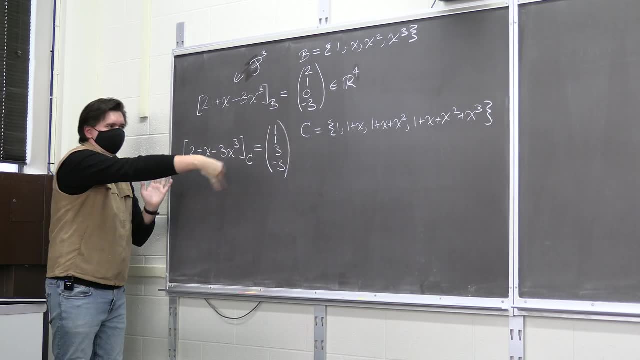 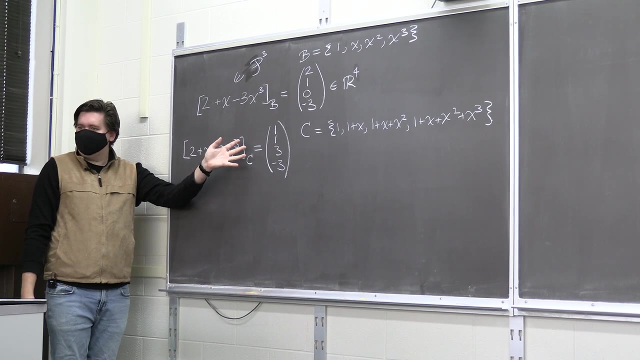 three ones, three ones and one one. so you want this to be another one. so your constants add up to two. we did this last time. you can just solve the system of equations. what linear Combinations of these guys give you this vector, and I'm pretty sure it came out to be this. Yeah, 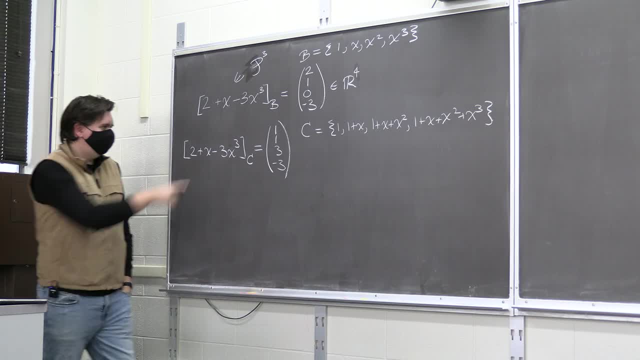 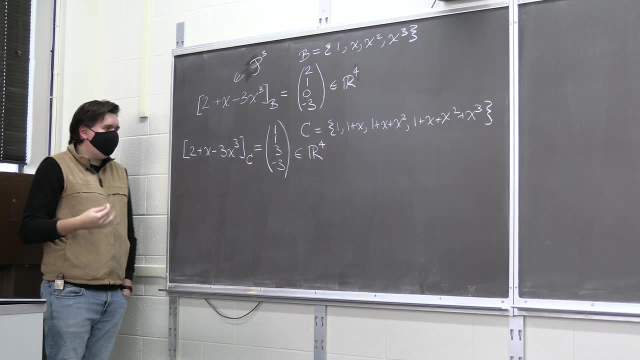 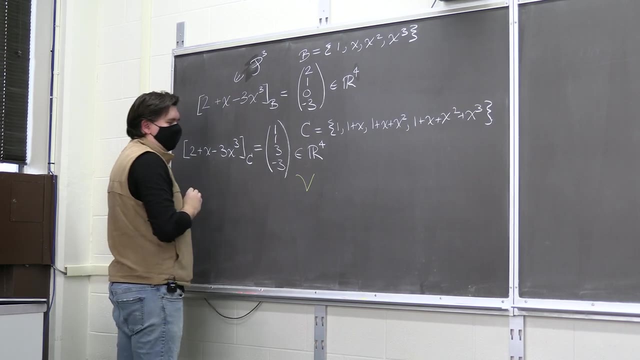 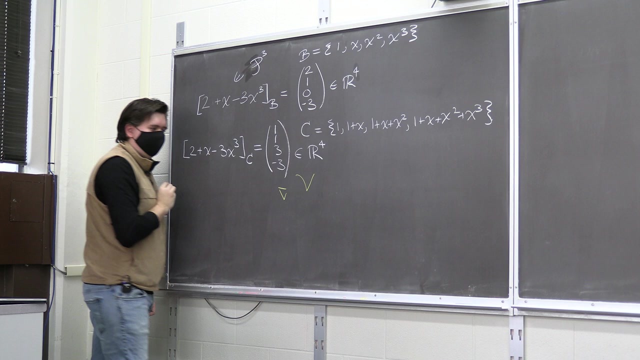 Okay, great, which is also a vector in our form. so perhaps the picture you should have in mind then is We're starting off in some vector space. in this particular example, this vector space is P 3, and in that vector space we have some vector V and 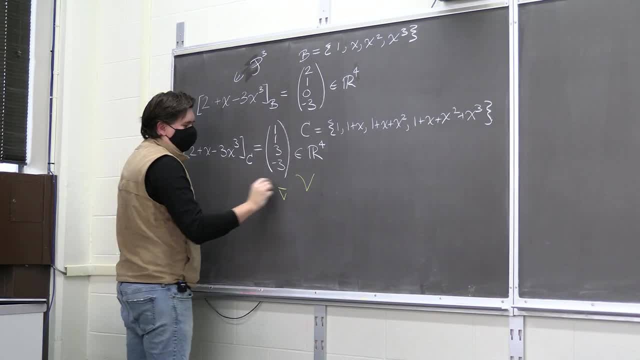 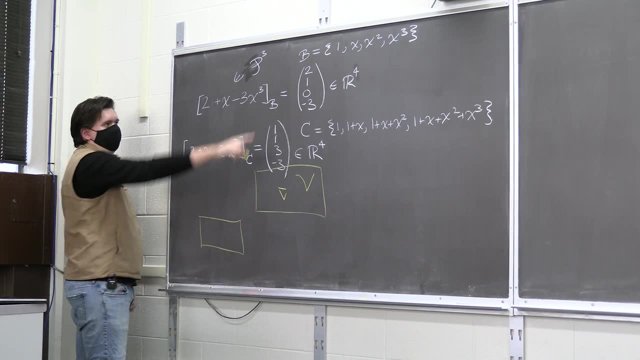 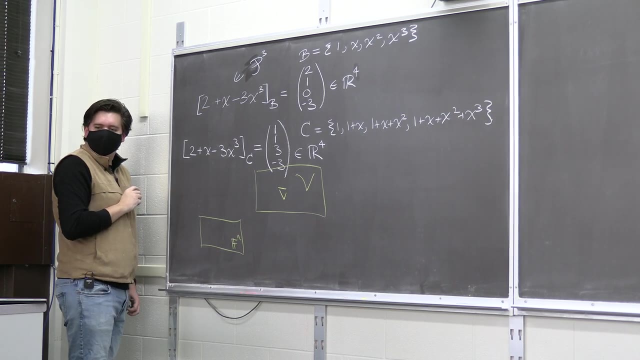 then what we're doing is we're moving from belonging inside that big vector space V to living inside of a Copy of- well, for us are four, so whatever, whatever your ground field is to the dimension of your vector space, and So we're sending- let me, let me draw a different color here, so it pops out- We're sending V. 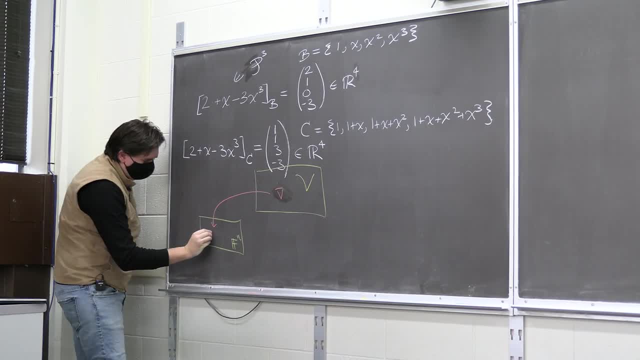 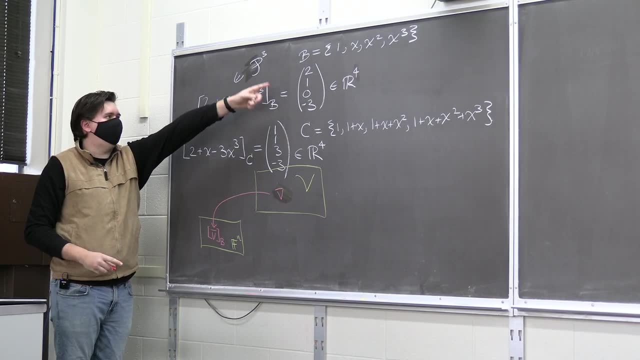 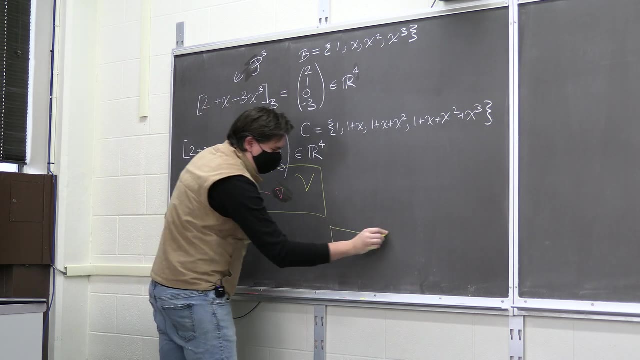 To some coordinate vector here, right, And so we're turning V into whatever the corresponding coordinate vector is here. That, that was turning him right here into two, one zero negative three. but then you might think: well, we did it again, But a slightly different map. so we still sent it into F? n. 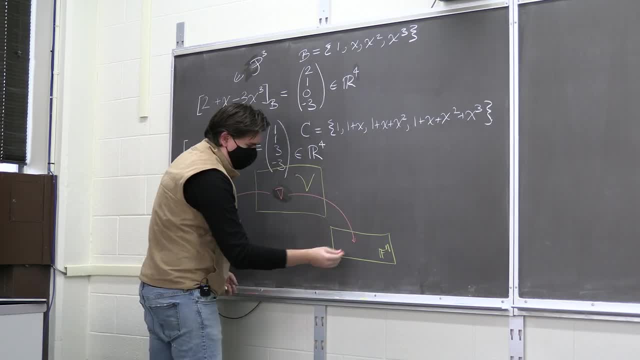 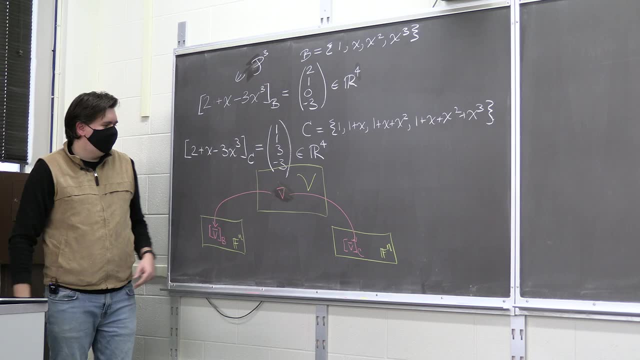 But this time with respect to a different basis. So now you have some other Vector V turned into some other basis, see, So so you can map it down to a copy of F? n, or you can map it down to copy of F? n, You get different vectors. 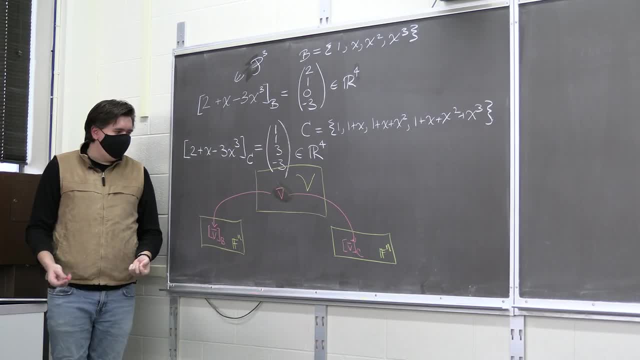 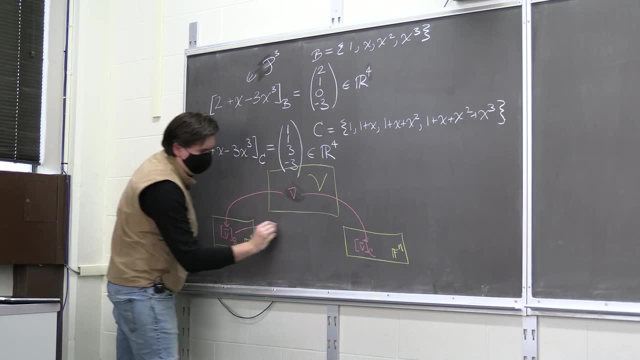 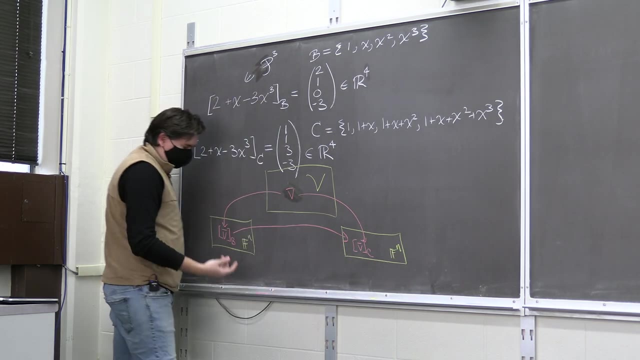 What we want to talk about today is what? is there a way to move directly from one of these to another one? Right, how can I move From here to here? What's a map from F? n to F? n that changes my basis? So what we're trying to figure out is a map that will perform. 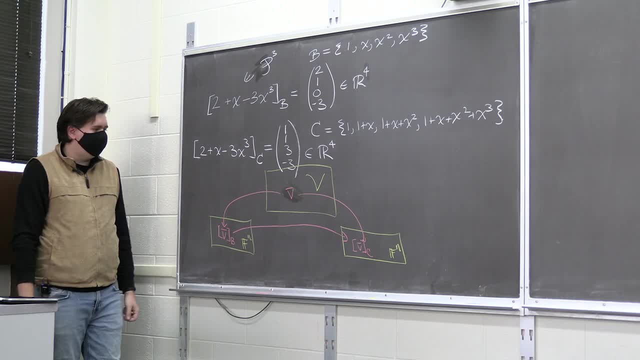 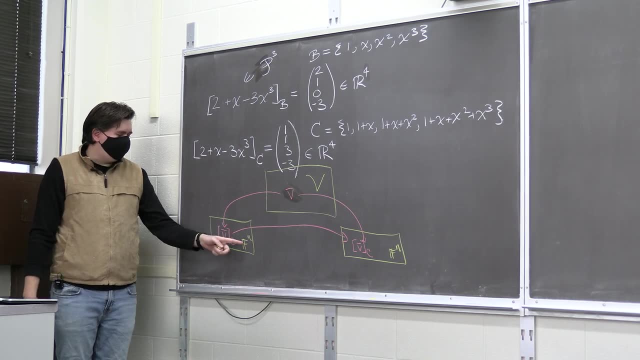 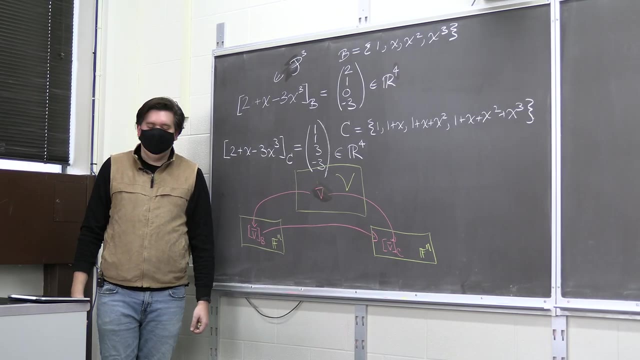 A change of basis for us, right? Okay, so Maybe, like this is a familiar story. How do we do a transformation from F? n to F? n? What's one way that's going to do that, Like from R n to R n? What's a map from R n to R n look like. 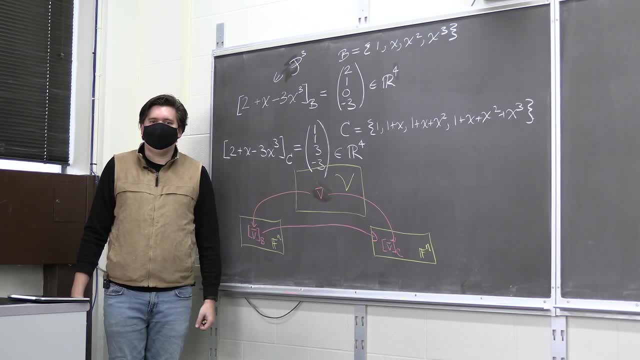 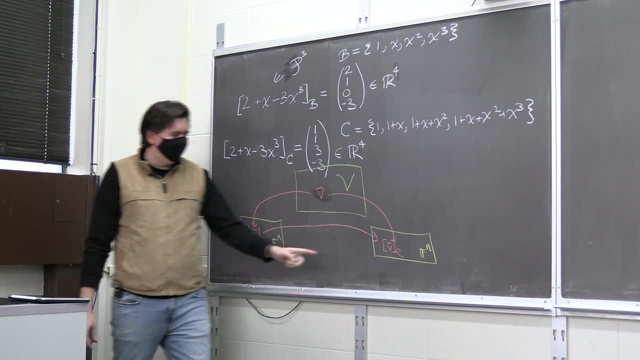 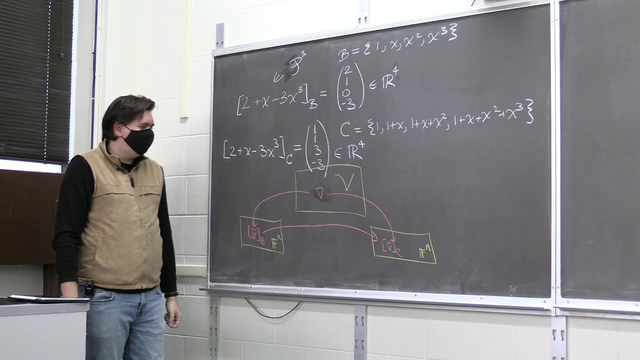 One you talk about in linear algebra, A matrix Right, it's like a matrix, an n by n matrix is a map from F? n to F? n or R? n to R n, more generally F n to F? n, where your coefficients are just coming from, whatever your, your field is. 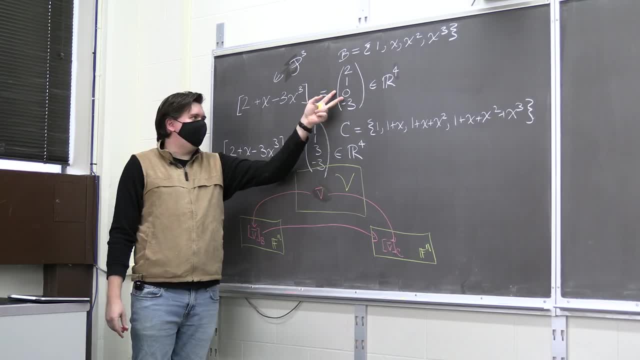 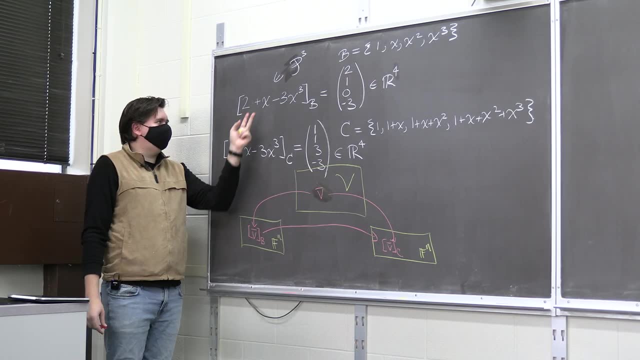 So can we think of a matrix that sends us from this vector to this vector, right? Well, there are lots of matrices, But, more generally, is there a matrix that sends us from, you know, this vector with respect to B to some other vector with respect to C? 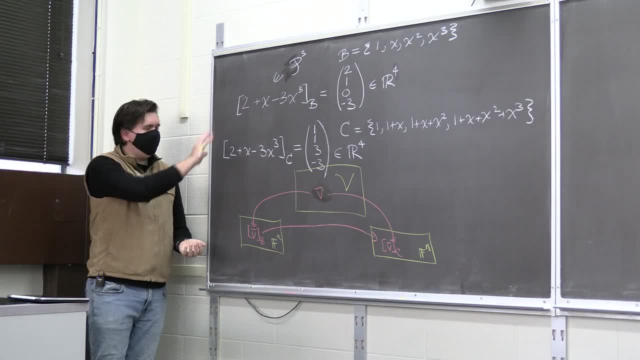 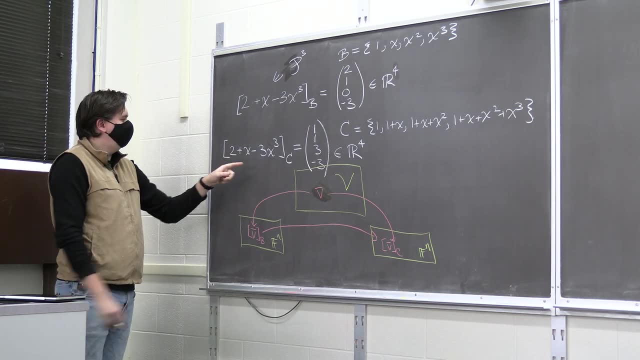 That's. that's what we're trying to figure out. So let's think of a little more about what's going on here. and one way to think about what's going on here is is: let's- um, let's start with this guy again and say that 2 plus 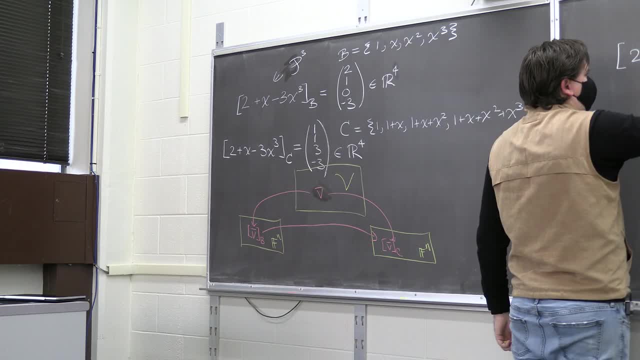 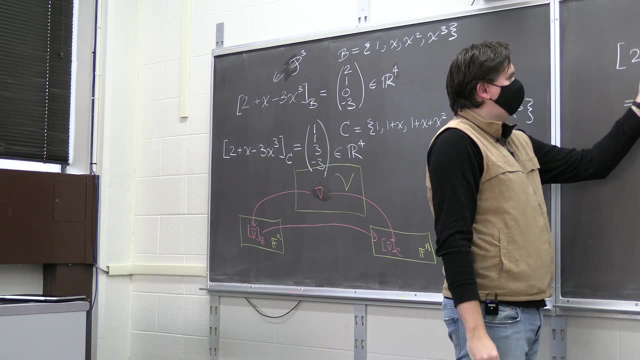 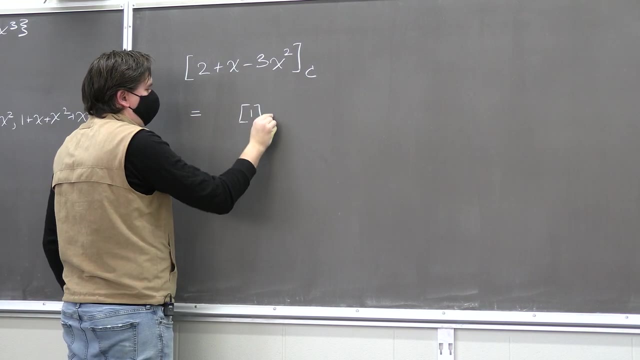 that x minus that 3x, squared in terms of C, we can think of as Well. in order to express this in terms of the basis C, it would be sufficient To figure out how to express 1 in terms of the basis C, How to express x in terms of the basis C. 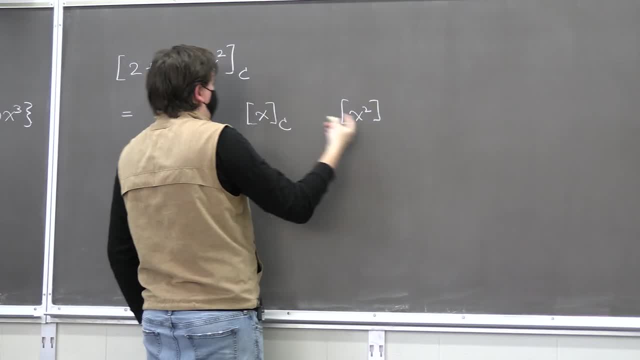 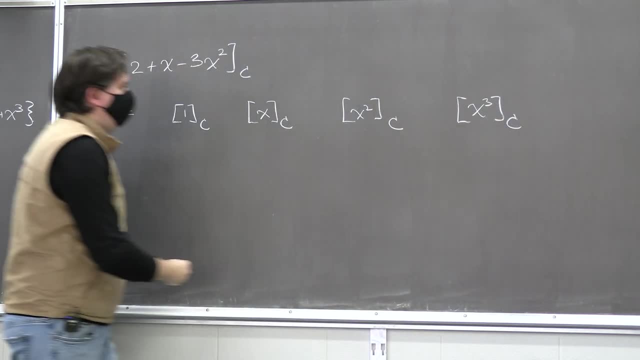 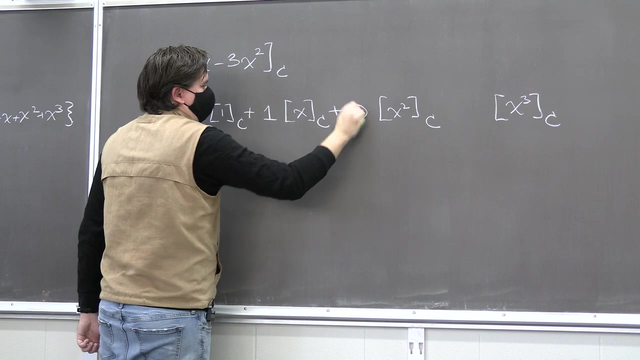 how to express x squared in terms of the basis C and how to express x cubed in terms of the basis C, and then take a linear combination of those two times the first one plus one times the next one, plus zero copies of this one plus negative three copies. 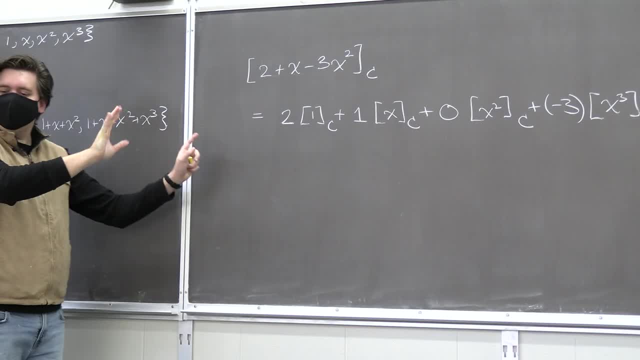 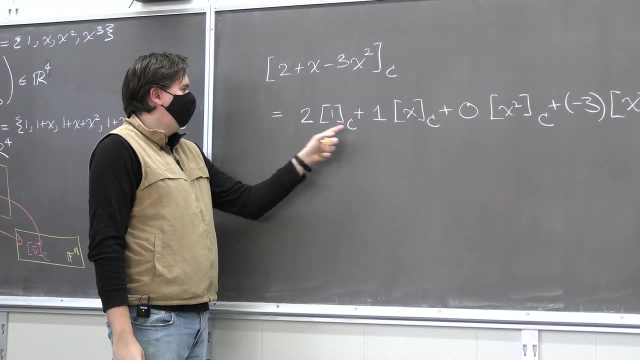 of this last one. Well, you need to take a minute to convince yourself. these really are the same thing. But, like you know, think: If you express something in terms of your basis C and you multiply that by two, you should convince yourself. 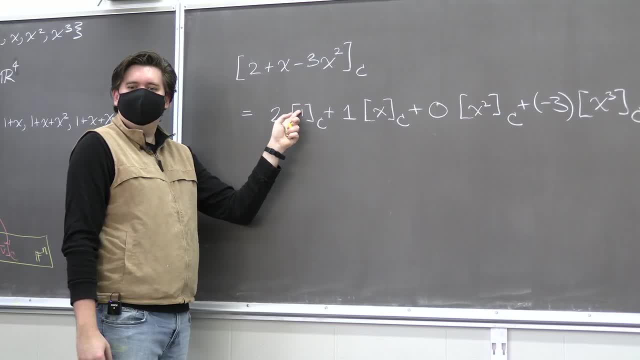 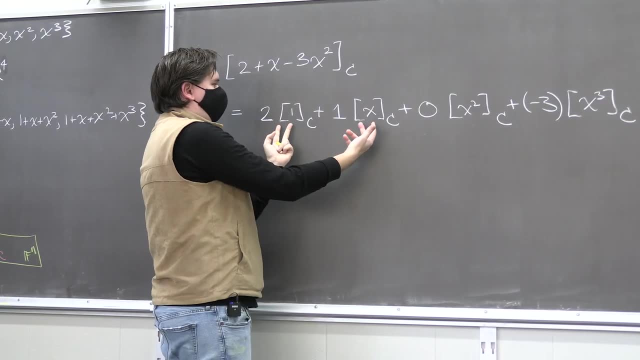 that's really the same as moving the two inside right. So like, take a second, think about how scaling works and agree: okay, that's fine And same, with addition That if you have some vector expressed in terms of the basis C. 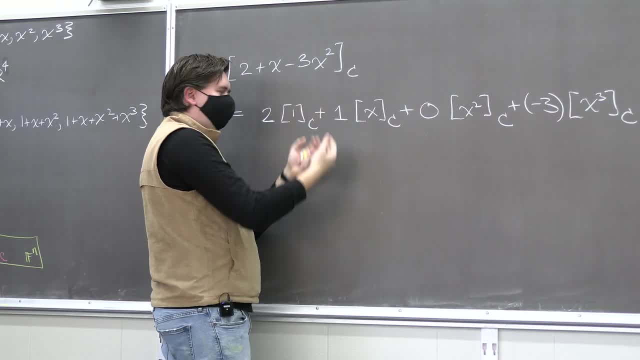 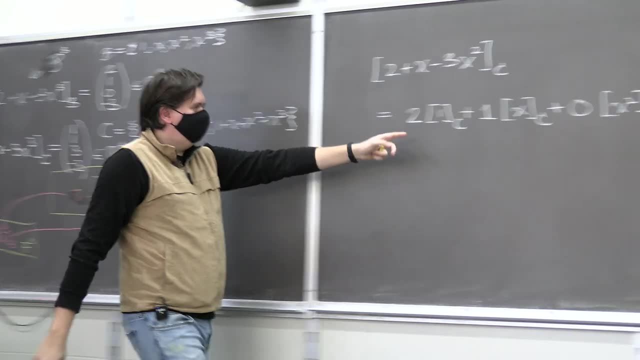 and some other vector in terms of the basis C and you add them together. that's the same thing as adding two vectors, then expressed in terms of the basis C. But I think that's pretty clear, since this is only going to come from just reading off. 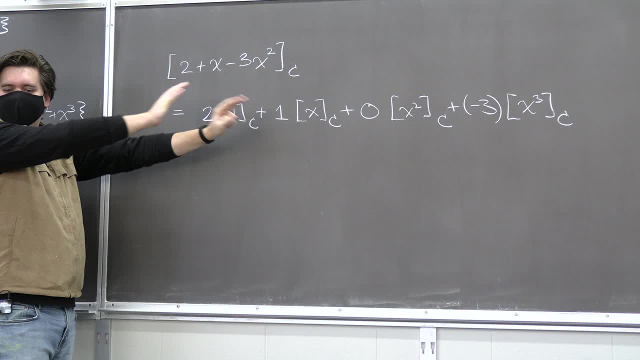 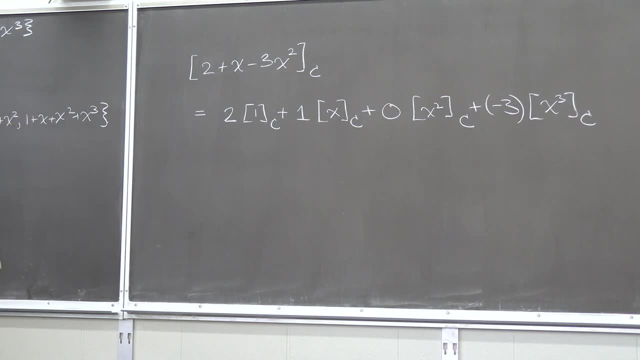 the coefficients of linear combination. So when you scale, you're scaling those coefficients. When you add, you're just adding those coefficients. So that should be believable, But you can convince yourself of that. Then it's like: okay, so what do we get? 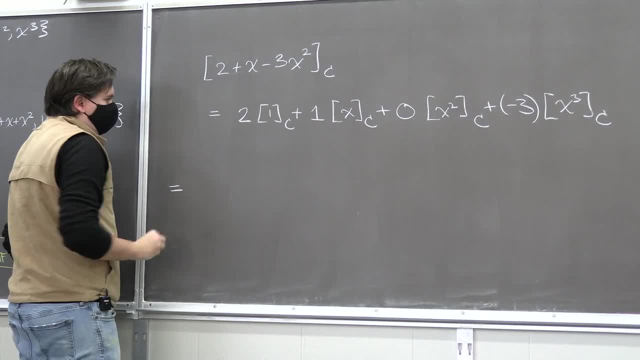 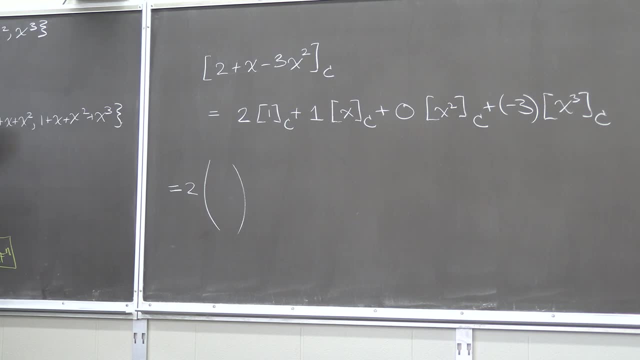 And well, we could just calculate this. So, if we want to just calculate this, you're like it's two times what is one in terms of that basis C? How do I get one in terms of this basis? Well, it's right there as one. 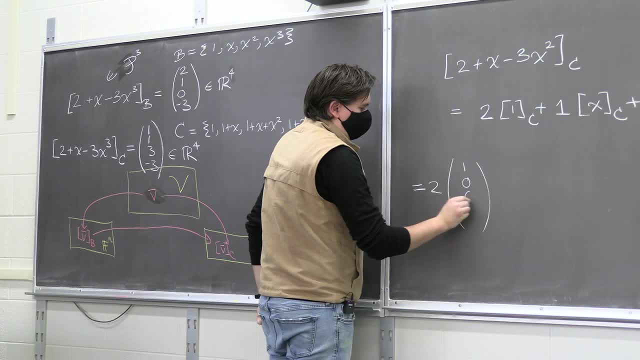 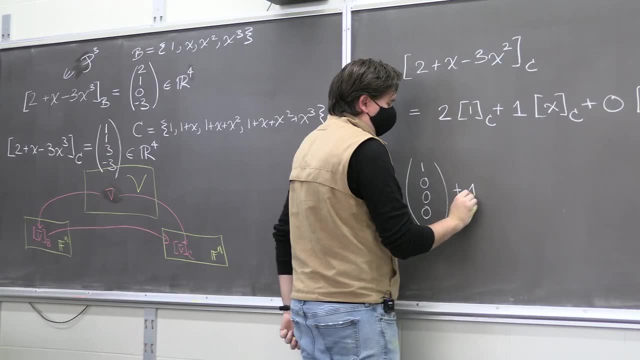 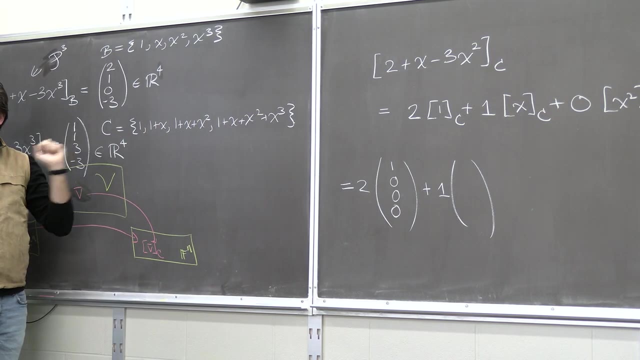 So one copy of the first guy and zero copies of everything else, right? How do I write X In terms of this basis C? How do I write X in terms of that basis C? Yeah, you want a copy of this second guy. 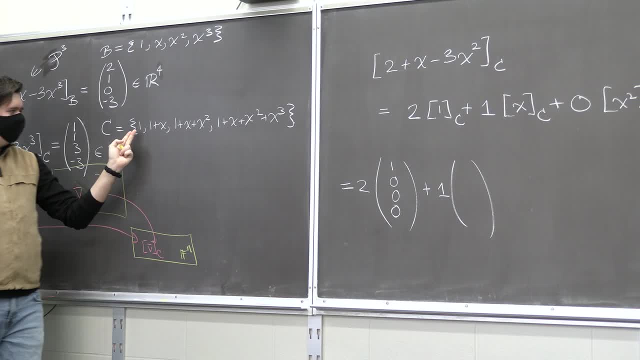 but then you have a plus one you need to get rid of. So you need negative one copies of the first guy. So if you take negative one copies of the first guy, you get a negative one, one copy of the second guy. add those together. 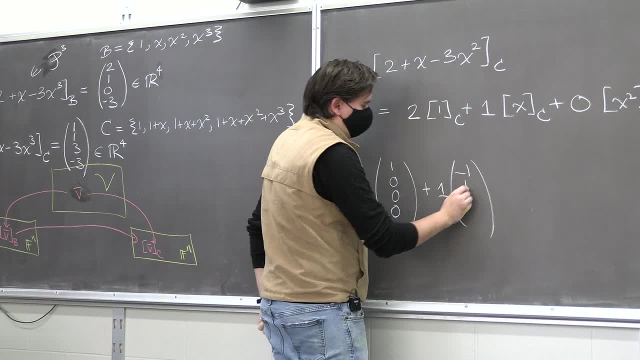 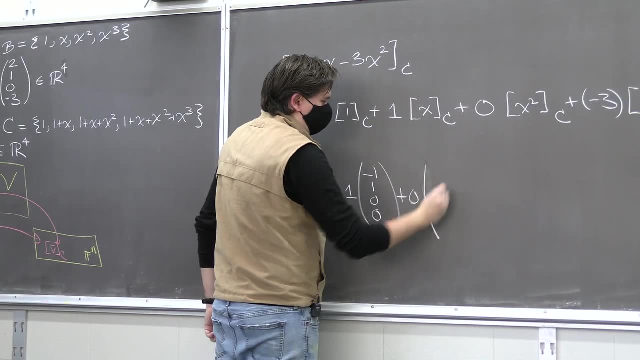 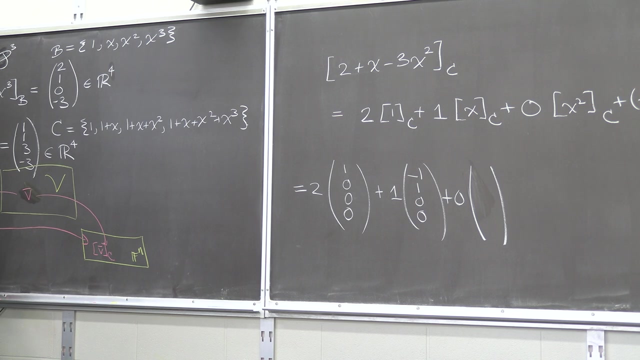 Now you're left with just X. So negative, one of the first one, one of the second, zero of the rest. How do we express X squared with respect to this basis? Yeah, we want a copy of here, this guy to get your X squared. 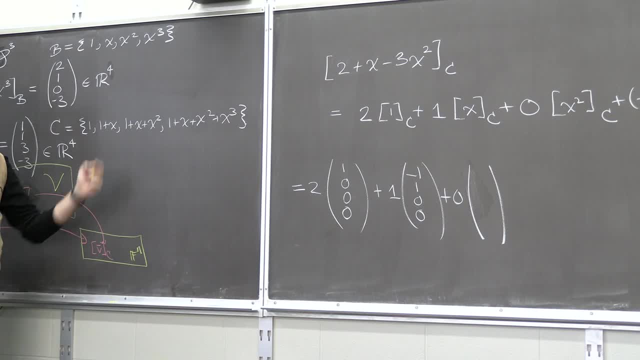 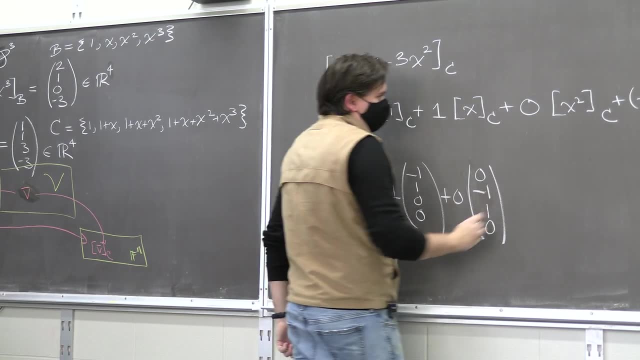 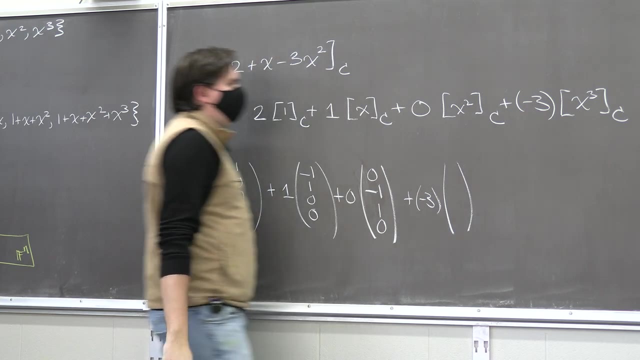 but then you want to get rid of your one plus X. So you need to subtract off the second guy. So we're going to subtract off the second, add the third and zeros for the rest. And finally, how do we get the X cubed? 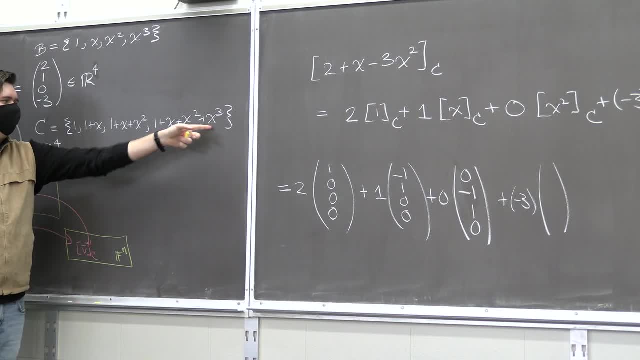 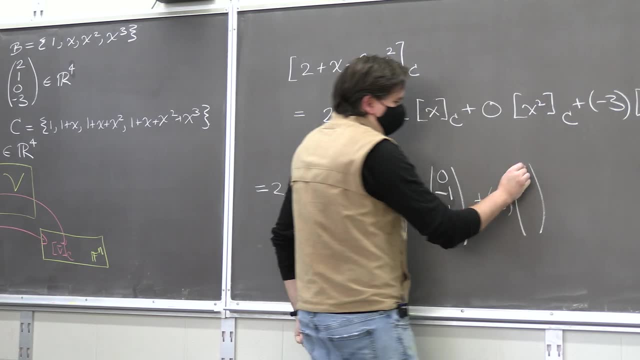 Well, same game as before. We want a copy of the last one. Then we want to get rid of all this other pieces- X squared plus X plus one- which just means we need to subtract off the penultimate piece. So we're going to do zero. 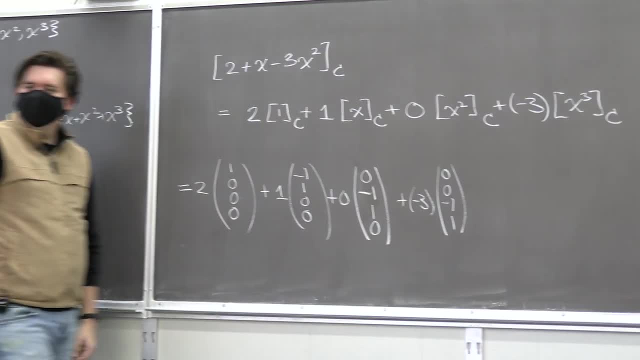 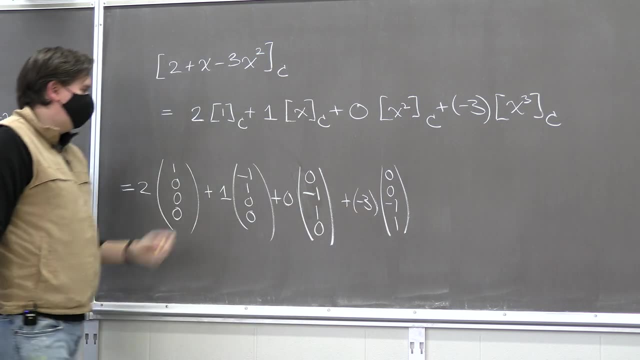 zero minus one one, Yeah, Okay, So it wasn't too bad to convert these guys into the basis. Okay, So we're going to do zero, zero minus one one. Yeah, Okay So. C. But now the claim is: 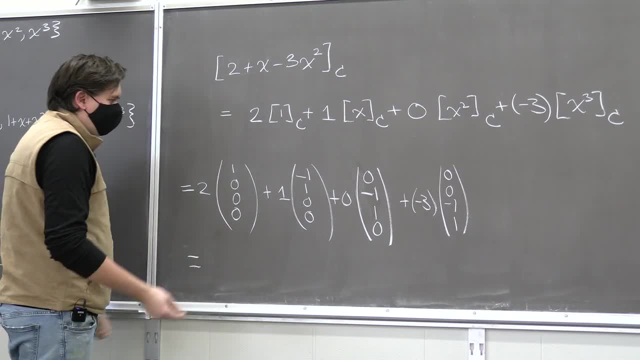 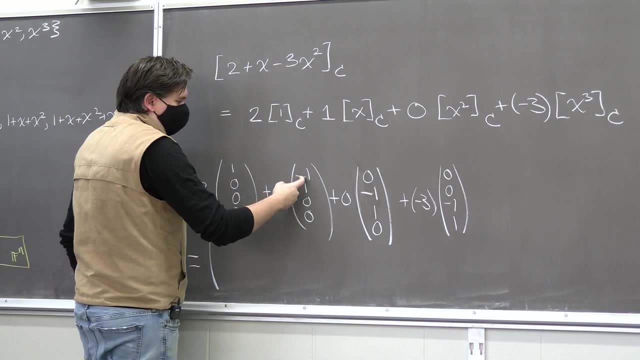 if we just add together the linear combination of those, we should get the right thing. Let's verify this Two times: the first number, two times one is two minus one, So we're at one, And so it's just one zero. 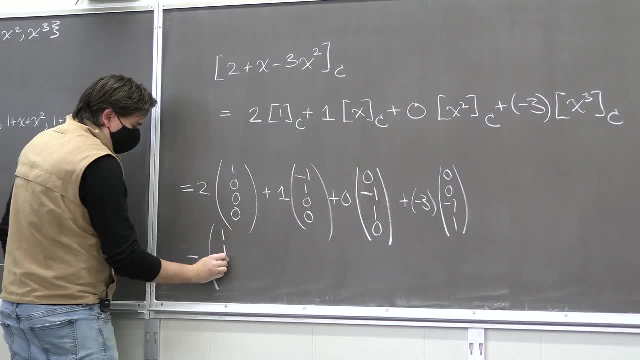 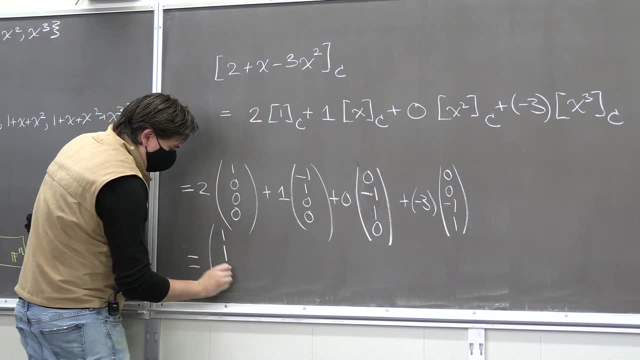 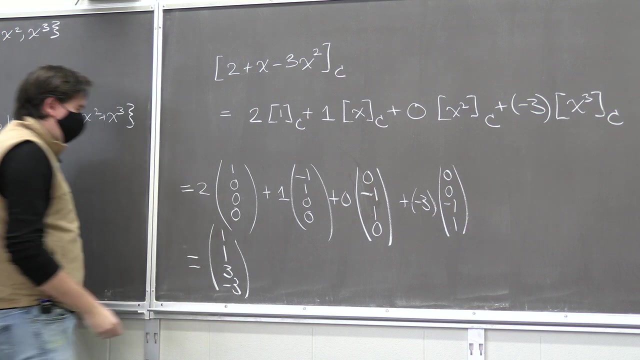 one zero zero. So it's a one zero, zero Doing the third row now. Zero positive three, Zero zero, zero, negative three, Which is sure enough exactly what we had before, Right? So things, things agree. 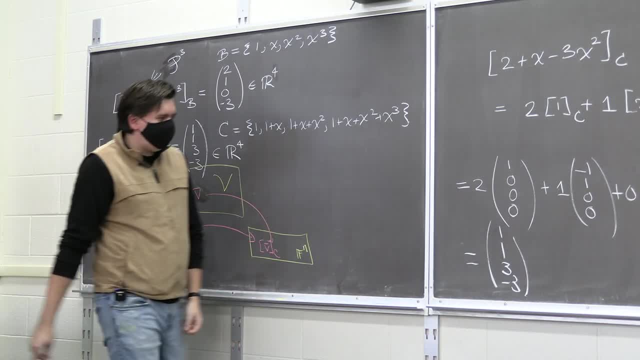 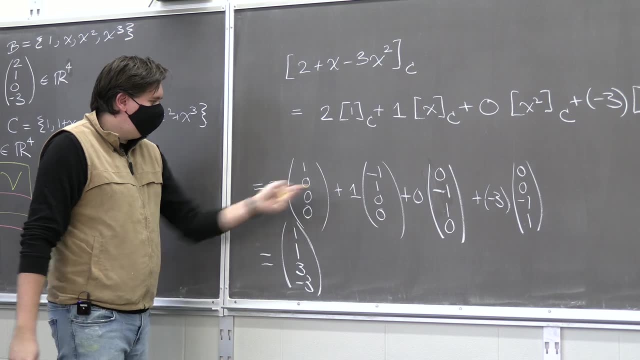 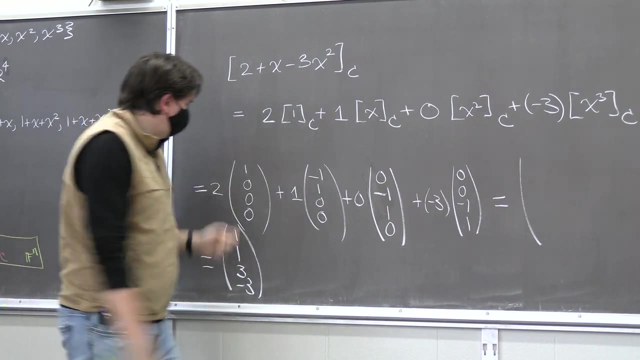 Things are matching up, But what's more significant than actually the calculation is this process to figure it out. I mean, if you look at what this is saying, this is really the same thing as just taking the matrix that you get from combining all these columns. 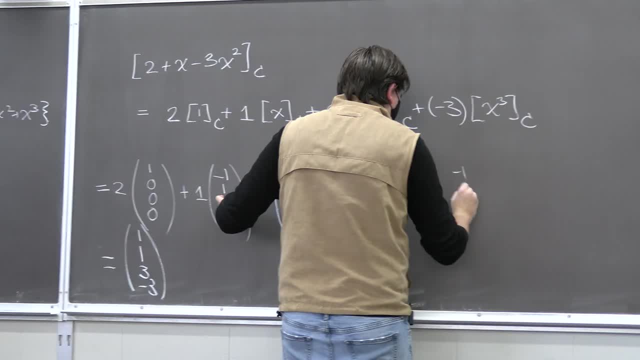 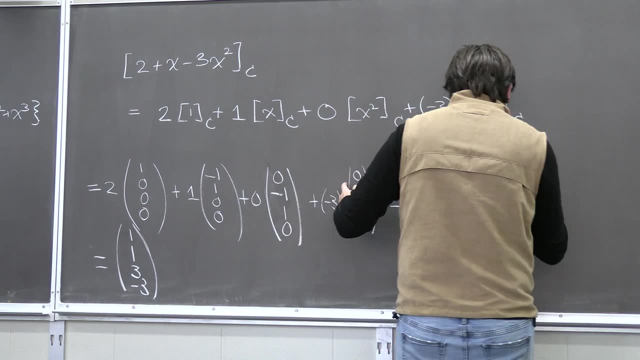 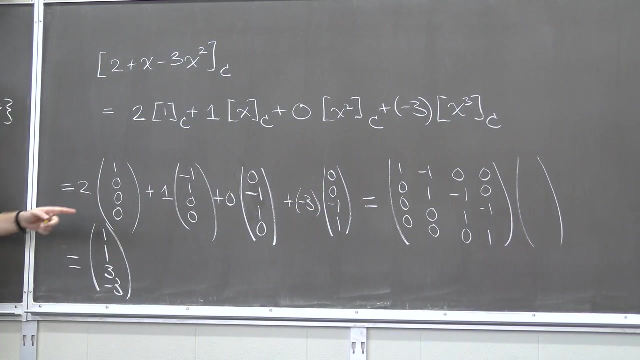 the first column: one, zero, zero. The second column, negative, one, one, zero, zero. The next column: zero, negative, one, one, zero. And the last column: zero, zero, negative, one, one. And multiplying that matrix by the vector, which is these coefficients: 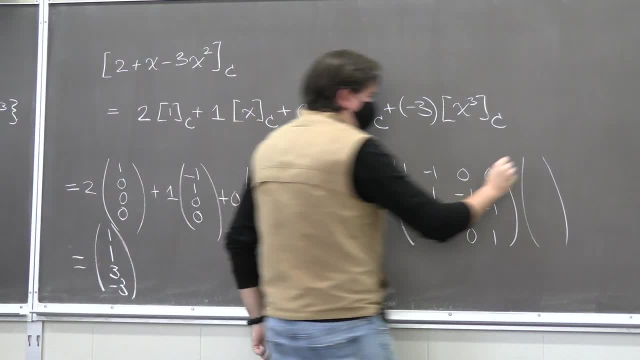 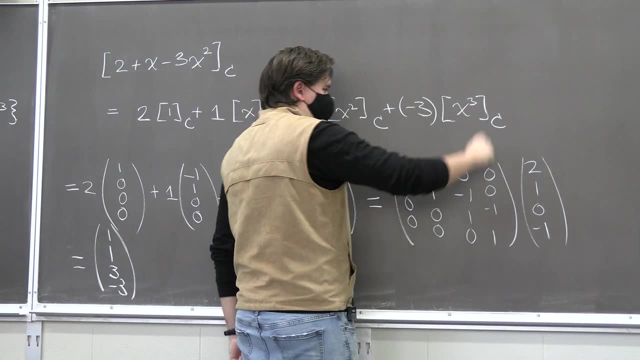 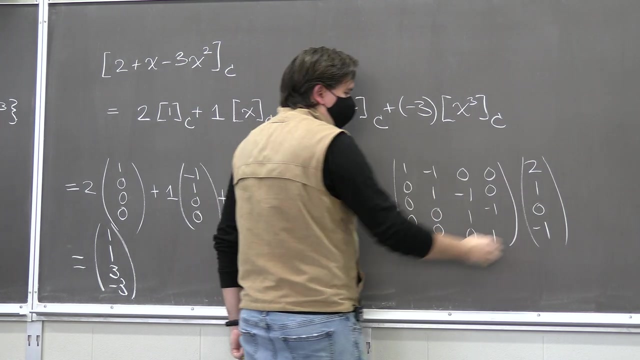 Two, one zero negative three. Because the way matrix multiplication works is when you do your row times column, you end up with two times all the guys in the first column, One times all the guys in the second column, Zero times all the guys in the third column. 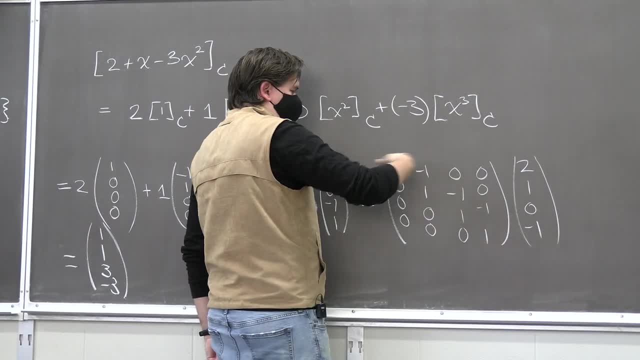 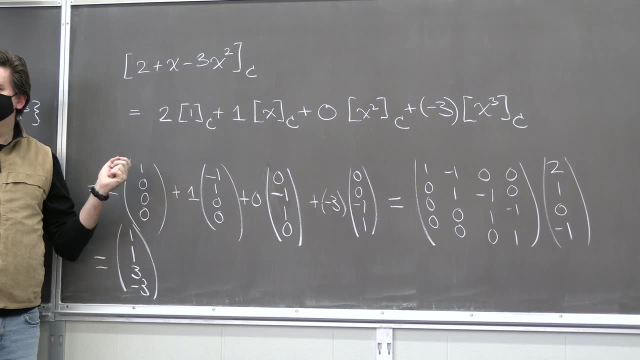 And negative one times all the ones in the last column, And then you sum together those columns, right? So that matrix multiplication is exactly this expression here, Right? so it's a little reminder of how matrix multiplication works. You happy with that? 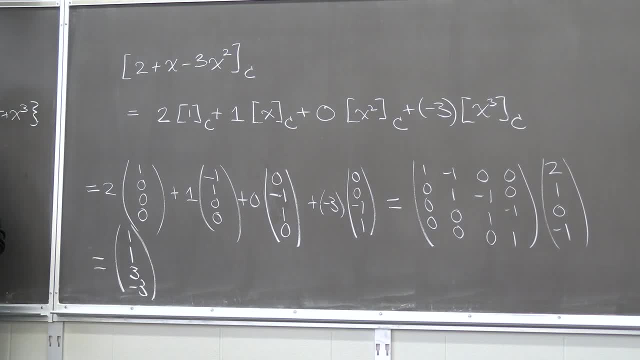 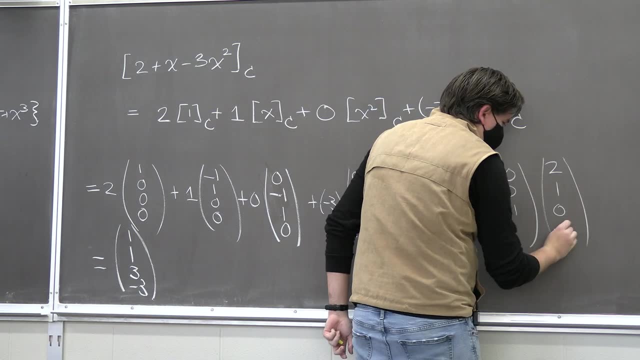 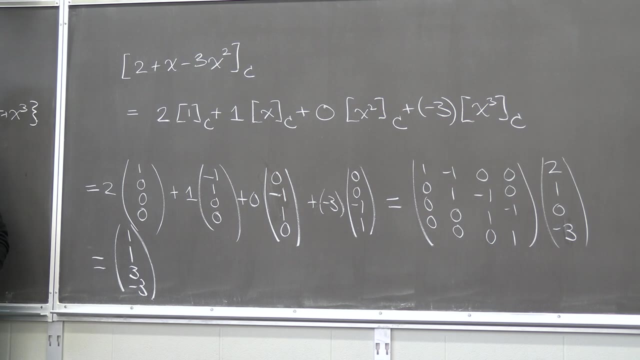 That's good. Yeah, The negative one is supposed to be a negative three. The negative one should be a negative three. That's exactly right. That's exactly right, That negative three. Good catch. But more than just this particular example. 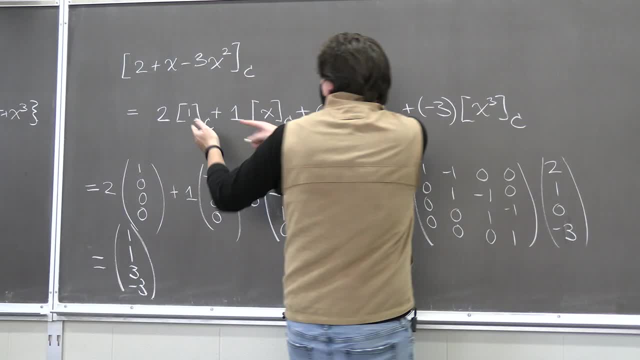 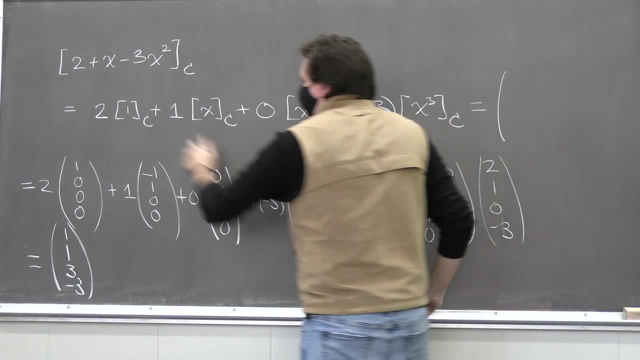 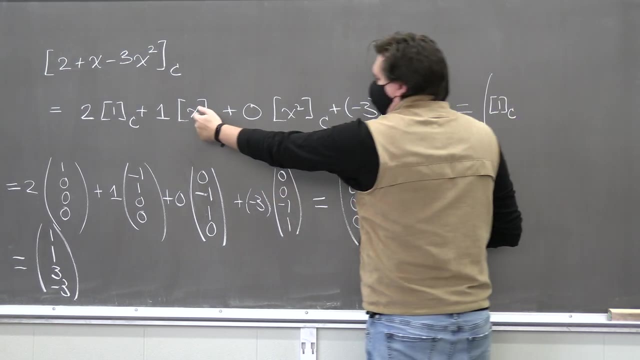 we're now seeing the pattern emerge Like: what is this thing really? This thing really is just the first column. It's where we got when we converted one into the basis c. The second column is where we got when we converted the next element of the basis b, x. 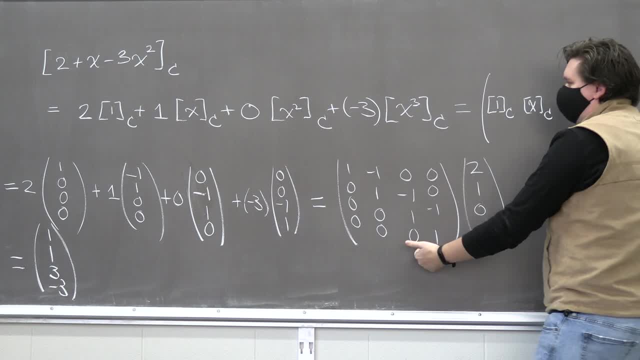 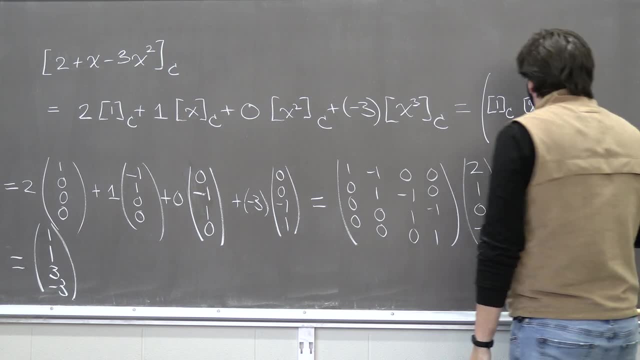 into the basis c. The next column is just what came from the x squared converted to the basis c, So the x squared being converted into the basis c. And the last column is what happened when we converted the x cubed, the last element of our basis b. 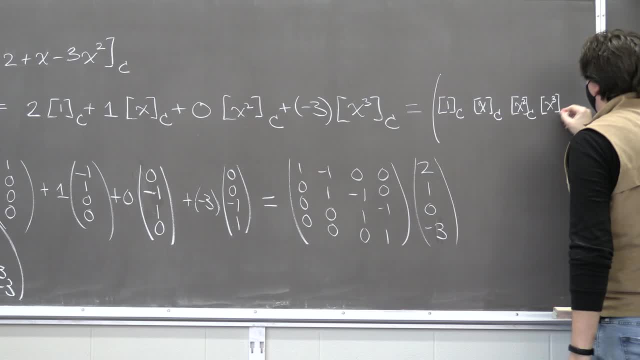 And the last column is what happened when we converted the x cubed, the last element of our basis b. And the last column is what happened when we converted the x cubed, the last element of our basis b, Into the basis c. 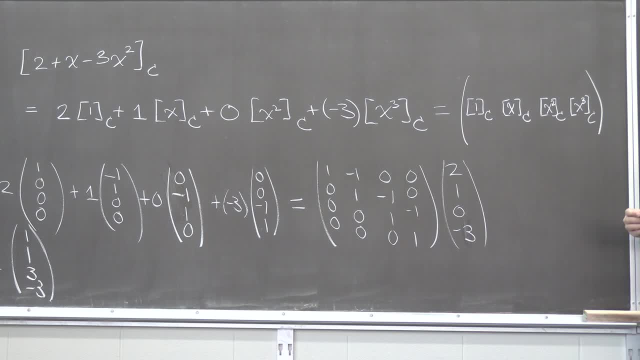 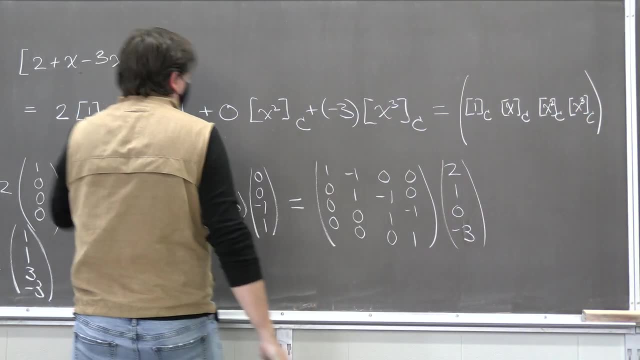 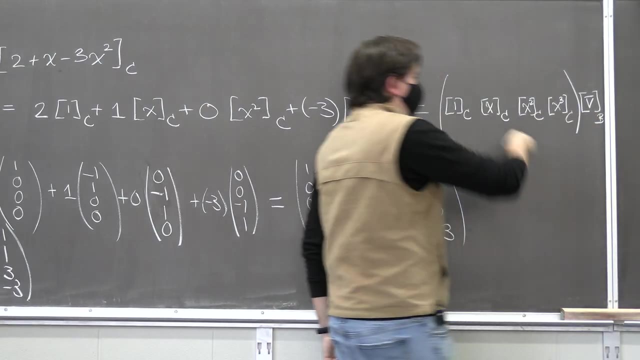 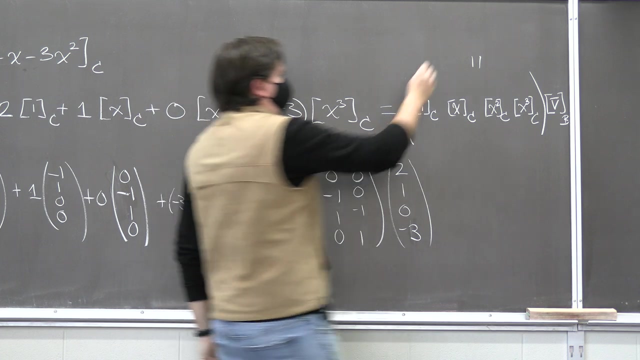 And then what is this vector? It's the coordinate vector. from taking our vector here and converting it into what basis b? And when we did that, we ended up with this guy, which is that same vector v. This is the same vector v. 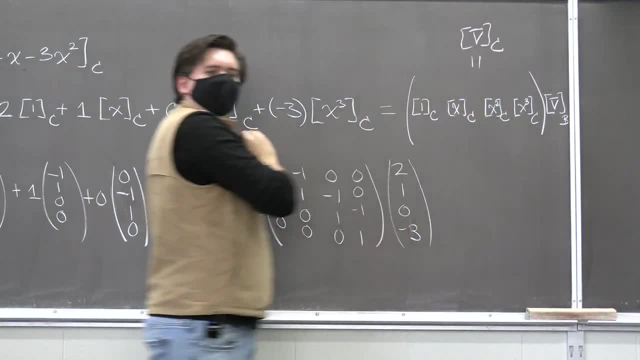 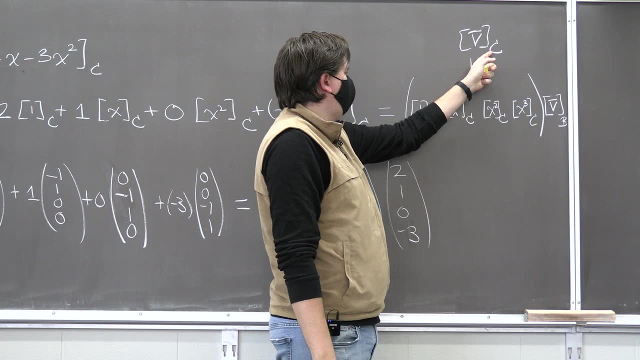 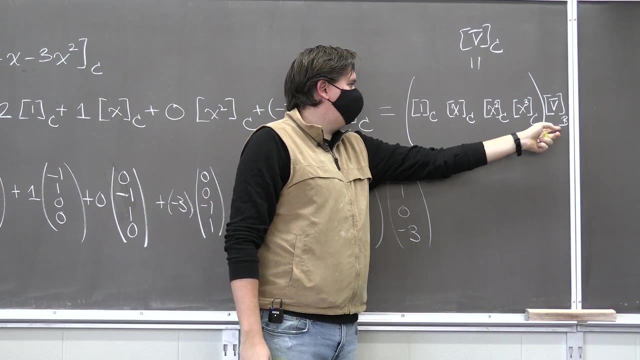 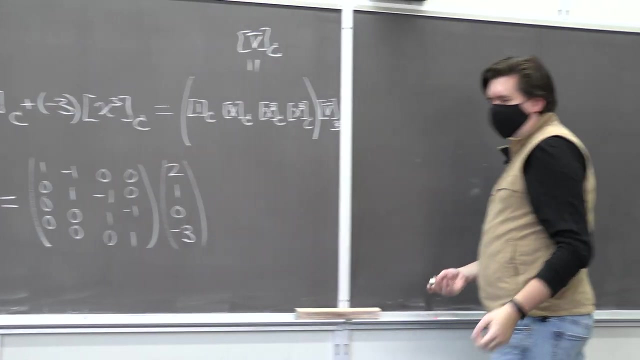 This is the same vector y, now with coefficients in c, right? So how do we convert from coefficients in b to coefficients in c? We multiply by a matrix where each column was just the elements of the basis b converted into c. So let's write this down as a result and show that it works in general. So here's my theorem. 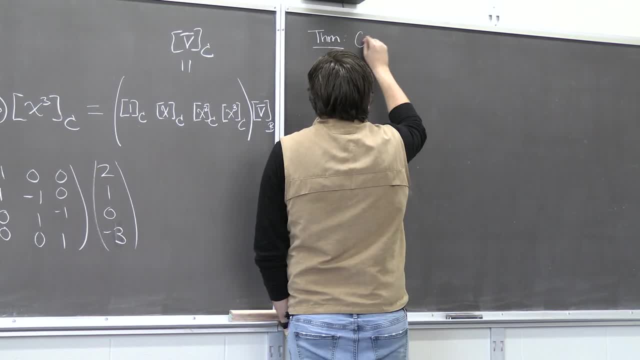 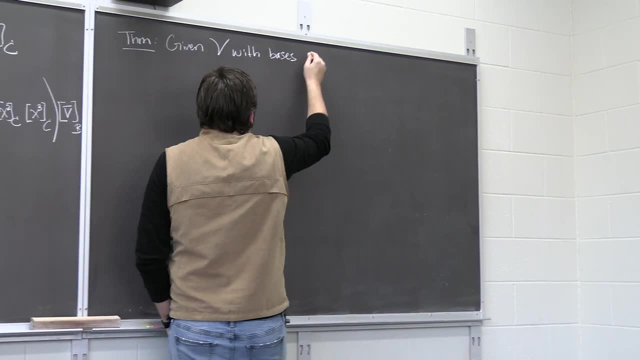 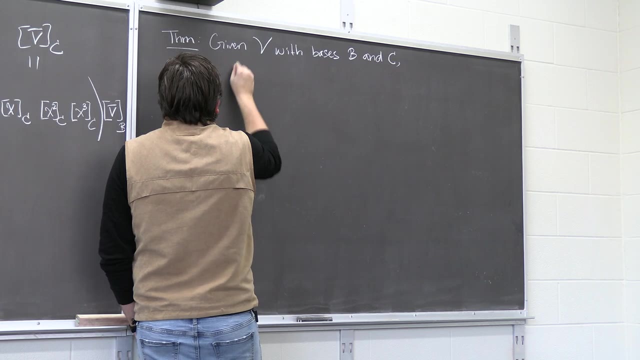 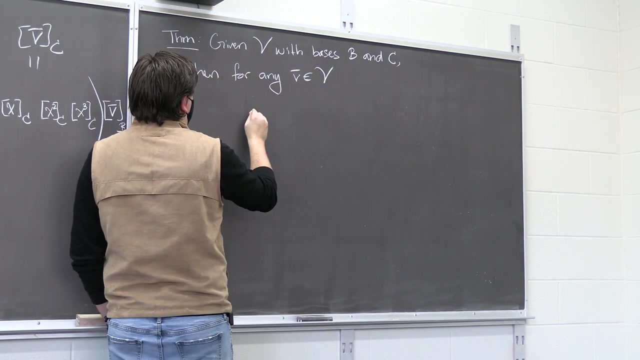 So we should be given some vector space that has multiple bases. So let's say one basis is b and another basis is c, Then the claim is for any vector you pick inside that vector space if you want to convert that vector from having coefficients. 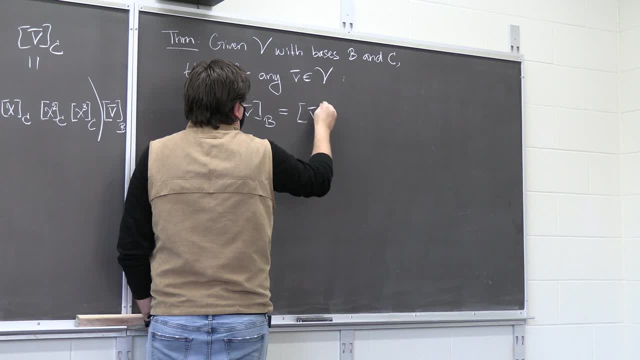 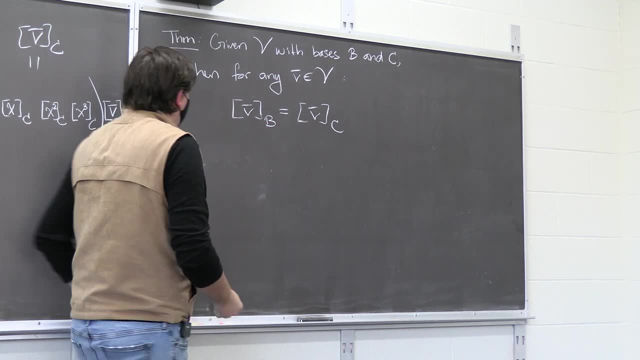 into coefficients in c, then you need to convert that vector from having coefficients in c to b, to having coefficients and c. if you want to find the coefficient vector in terms of c, given the coefficient vector in terms of the basis b, you need to multiply by some matrix that does the. 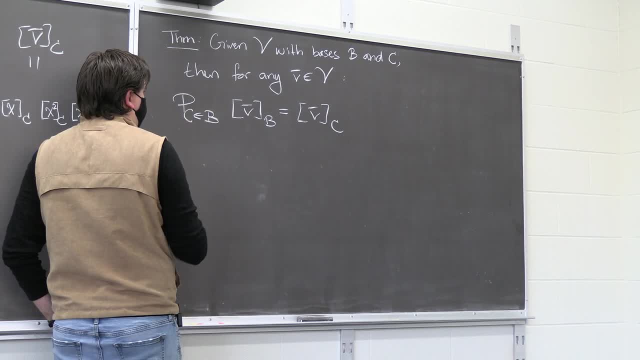 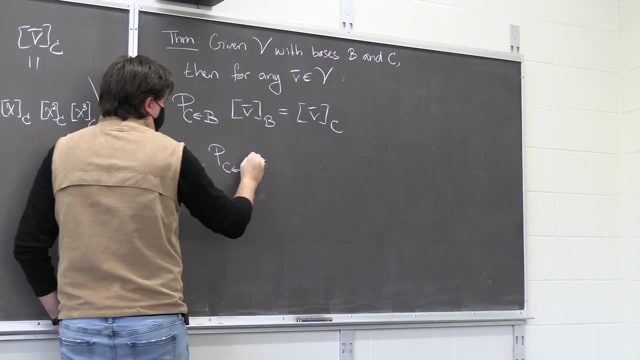 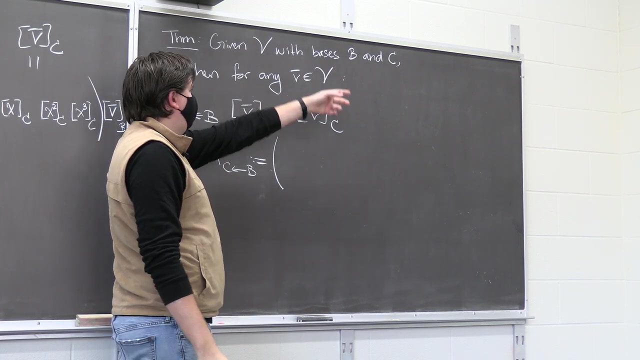 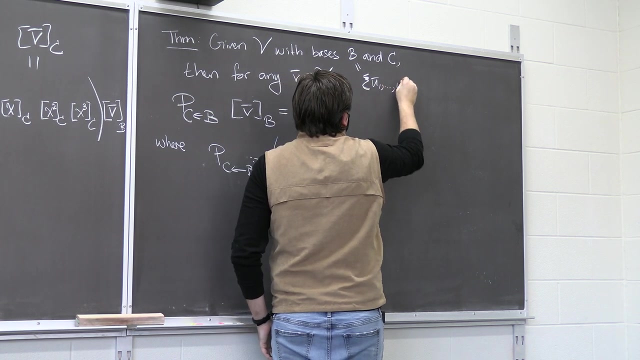 work of converting b into c, where that matrix is just going to come out to equal, is defined to b, the matrix you get from. oh well, i should give these these guys some names. let's say that b is the basis comprising the vectors u1 through un, where n is whatever the dimension of my vector. 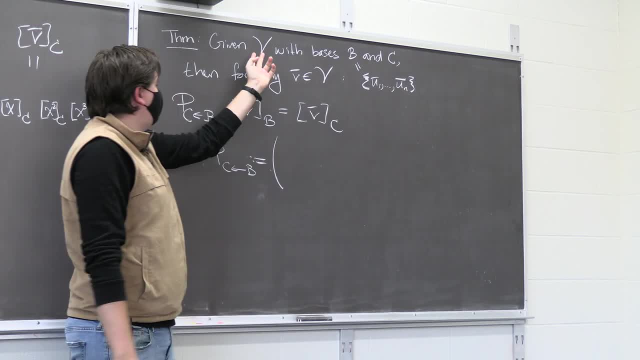 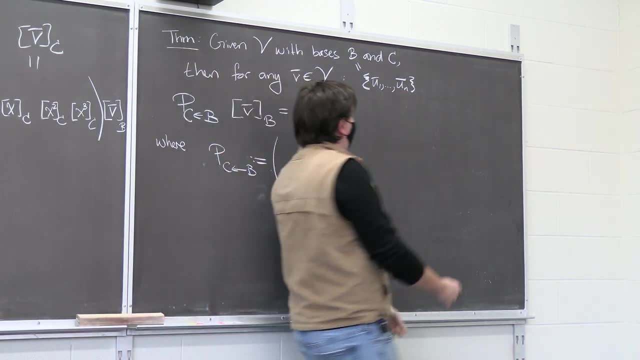 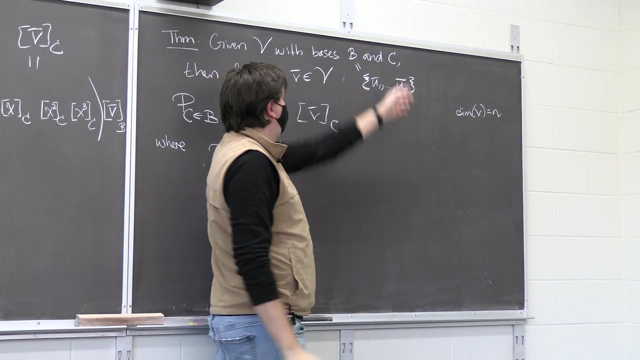 space is. note: this is only going to work if this is finite dimensional. so so i'm assuming this is a finite dimensional vector space. right, this has some dimension. n let me just write that here. i'm assuming the dimension of my vector space is finite, and then c should be some other basis with some vectors. let's call: 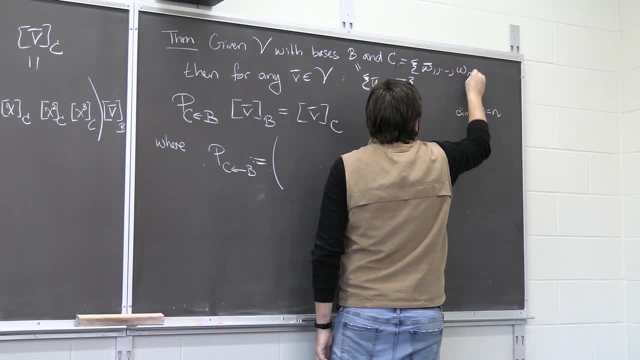 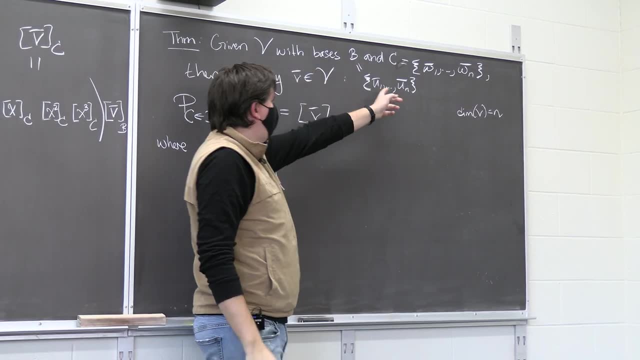 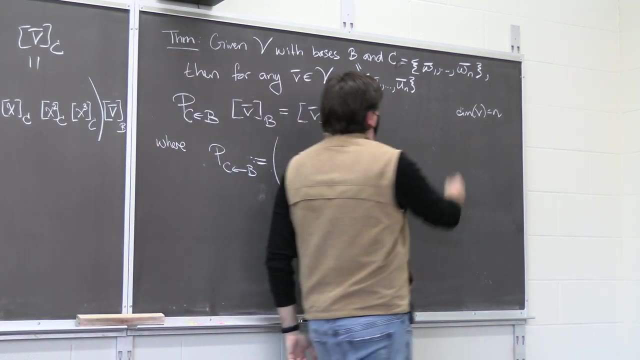 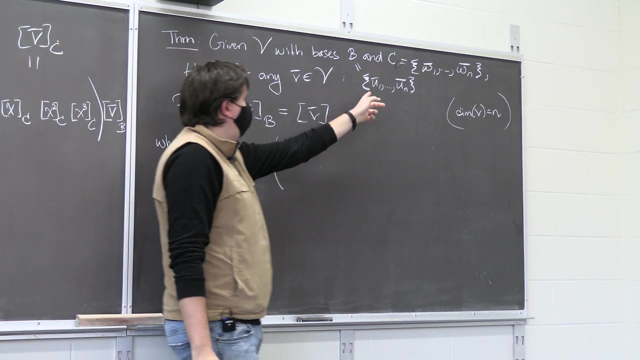 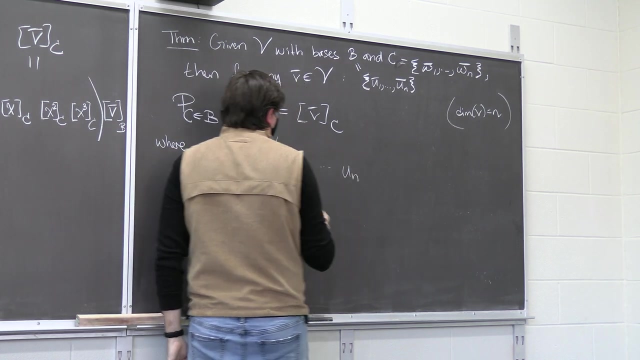 them. maybe w 1 through w n? we showed last time that any two bases will have the same number of elements. that number of elements is your dimension, right? okay? so then how do we convert from D to C? you just take all the vectors in the basis for B- u 1 through u n- and you convert those into C. 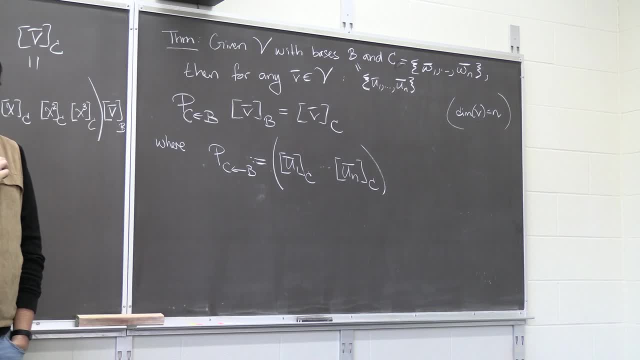 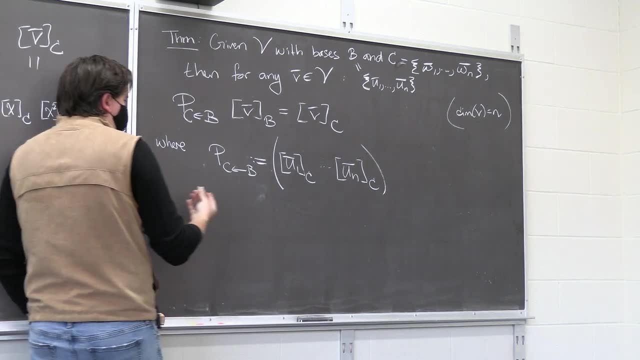 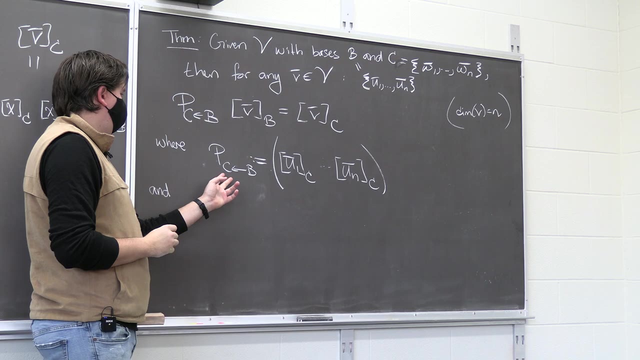 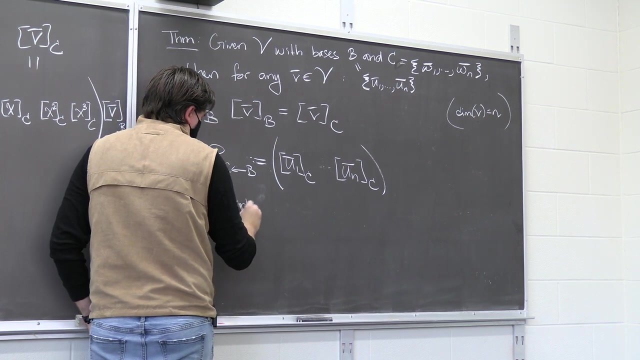 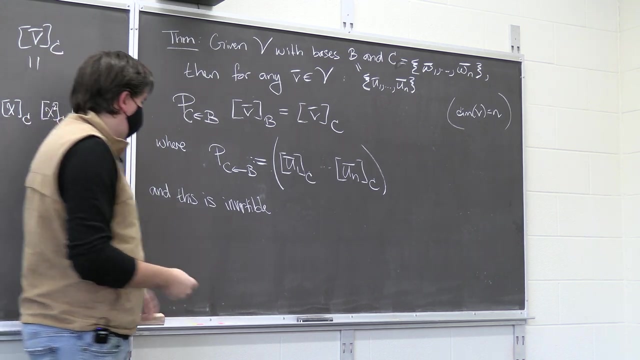 obviously a couple things about this matrix. first of all, this matrix is invertible. so the determinant is going to be non-zero. so the determinant is going to be non-zero and what will the inverse be? what do you think the inverse should be of the matrix that turns? 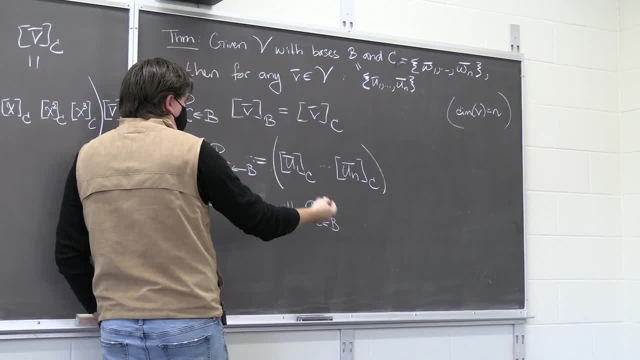 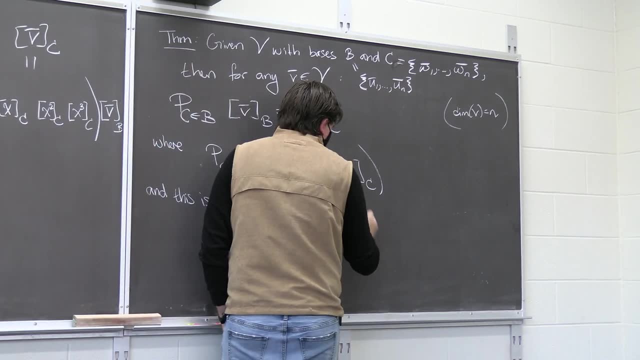 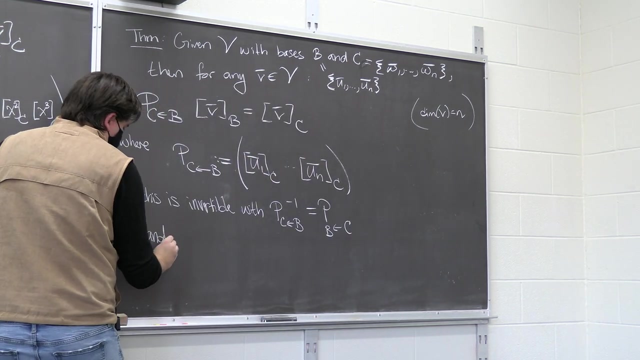 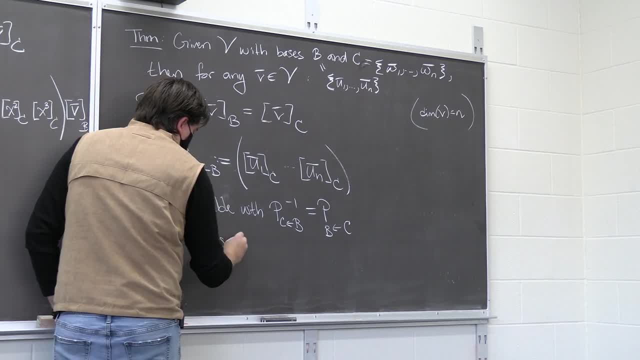 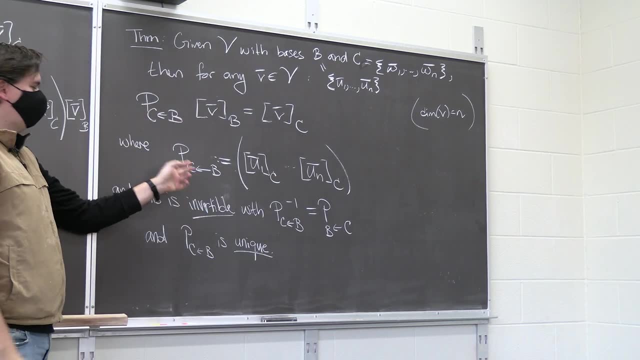 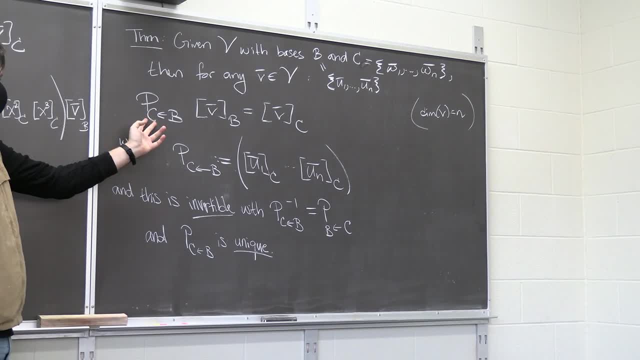 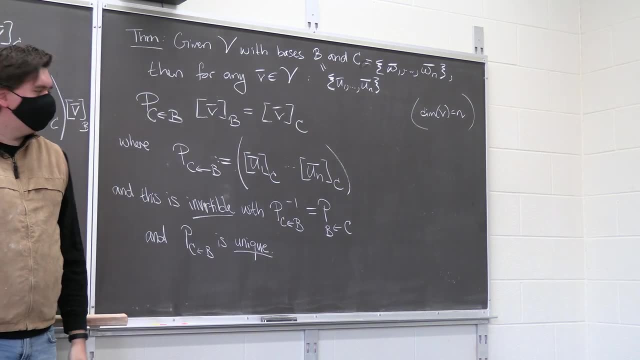 there's no other matrix you can put here that will convert it for all vectors in vector space. so we have three things to prove, first of all, that this matrix actually does where you want it to. second, it's invertible. third, it's unique, right okay? third, it's unique, right okay? 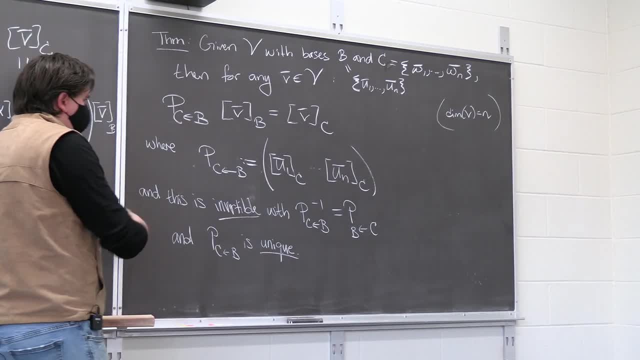 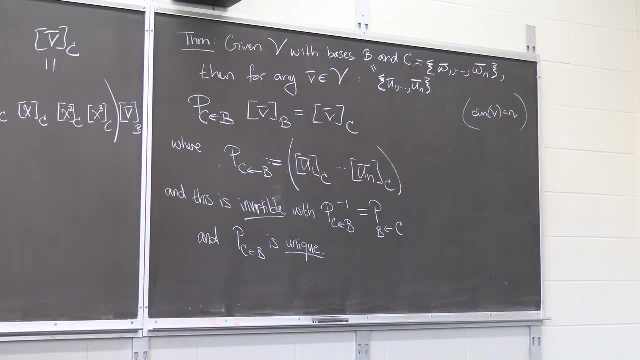 Okay, first one's going to be the most interesting, it's pretty straightforward: the last two. they're going to follow very quickly, So let's prove this. I want to leave this picture here for now, so I'm going to clear this board. 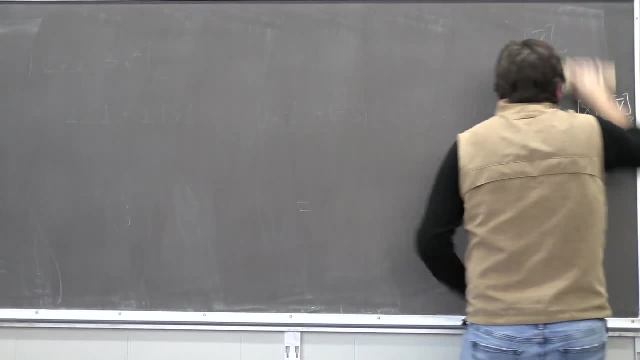 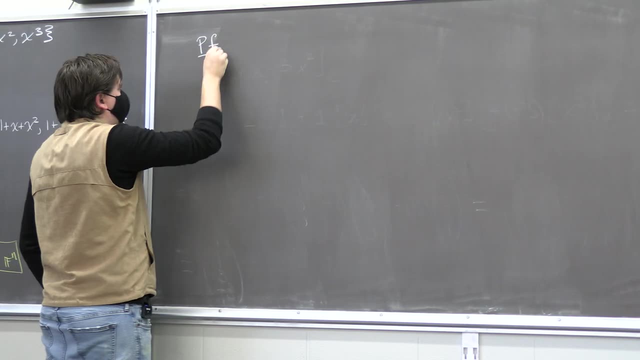 We're essentially going to do what we just did, but instead of working with a specific example, we're just going to work in general. So here's my proof. I mean, I just need to show that this really is equal to this guy. 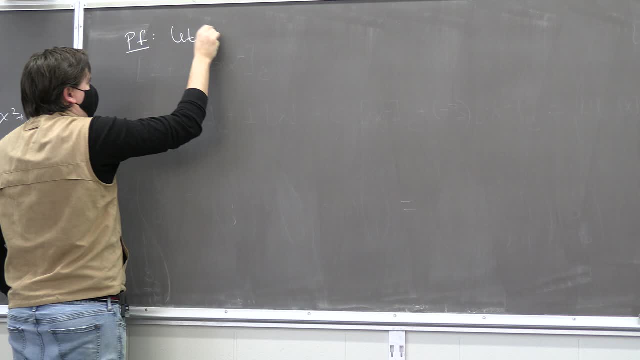 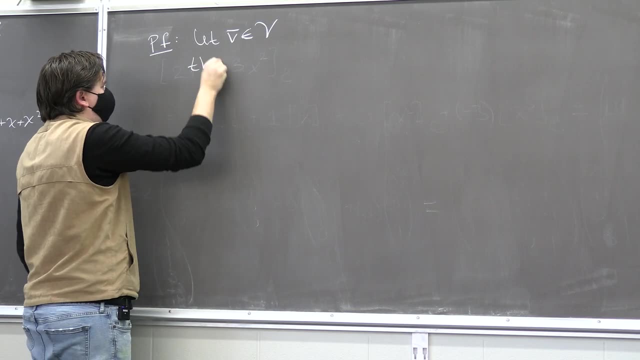 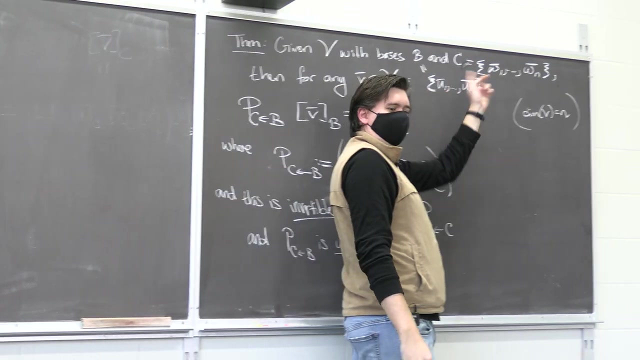 So let's just show that. Just let v be something in your vector space, Then we can write v as a linear combination of either one of our bases, either one. For now it's going to be convenient to write v as some linear combination of either one. 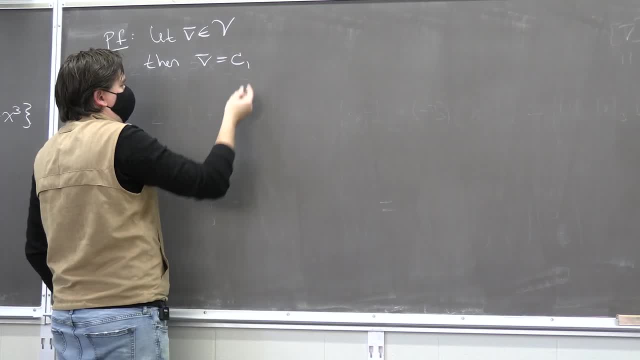 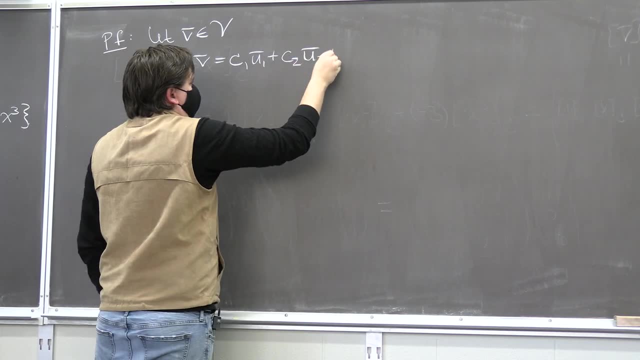 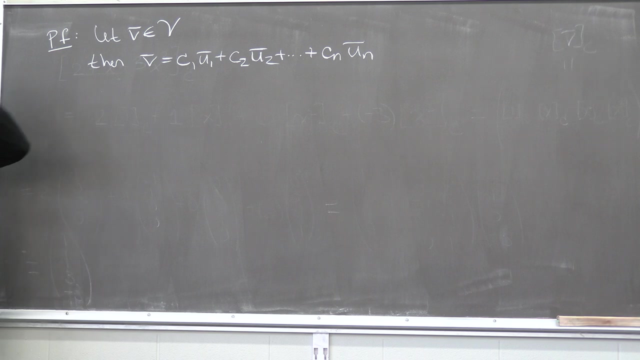 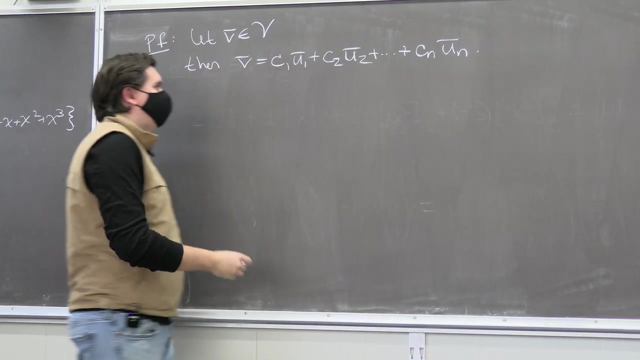 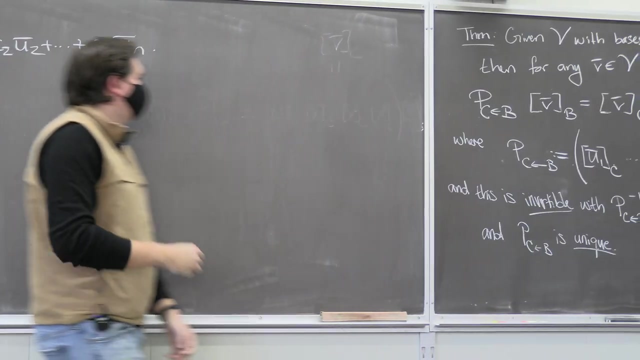 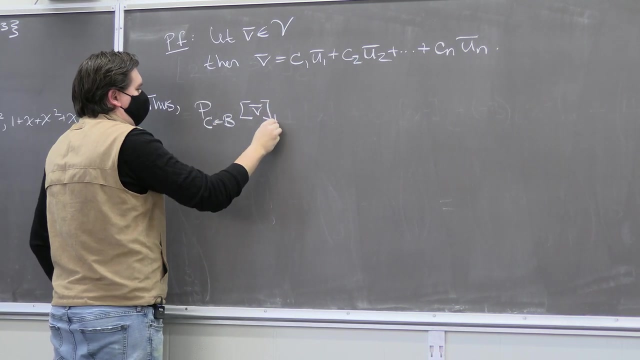 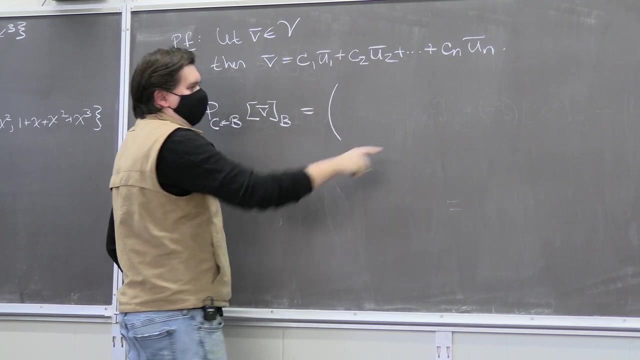 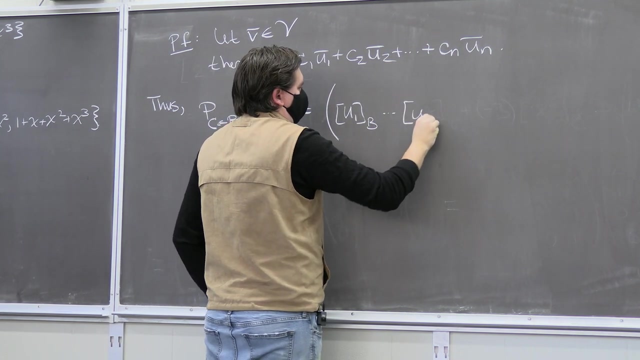 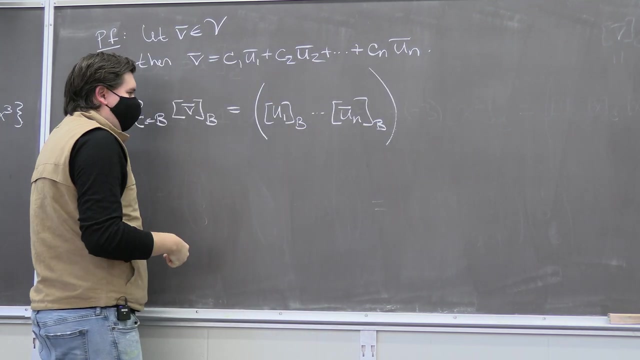 of our bases. So let's just show that this calculation works. What is my matrix times v converted into the basis b? Well, that's going to be the same as my matrix given by u1 through un coefficient vectors, in terms of the basis b as its columns times u1 through un. 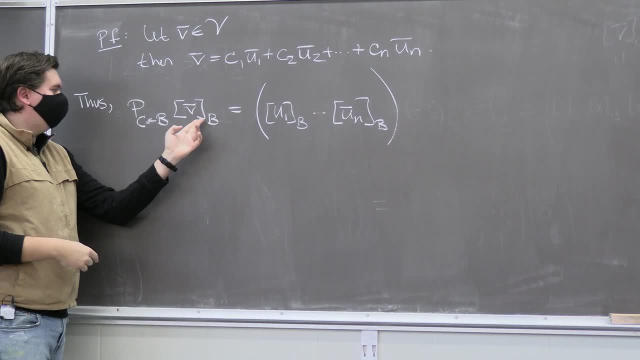 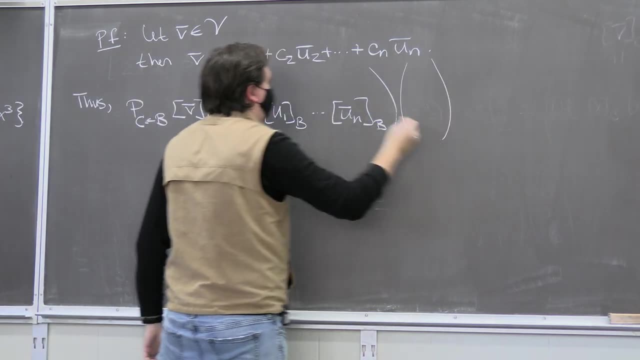 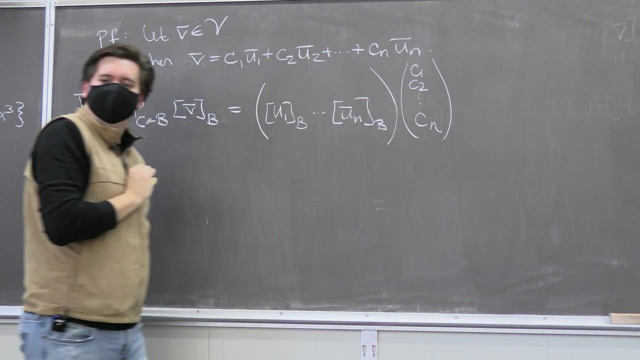 So that's going to be v times this vector, which is the coefficient vector for v in terms of the basis b. And what is that coefficient vector? Well, it's just these coefficients: c1, c2, down through cn. These are columns. 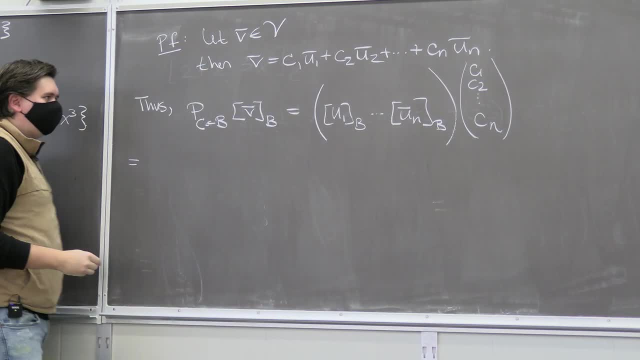 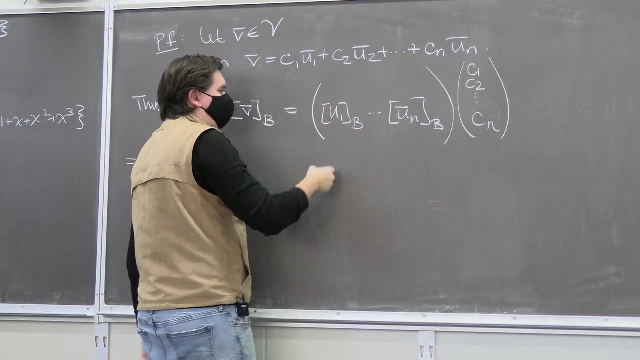 These are columns, So how does matrix multiplication work? Row times column or equivalently. what ends up happening? Is it c1 times all of your first things plus c2 times all your second values, all the way down to the end? 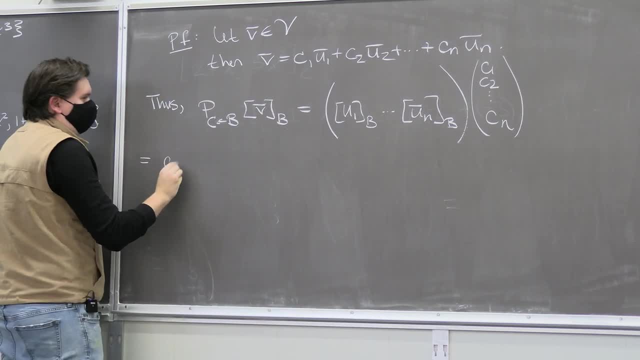 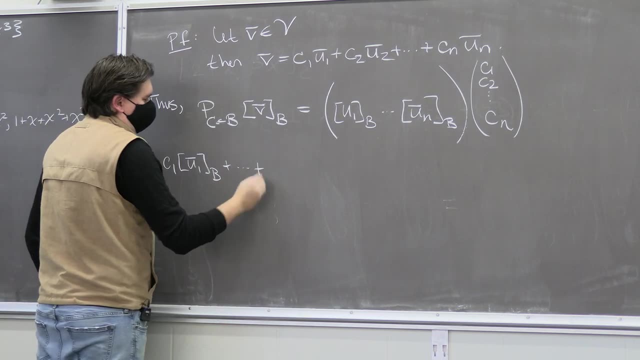 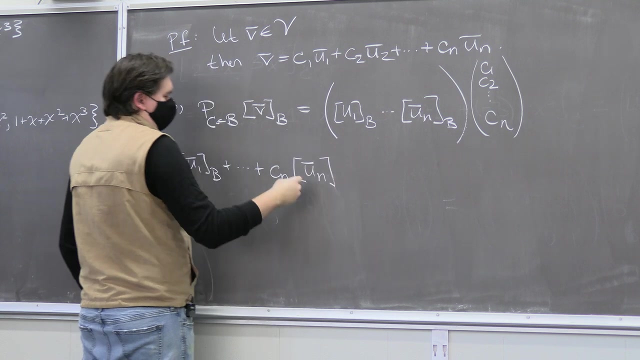 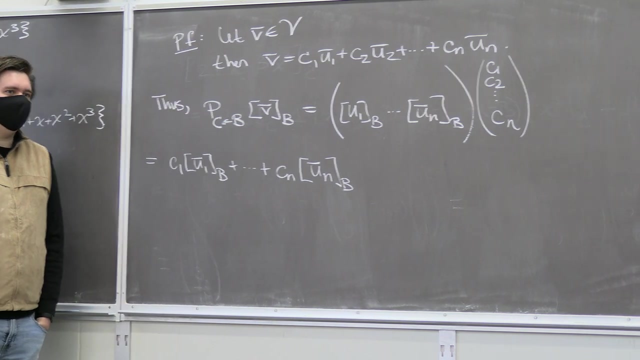 And so you end up with c1 copies of u1's coefficient vector in terms of the basis b, up through cn copies of the basis vector, un's coefficient vector, whose coefficients are in terms of the basis b. Well, shouldn't it be in terms of the basis b? 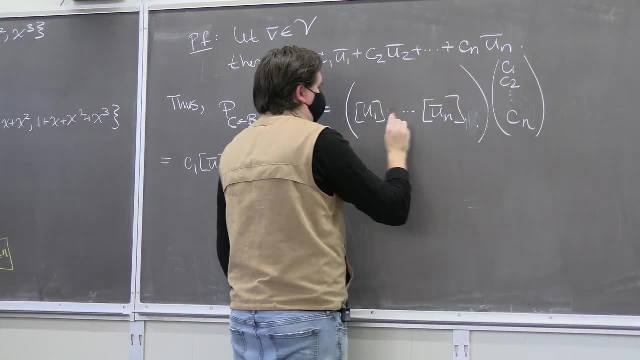 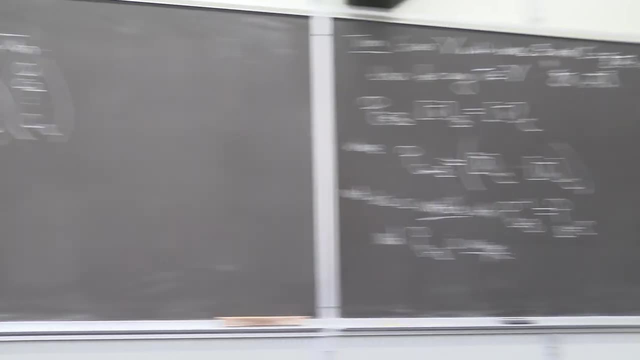 Oh, my goodness, thank you, This coefficient vector. these should be in terms of c. That's our definition, right here. right, In terms of c, Yeah, Which you're about to see, right Like, that's what we need. 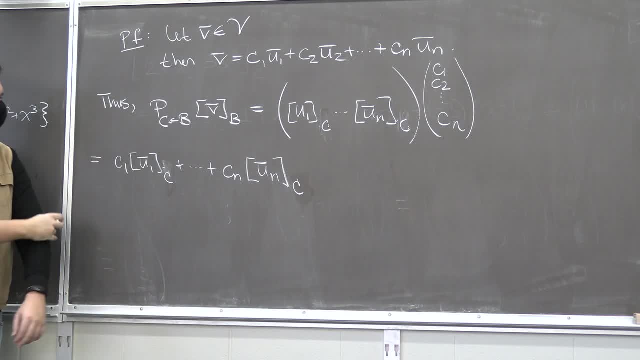 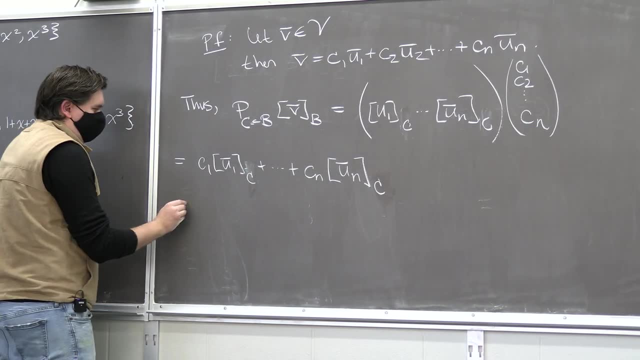 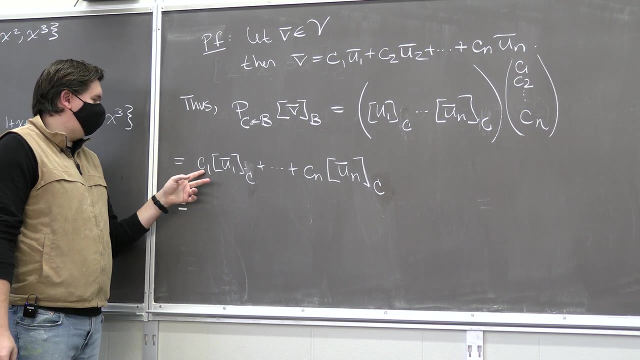 These should be c. Thank you, thank you, thank you, Good catch. So what is this? Well, I don't know. As we said before, it's like: what is the coefficient vector scaled by c1?? Well, that's just the coefficient vector of u1 scaled by c1, right? 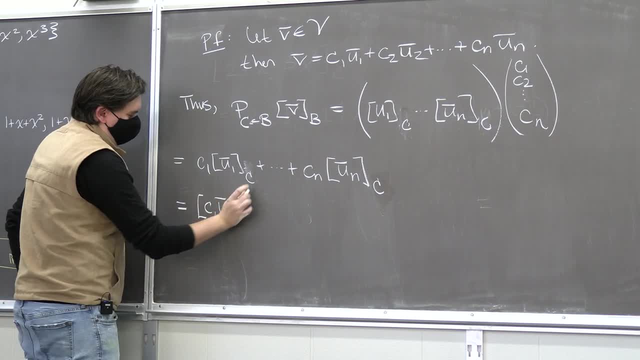 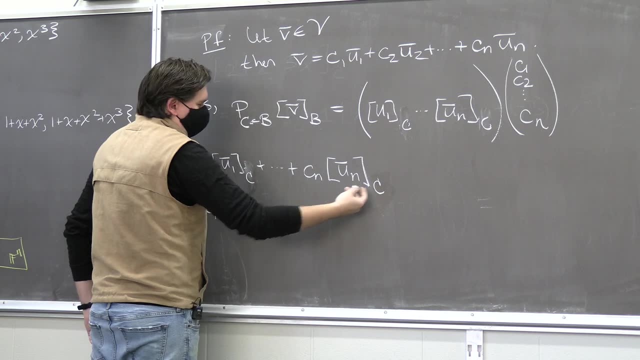 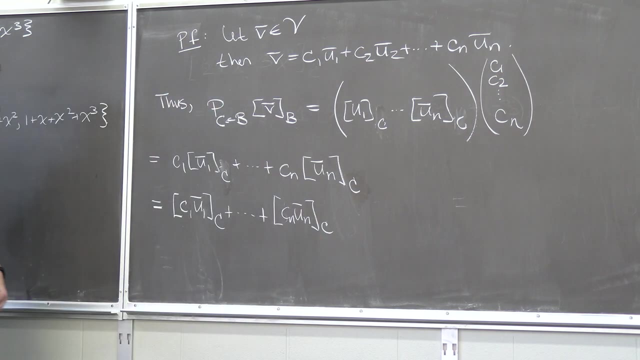 That's just the coefficient vector of doing c1 times u1, all the way through. So this is just going to be cn copies of this coefficient vector is the coefficient vector of cn copies of un And then the coefficient, the sum of the coefficient vectors of two vectors is equal. 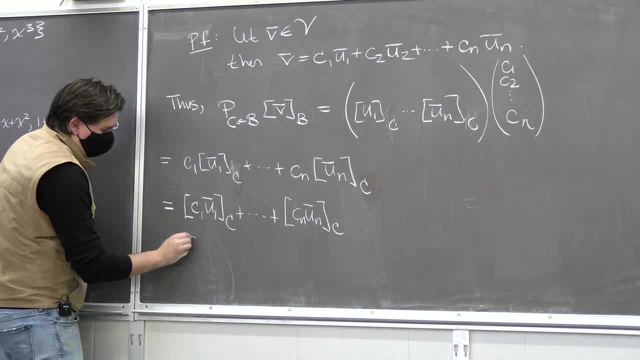 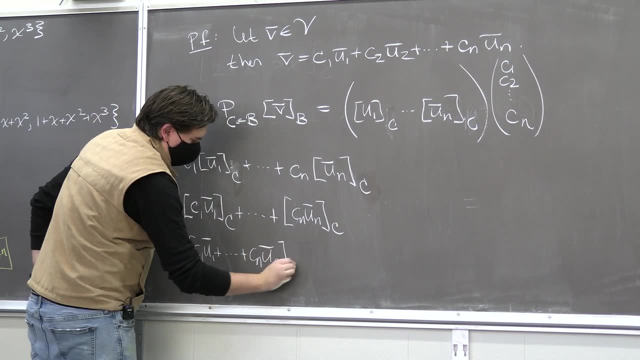 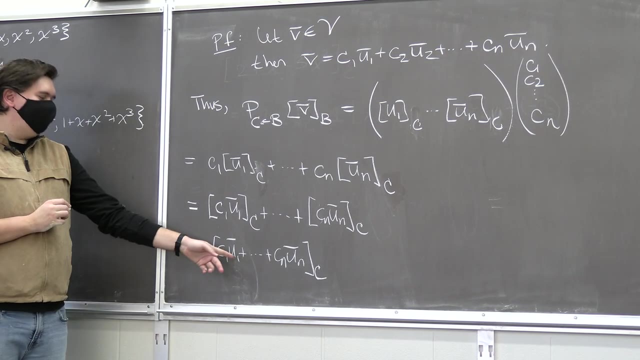 to the coefficient vector of the sum, That is, this just comes out to be c1 u1 through cn un. Happy, Well, I mean, what is that? c1 u1 through cn un is just b, So that's just v. 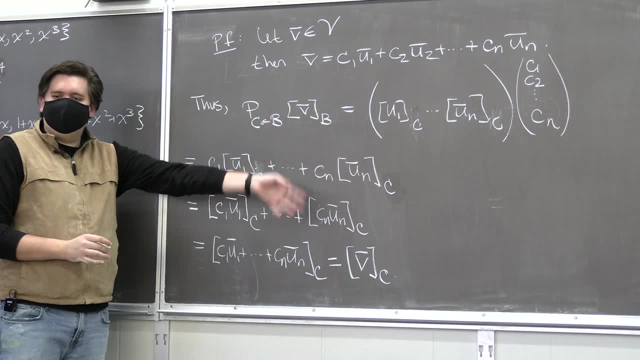 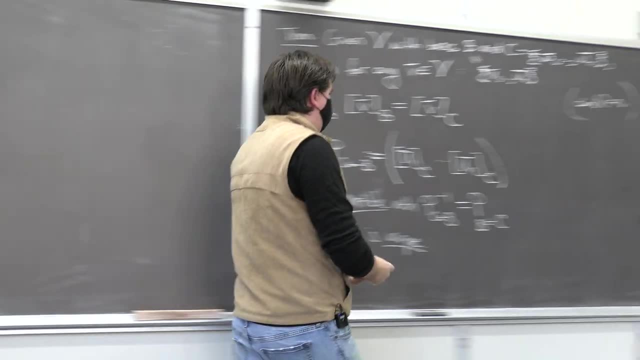 In terms of c. So now we've checked that, yeah, this does what it's supposed to do. We built it to do it, but now we've verified it works in general. So we've verified this first part, that this matrix does the trick. 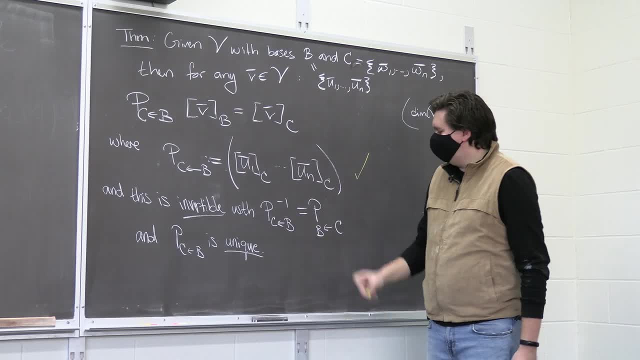 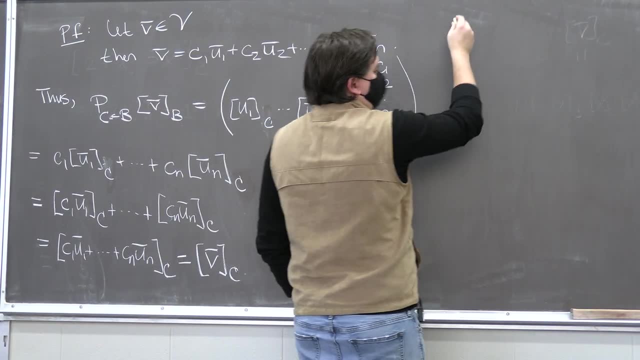 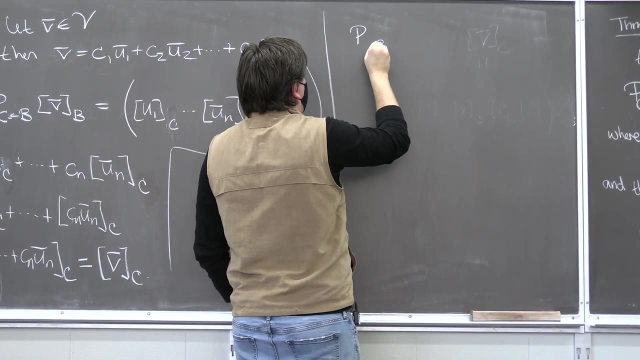 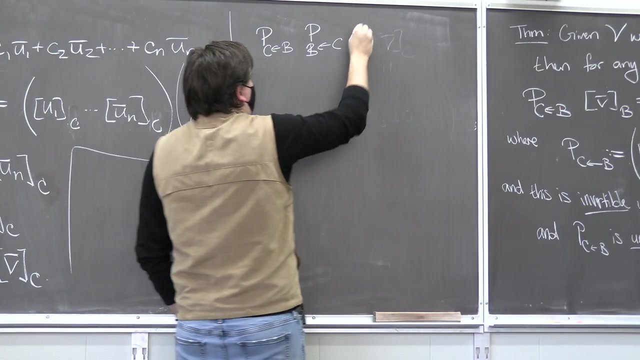 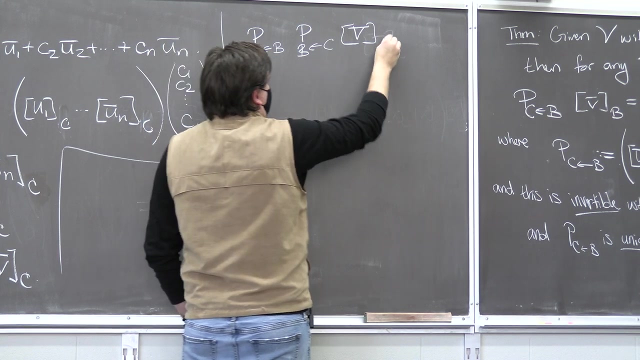 Okay, Let's try and prove the second part, that the matrix is invertible. To do that, I'll just notice what is this: P b to c times p c to b times some vector whose coefficient? this is the coefficient vector with coefficients in c. 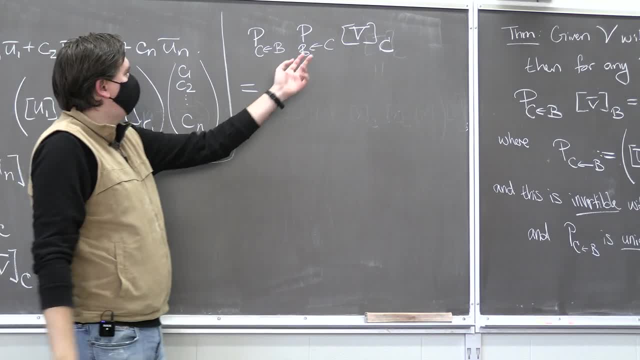 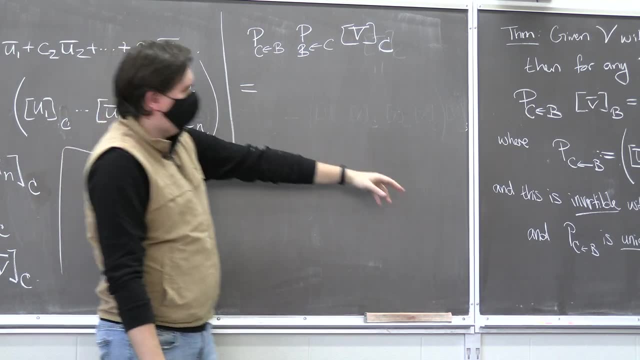 Let's evaluate what this comes out to be. Well, we're going to do first the multiply by the matrix on the left And by our matrix. we're going to multiply by the matrix on the left theorem: okay, so I'm going to prove this theorem going this way. but you can just rewrite, you can. 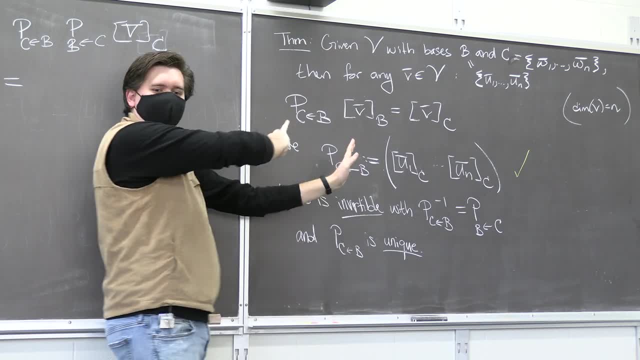 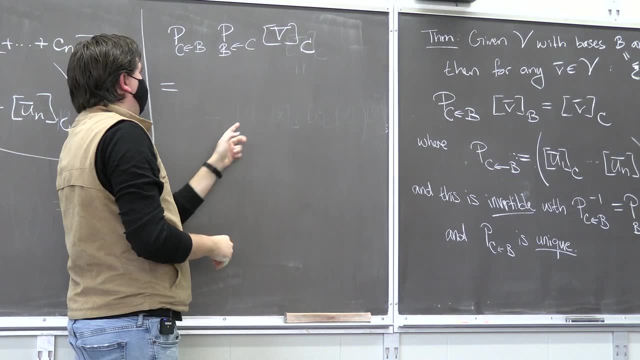 rename c and b. you have the exact same theorem for c to b, right, You have the exact same theorem. So now that we've proven the first part, we know that this first guy is just changing us from c to b. or if this was a b, it would change from b to c. So this guy, this first multiplication step, 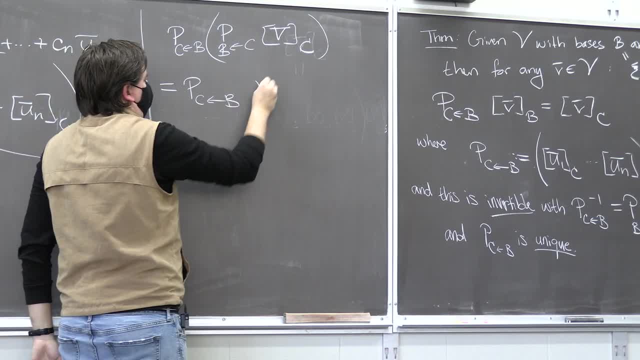 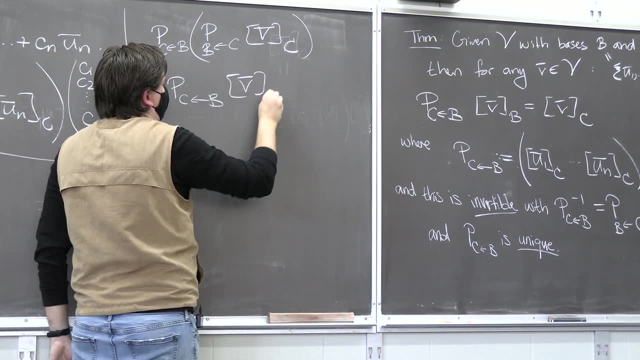 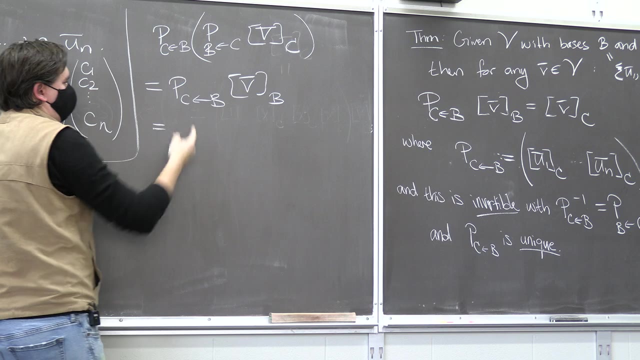 is just going to give us a vector coefficient, the coefficient vector of v in terms of b. right, That's what it does. it changes it from c to b, And then this guy is just going to change you back, and so he's going to end up with this guy. 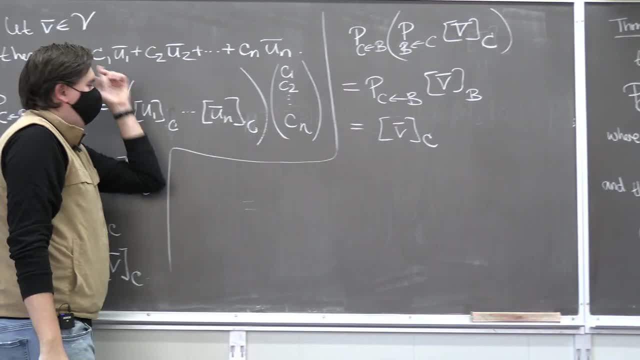 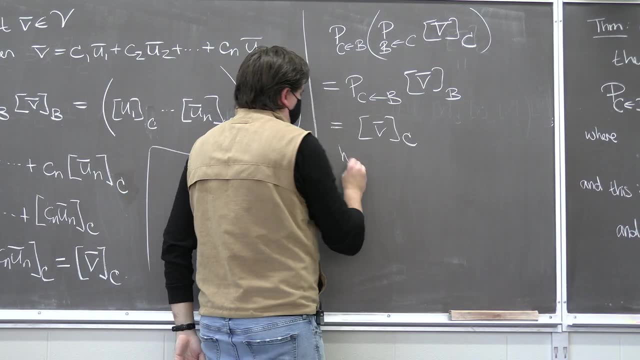 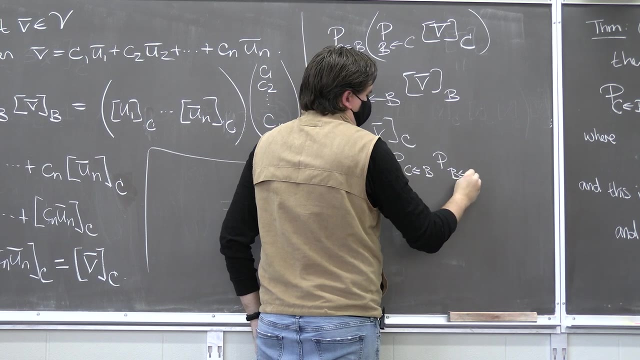 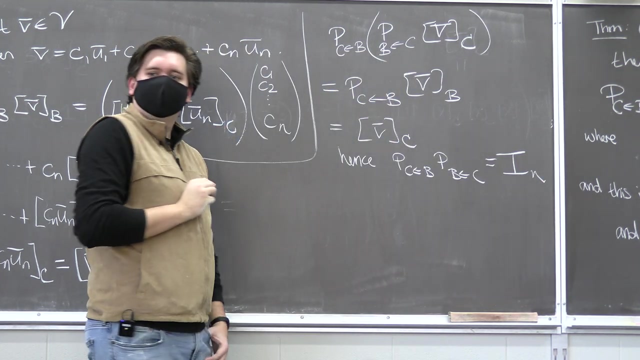 And that's for all of this, All of these in your vector space. Hence it's for all coefficient vectors. Hence your multiplication of these two matrices must just be the identity matrix, the n by n identity matrix. But that means one is the inverse of the other. 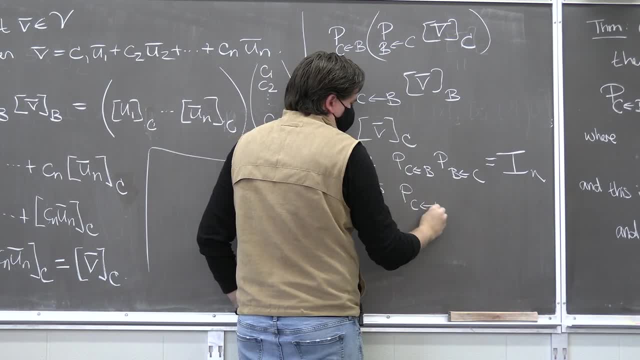 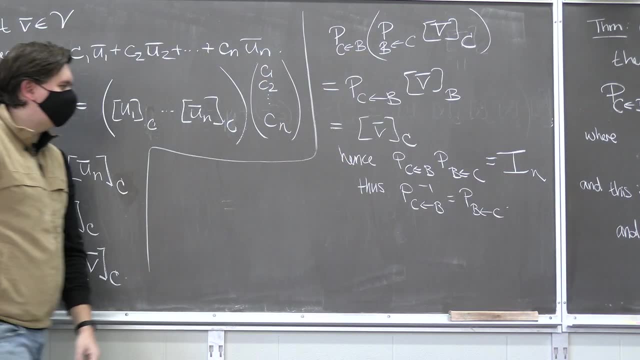 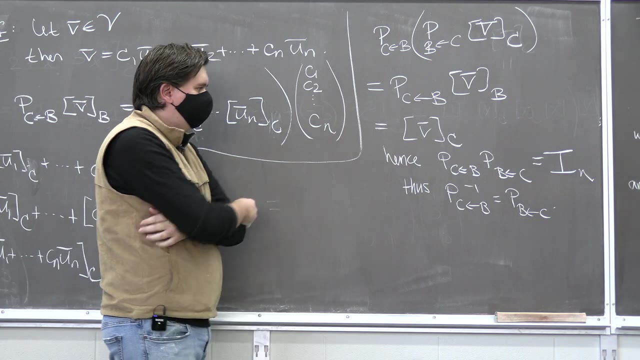 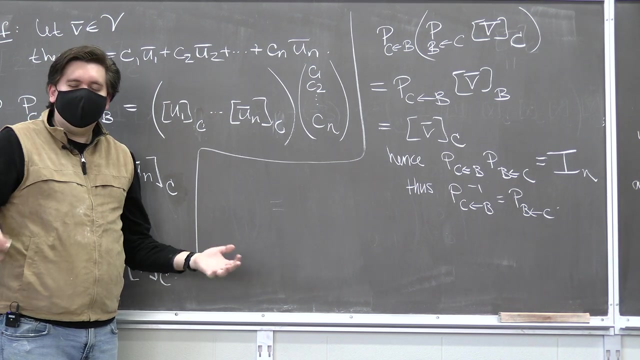 Thus the inverse of one is just the other. So this pretty much comes for free. Like this is rather immediate. Once you know what these matrices do, it's pretty clear that they're inverses of each other. The last point you might worry about a little bit more is like how can we possibly? 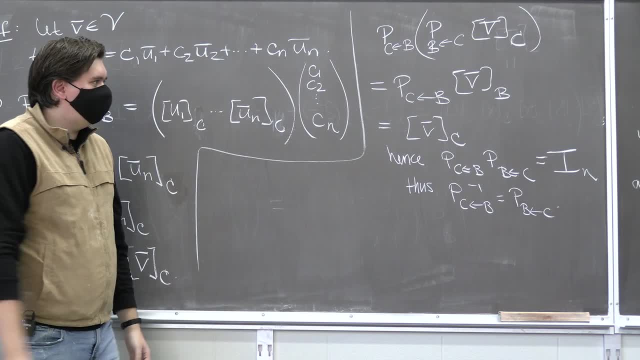 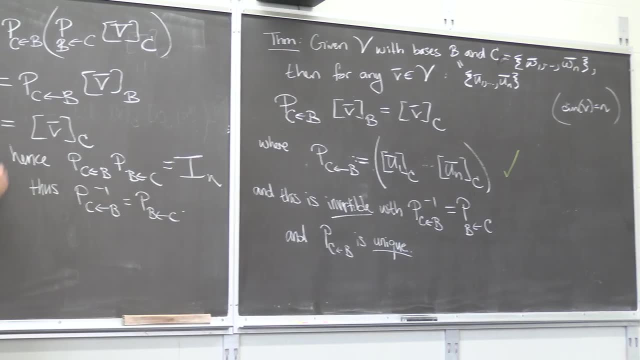 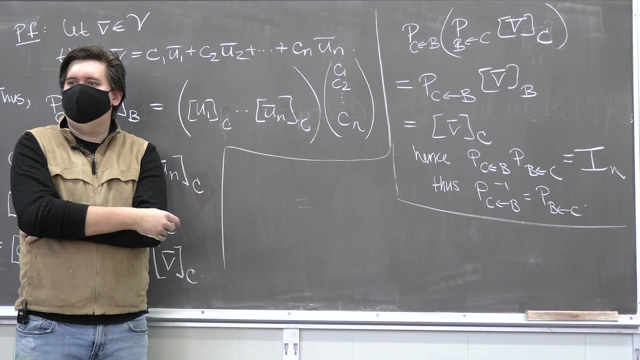 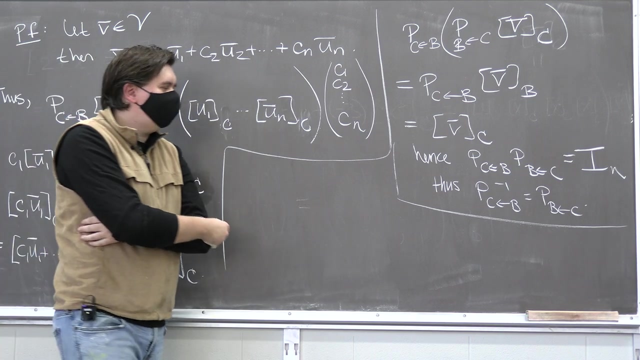 show uniqueness right, Like: how do we know there's not some other matrix That maybe does the same trick? So any thoughts on how to show uniqueness? Yeah, Essentially, In this case we're just going to say: say you have some matrix that does this. 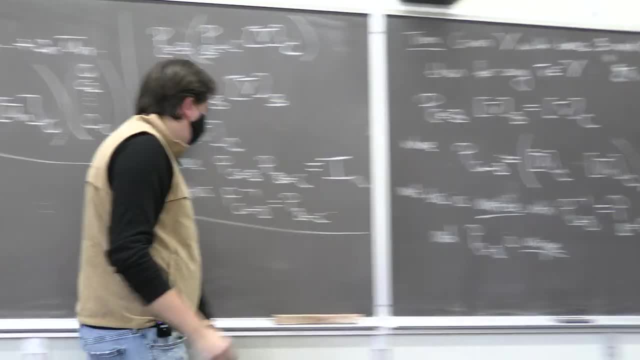 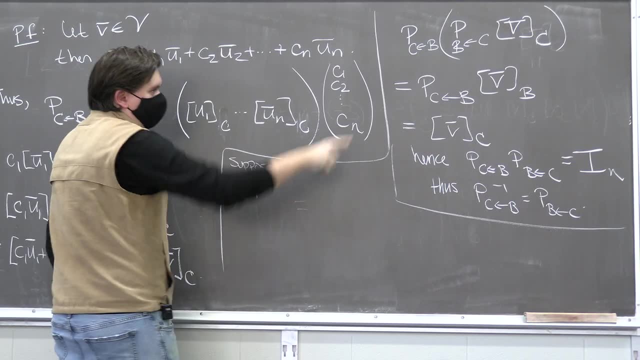 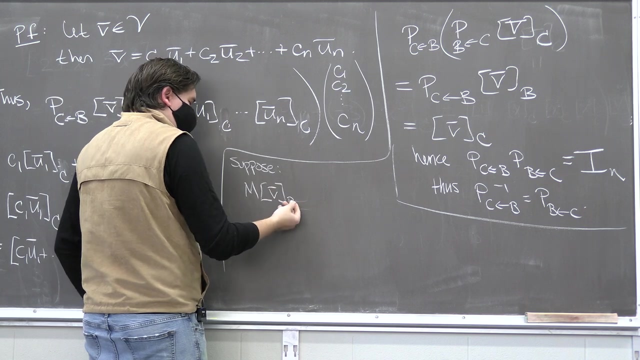 and then we're going to show secretly. it's this matrix, right. So for uniqueness you just need to suppose you have some matrix M that when you multiply it by the coefficient vector of V in terms of the basis B, you get the coefficient vector of V. 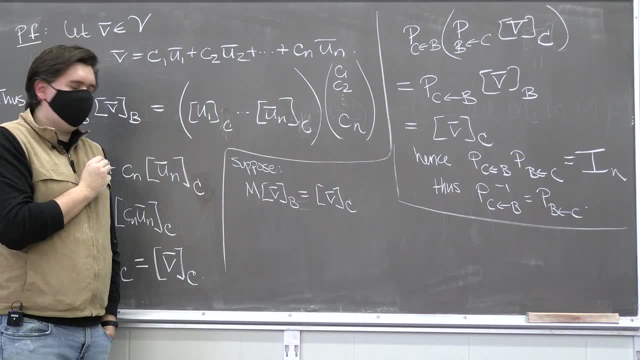 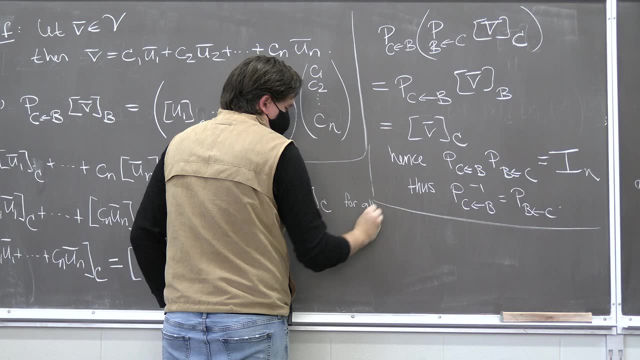 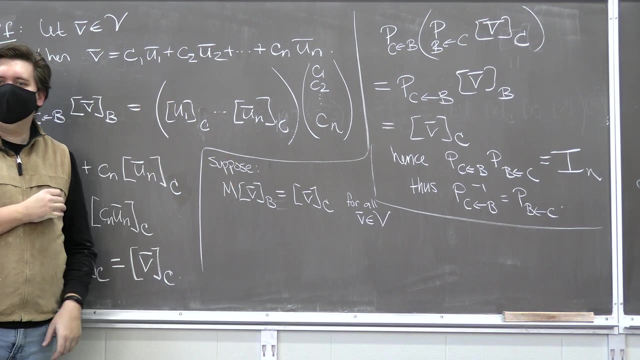 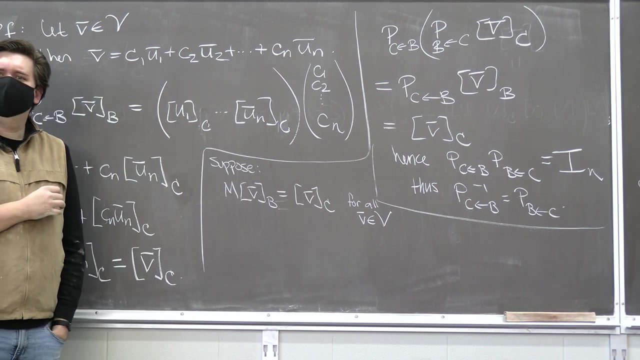 in terms of the basis C for all vectors in your vector space. there'd be lots of matrices that might do it for one or two vectors in there, right, but let's think this is one that does it for all vectors. okay, what should we do now? well, it works for all the vectors. 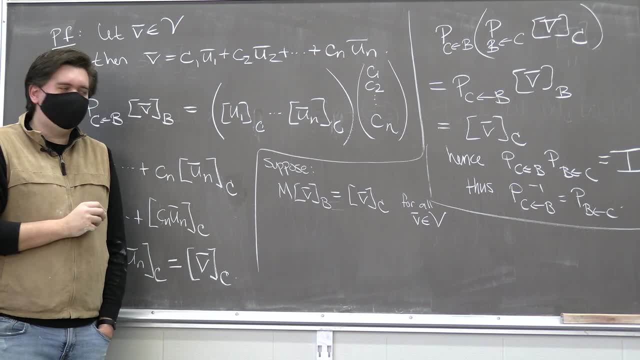 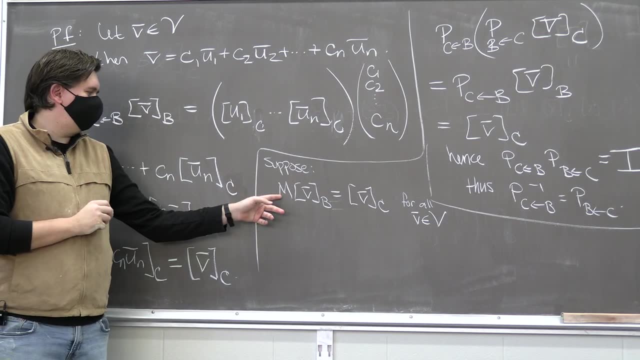 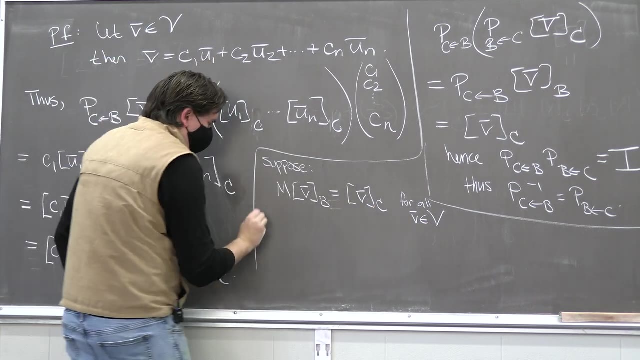 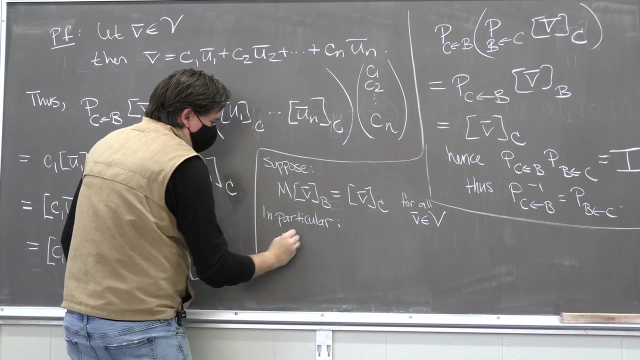 let's pick some special ones. what are some special vectors we might pick? no, you'll just get the matrix times. the zero vector is zero, not very interesting. ah, basis vectors. since this is true for all, V in particular, you know, it would be true for, say, your first basis vector of B. 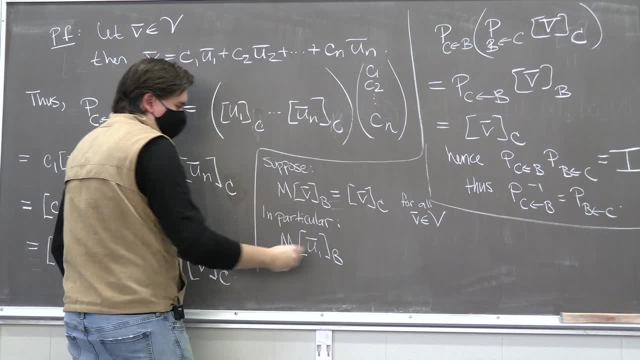 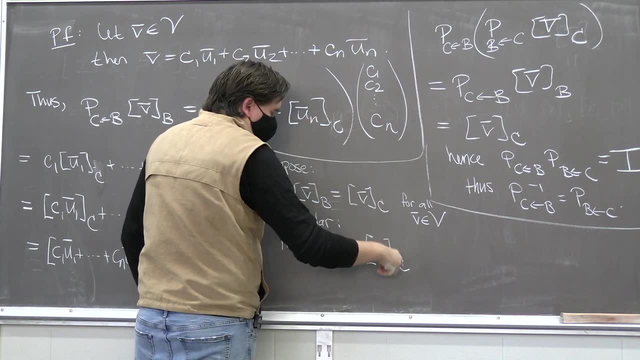 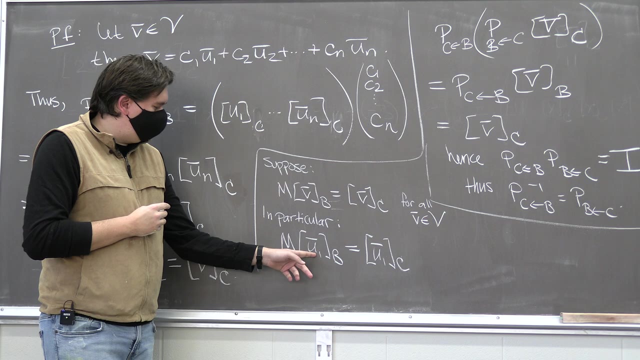 right, that is going to come out to be your first basis vector in terms of the coefficient vector for U1, in terms of the basis C. but what we're going to do is we're going to do a little bit of a little bit more math. what is U1's coefficient vector with respect to B? 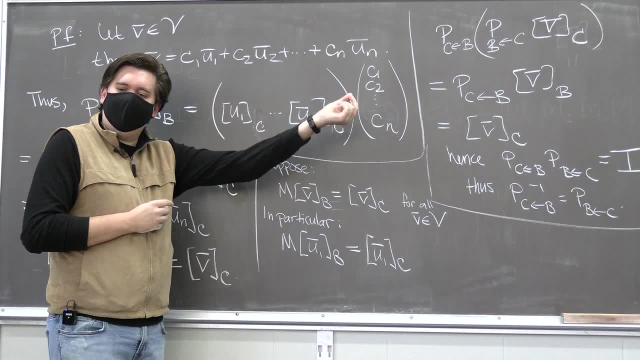 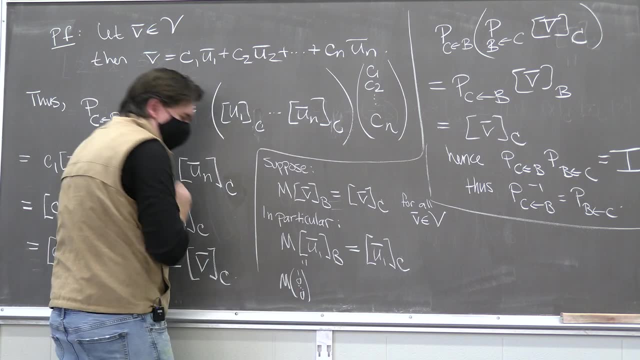 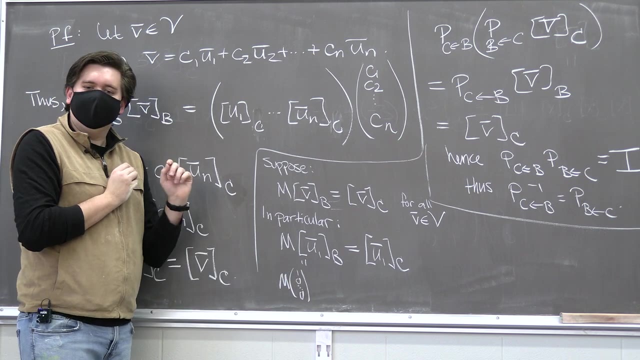 right. U1 is just equal to one copy of U1 plus zero copies of everything else. so this is really just M times 10, zzzz, 0, all way down, right. so what is this really? what is the matrix times 1, 0, 0, 1? 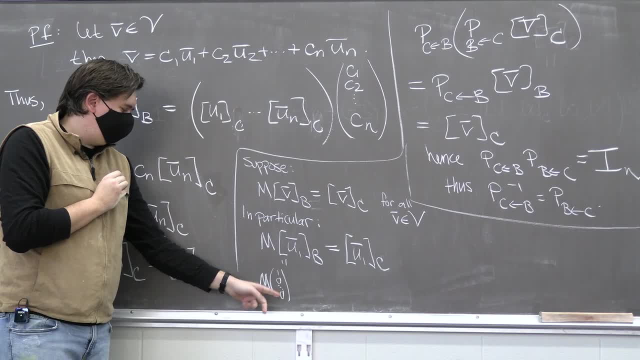 a matrix times 1, 0, zzz, 0 all the way down. what does the matrix x times 1, 0, zzzz 0, 1 it down? What does that give you? Just the first column. right, You're multiplying the entries in. 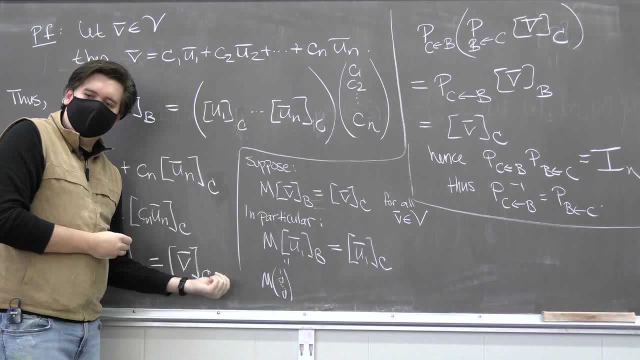 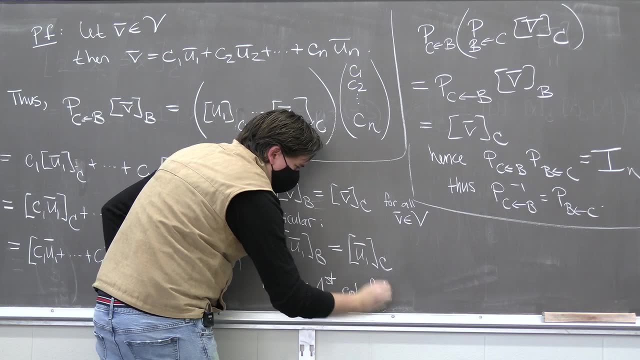 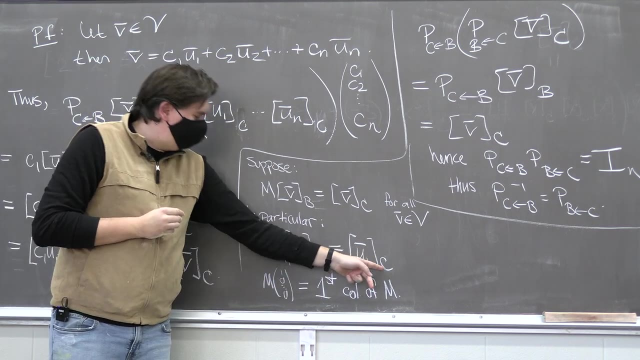 the first column by one, everything else by zero and add them together. You're just recovering the first column. This is just going to be the first column of M. Hence we have the first column of M. must be just the coefficient vector in terms of the basis C for U1. 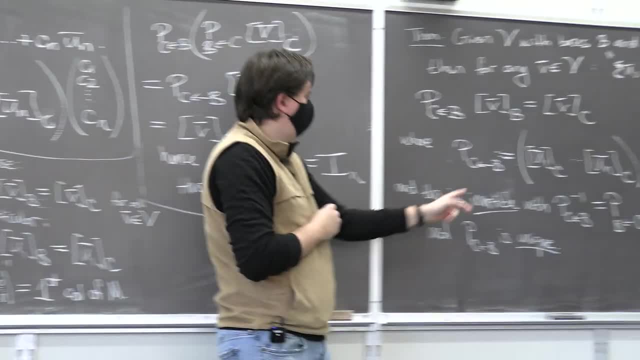 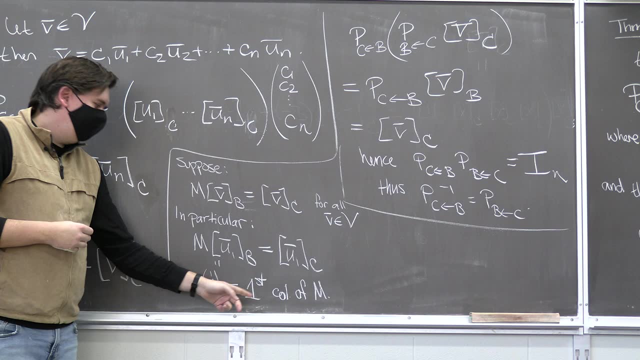 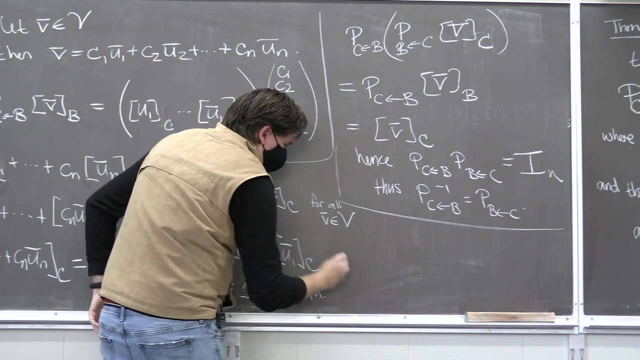 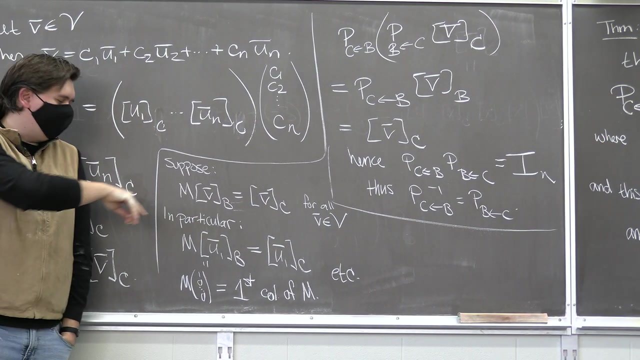 Exactly like we showed here it should be, And of course, there's nothing special about U1.. You could do the same argument for U2.. You get the second column, or U3, or in general for any UI, right And so on. right, It's true for all UIs. 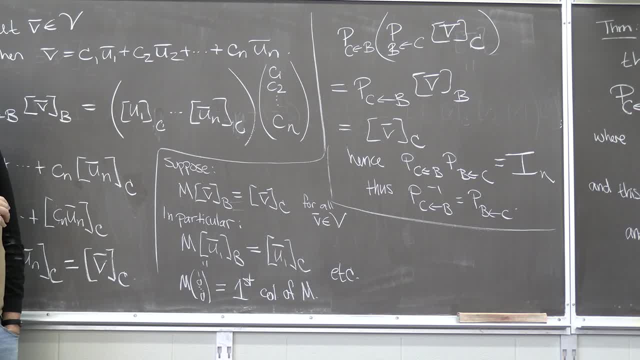 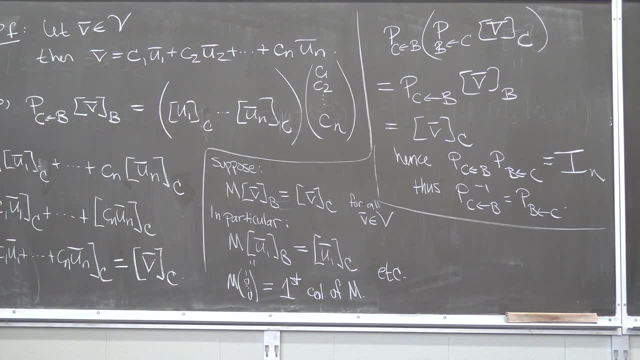 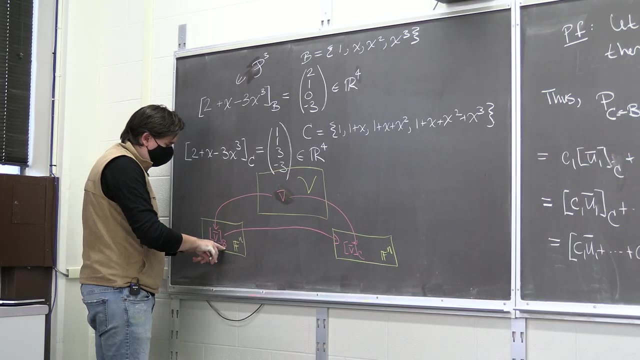 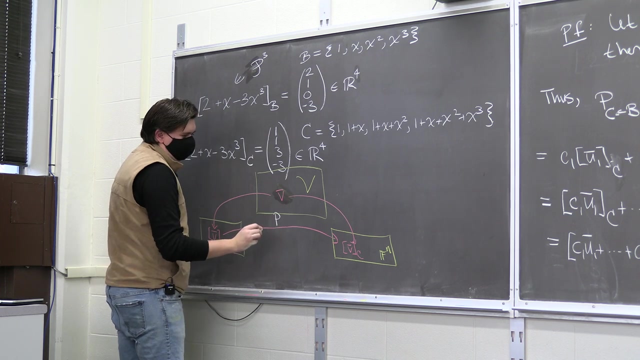 Good. So in our picture we can fill it in a little bit and we can say: to go from the coefficient vector in terms of the basis B for the vector V to the coefficient vector in terms of the basis C for the vector V, you're multiplying by this special matrix that is going to be denoted P sub. 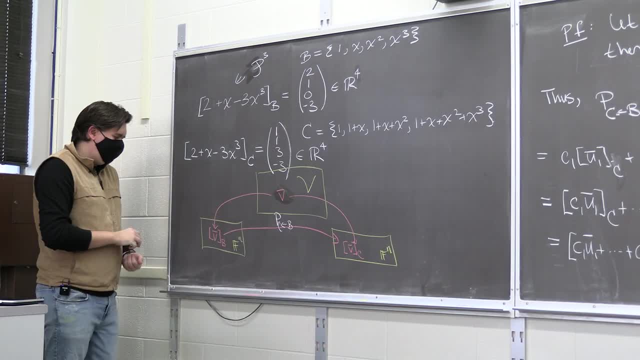 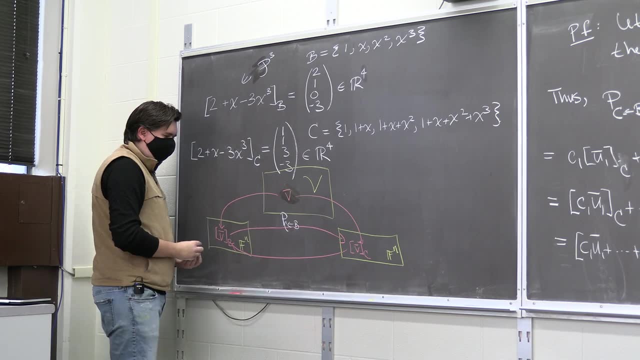 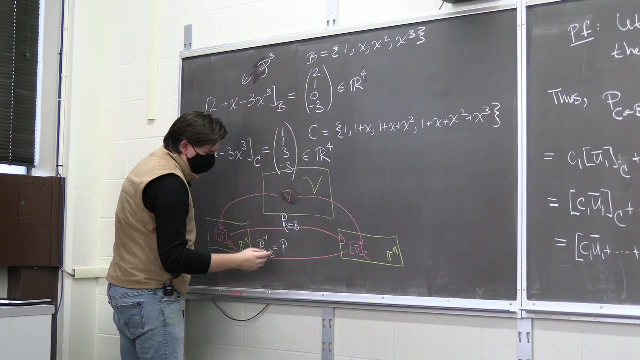 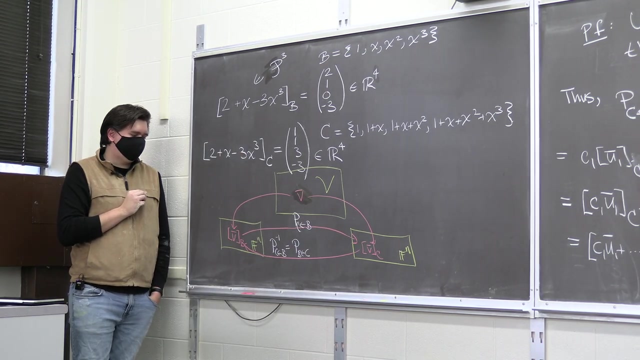 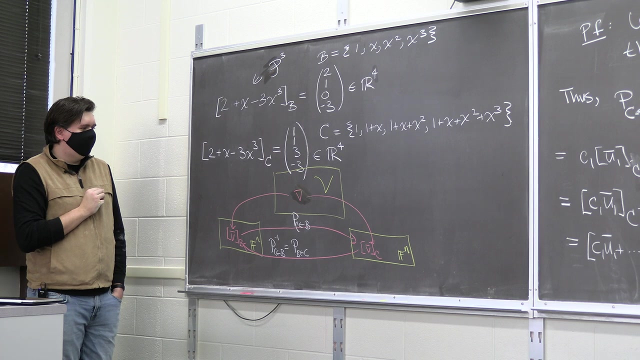 beta C And to go the other way. you're multiplying by the inverse of that matrix, which is just the change of basis matrix from C to B. So this should be a little more abstract, but very similar to what you've seen in the. 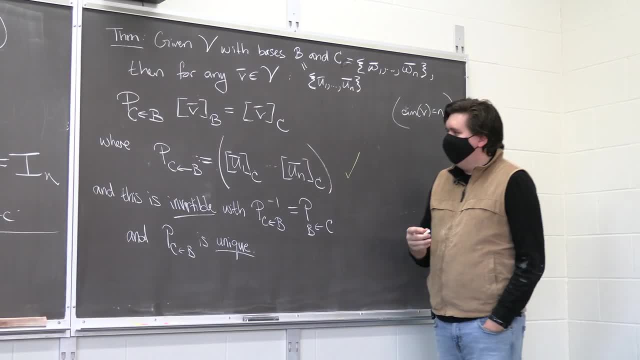 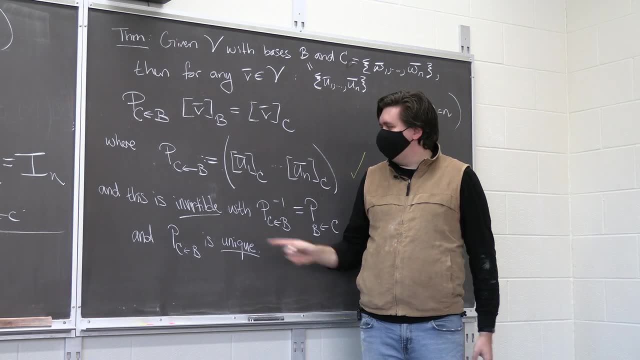 introduction to linear algebra. In your first course on linear algebra it's like how do you figure out the matrix of some transformation? Well, you just ask: what does the transformation do to your basis? vectors like 1, 0, 0, 0,. 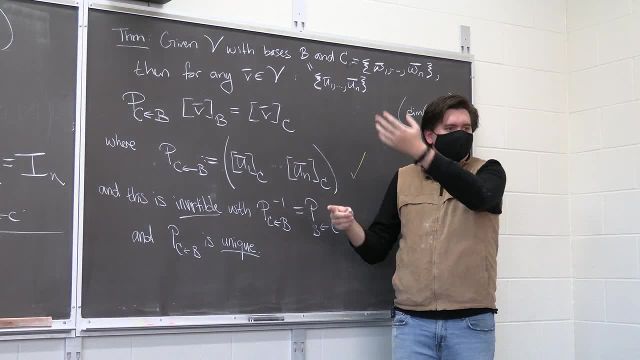 and then 0, 1,, 0, 0, and 0, 0, 1, 0.. You just look at those elementary vectors, the basis vectors, and you just ask what does the transformation do to those? 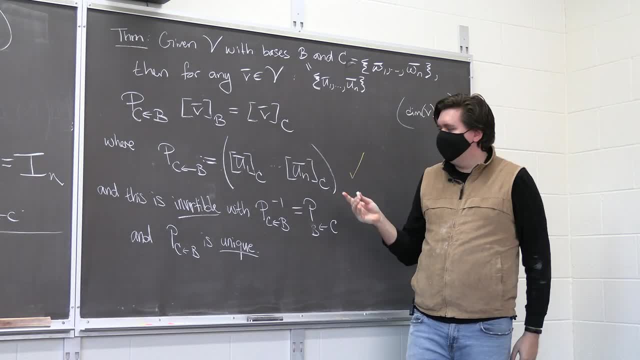 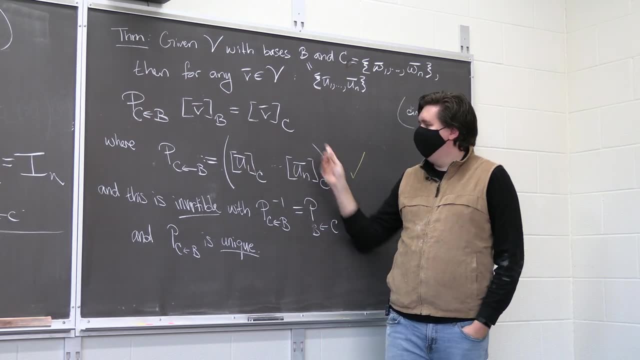 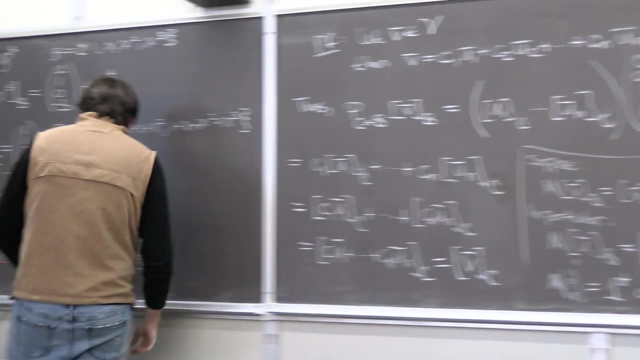 And then you recover the matrix. So we're saying the exact same thing here. So to figure out this change of basis matrix, we just figure out how the change of basis works on the basis vectors and you recover the matrix. This notation might seem a little bit strange, like: why are you writing B to C with an arrow? 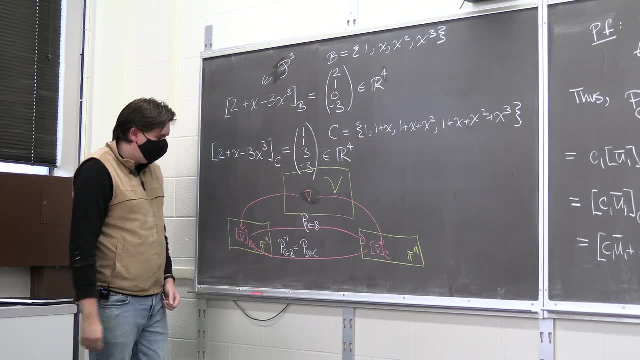 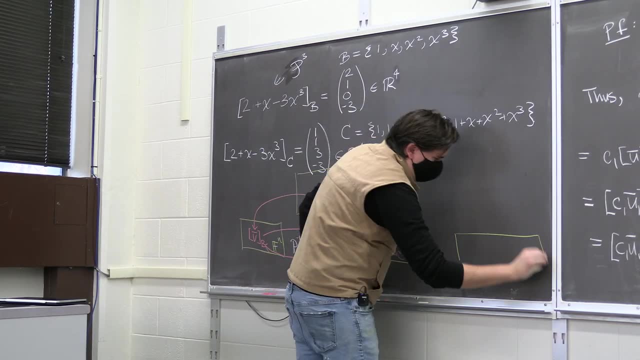 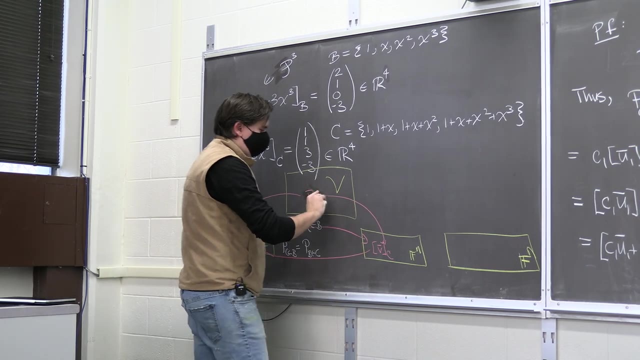 like this. It's like seems like it's going backwards, But when we start thinking about compositions of things, well, I think it's a little bit helpful. So maybe you have some third, some third basis D, And so that would give you another map that sends V down to the vectors, v down to v. 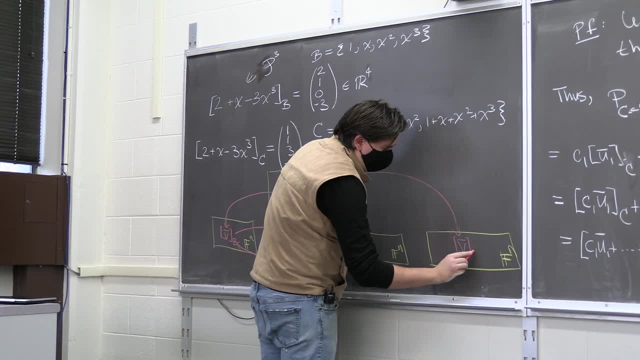 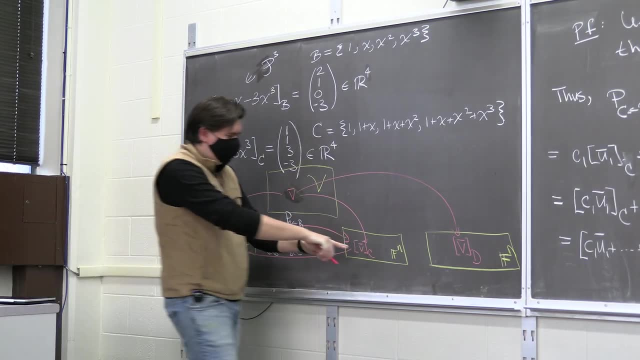 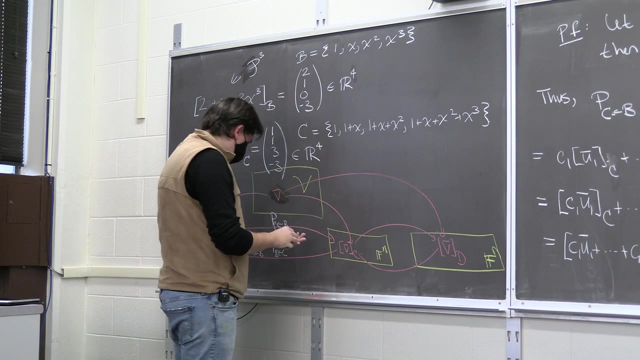 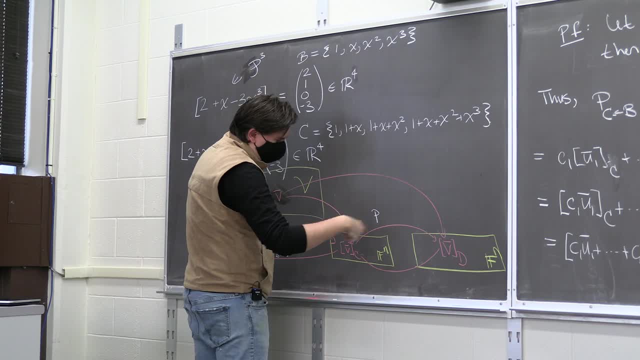 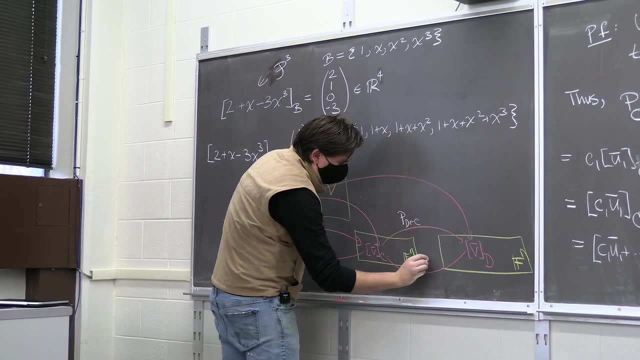 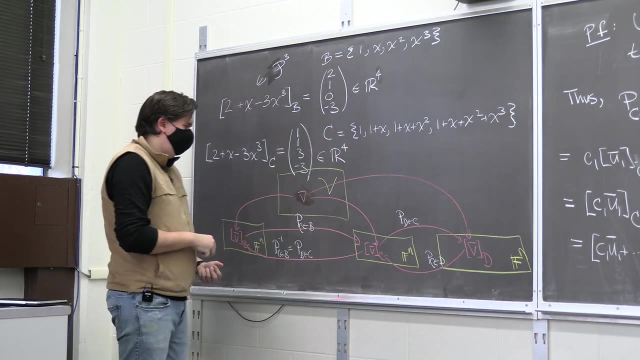 maps that converts. this is the change of basis matrix going from C to D and the change of basis matrix going from D to C, which is, of course, the inverse of the guy above it. but then it's like: okay, what if I want to know what is the? 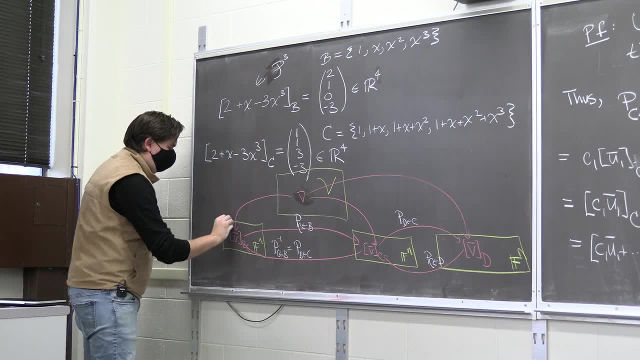 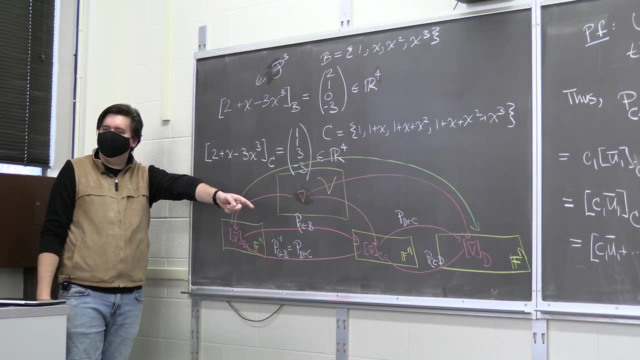 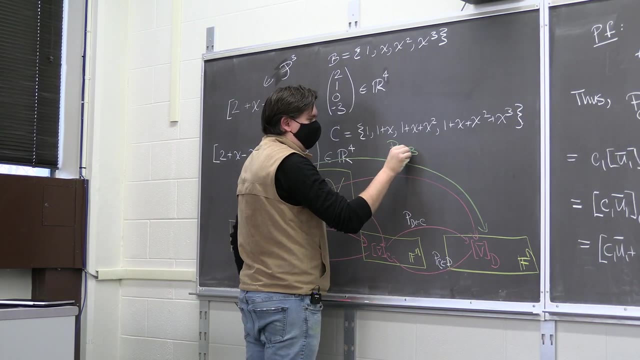 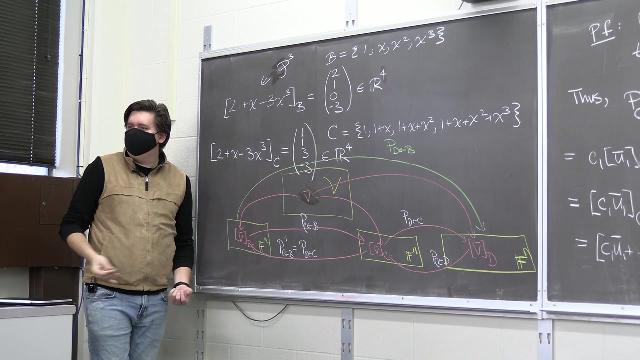 change of basis matrix to go from B all the way to D. like what is that guy going to be? what is the change of basis matrix to go from B all the way to D? so this is no mystery. you can just tell me. how do I figure out? 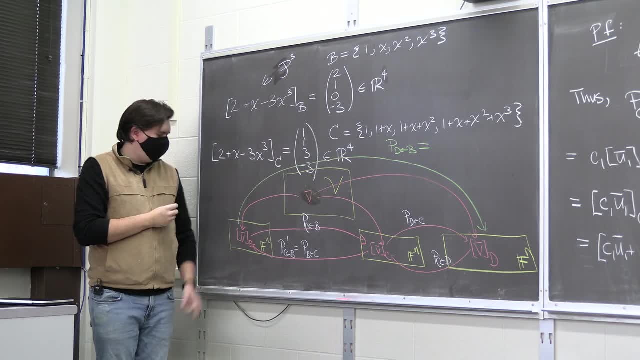 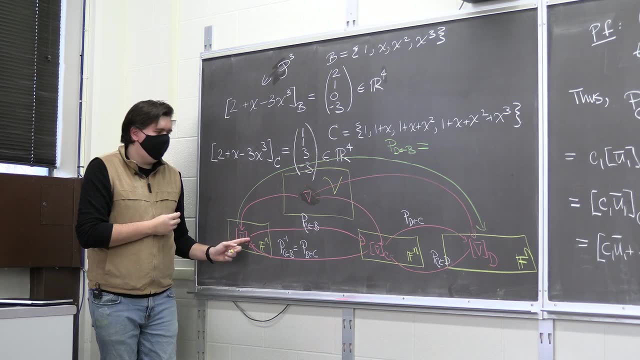 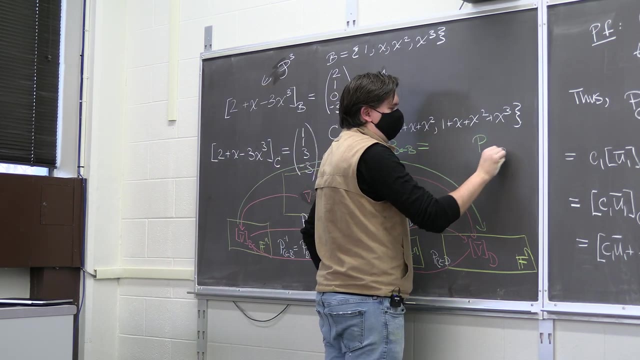 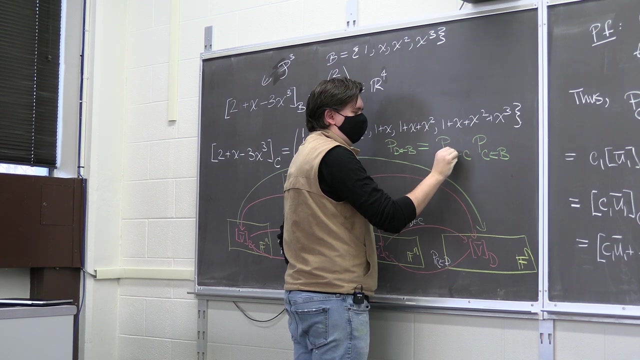 what this matrix is. well, how can I go from here all the way there? hey, like one step at a time. right, so to go from B all the way to D. first I want to go from B into C, and then I want to go from C into D. right, if I wrote the arrows, the other. 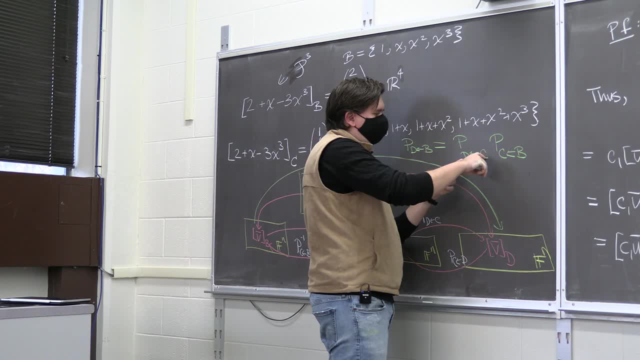 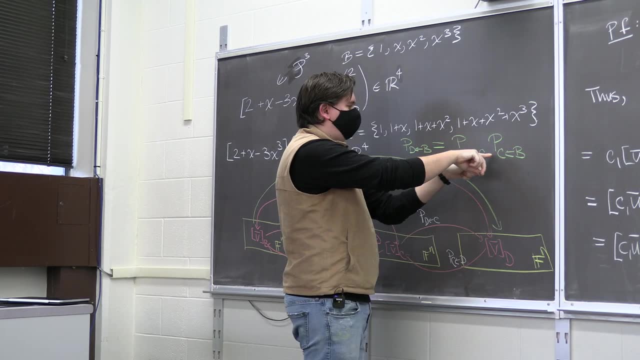 direction. you know, maybe you wouldn't see as well. it's like C to D, B to C. it wouldn't look as clean, but when you write them this way it's like: well, now you get to clear. this is going from B, stopping along at C, headed to D right. so 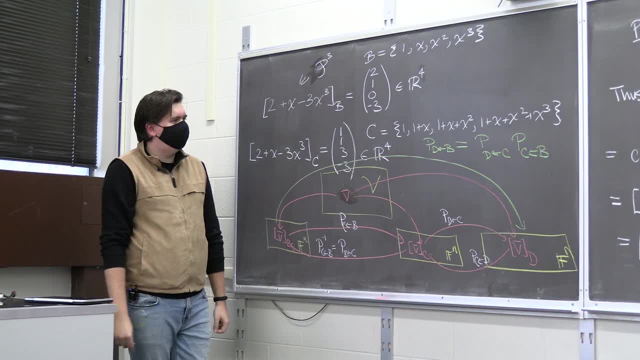 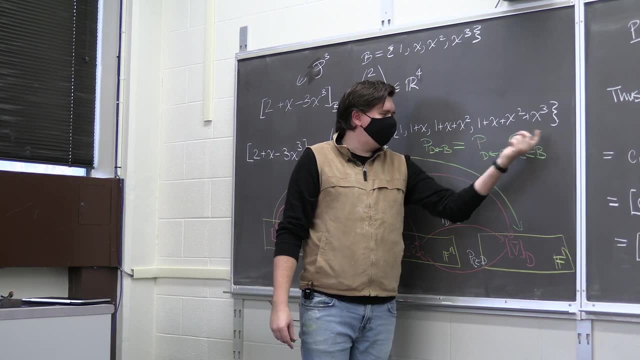 maybe this justifies the notation a little bit, because if you have any vector expressed in terms of a coefficient vector of coefficients on B, this changes it to that vector of coefficient vectors in C and this changes it in terms of the coefficient vectors in terms of D. and then, since we know that there's only one, 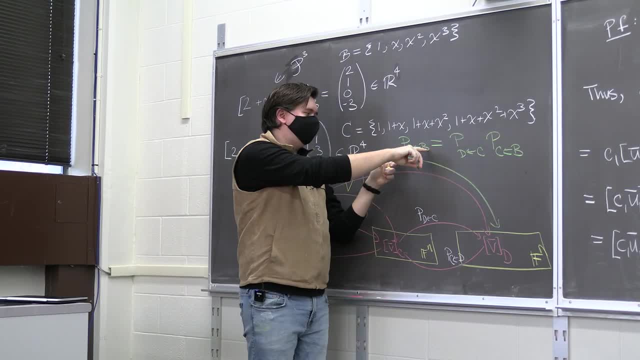 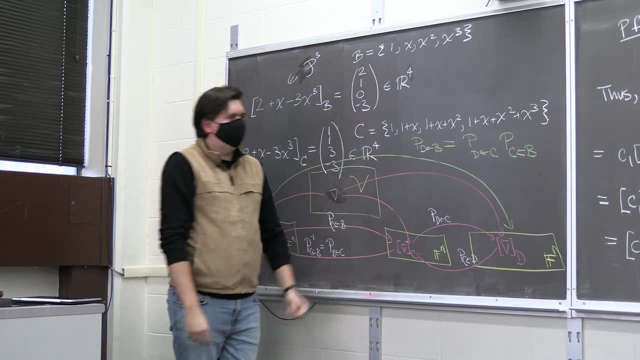 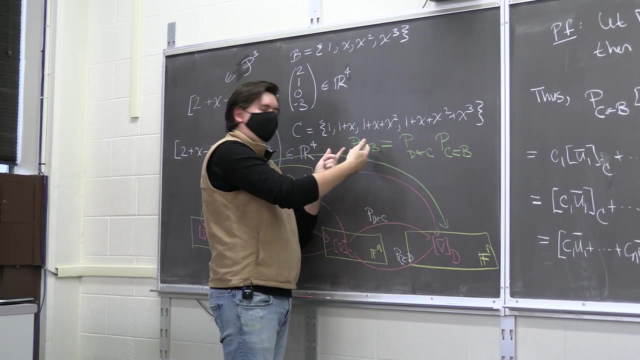 matrix that does that. the matrix is unique. we have therefore this matrix, since does the same thing, must equally be the same as the multiple of those two matrices. so we're taking advantage of uniqueness from the theorem to say, yeah, he must actually equal that product, since the product accomplishes the same. 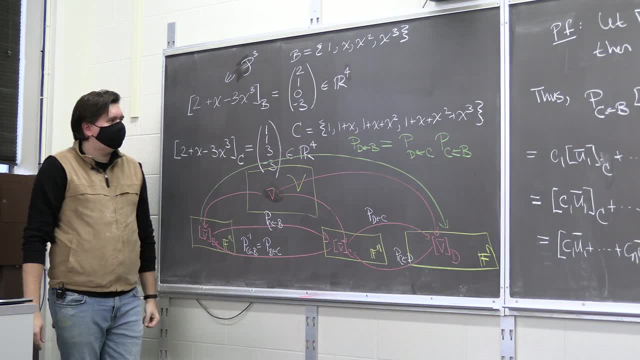 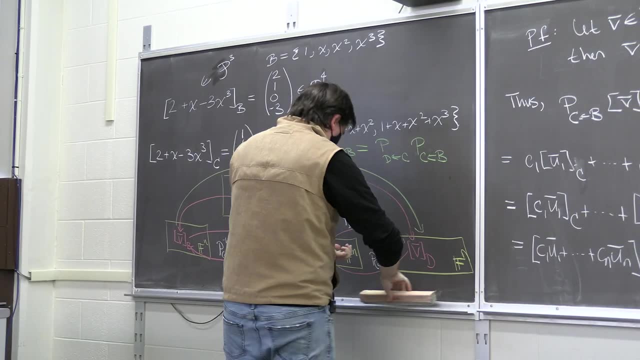 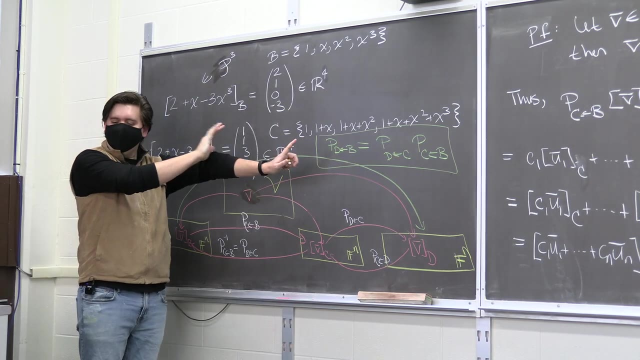 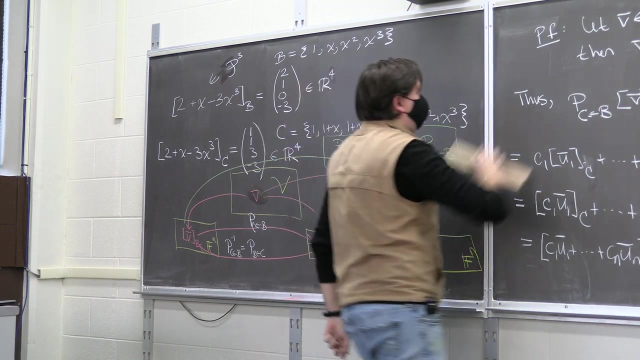 thing that he accomplishes, that is, let me just write this down like as low property. well, I guess the property is right. here we have this composition, but in general, this is going to be really useful to well, let me give you an example. let me give you an example. 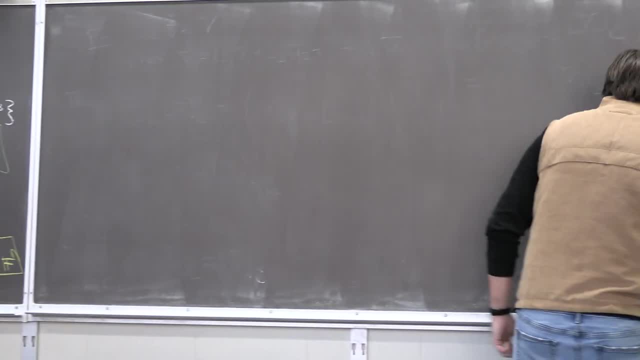 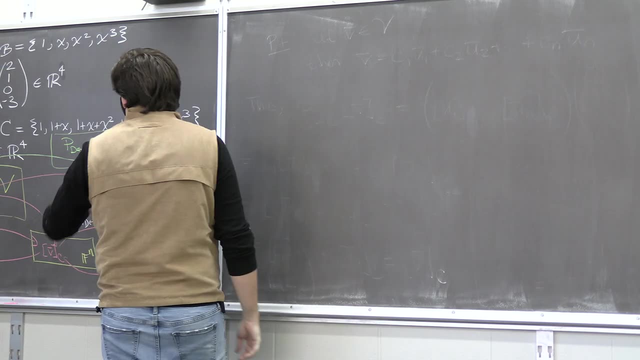 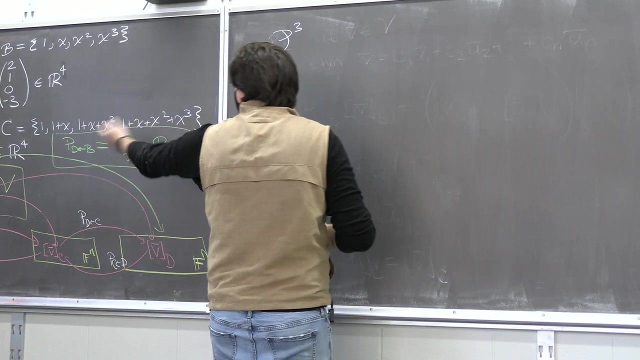 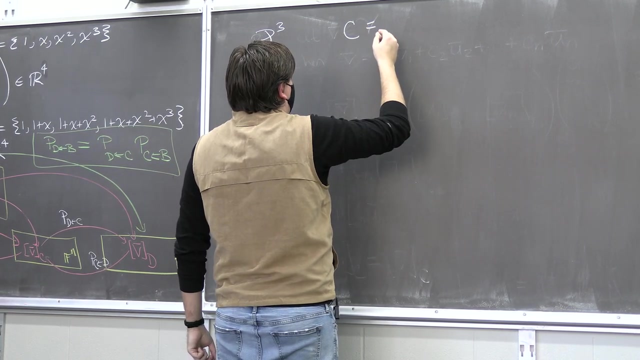 do we want to stick with with this first guy, with these coefficients? I mean we can so. so here we had P 3 and we had some basis. you know, like, say, the basis C, which was an ugly basis, was the basis 1, 1 plus X. 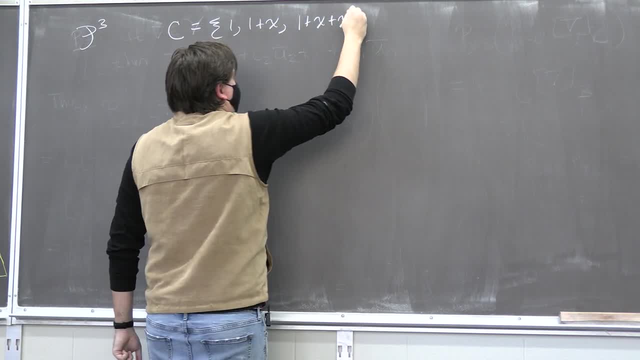 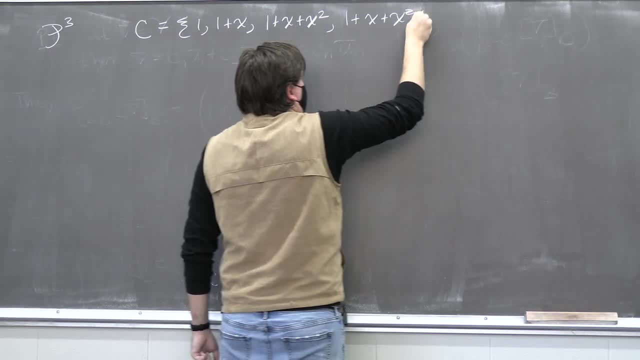 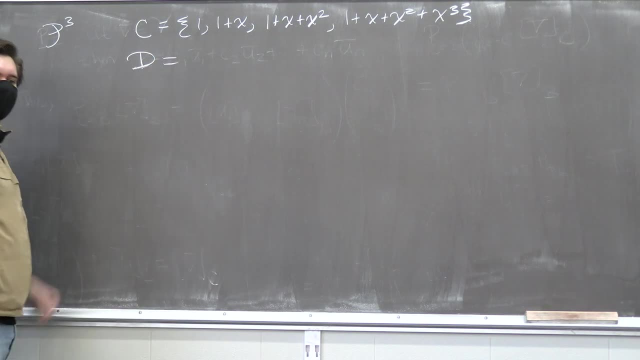 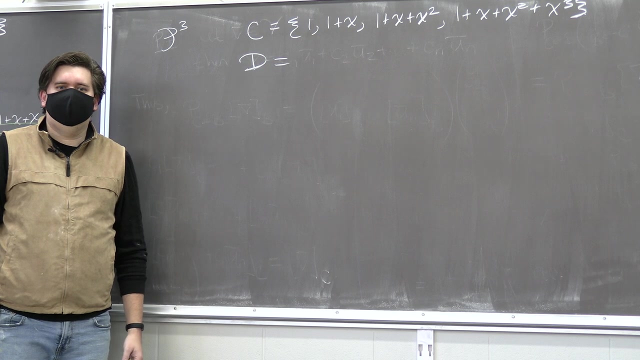 1 Plus 2, 1 Plus X, 1 x 1ux squared 1 one plus x plus x zl plus X Q queed u packing ugly basis, ugly basis. once another ugly basis. what's another ugly basis? you don't make one up. 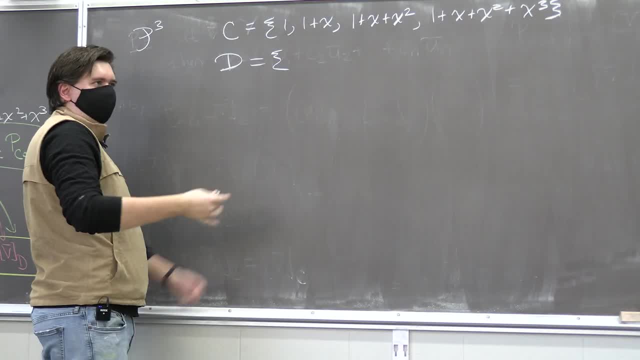 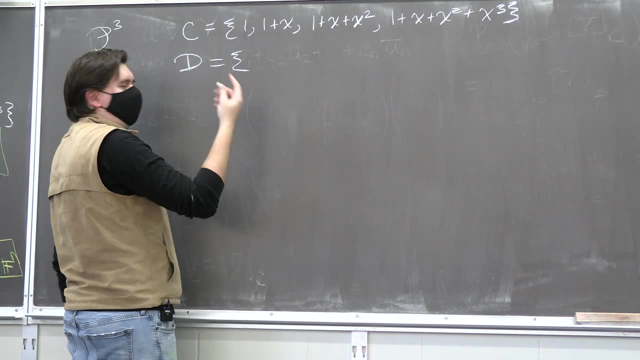 let's just make up something and you know we'll squint our eyes at it, convince ourselves. it's a basis and if you want to go home and check it's a bit basis you can name. instead of a one we can put like a two. it's scale. so 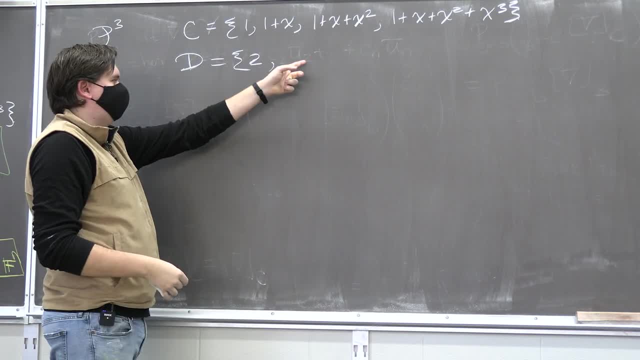 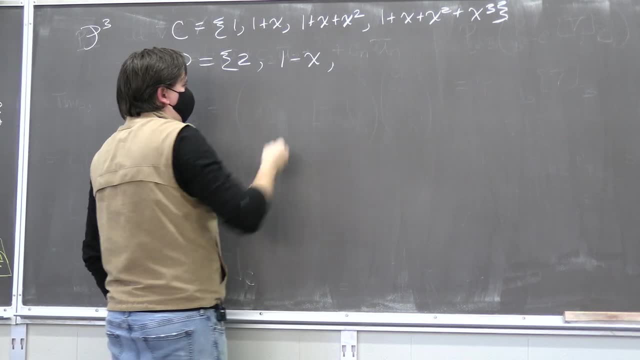 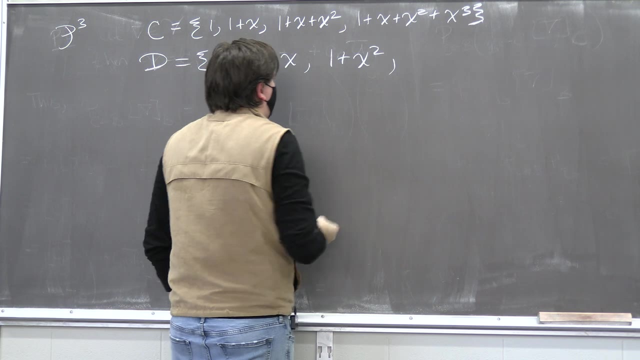 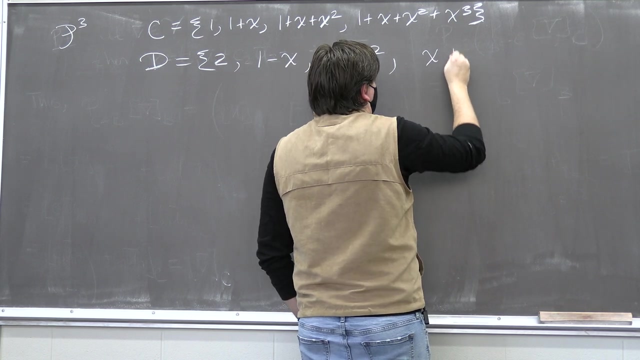 that's fine, right, we want something in the second world. I like eventually give us an X, one minus X, that's just good. to be chaotic, that's great. and then we maybe make this like one plus X squared, and then maybe here we'll have something like X plus two X cubes. okay, so, like usually, convince yourself this. 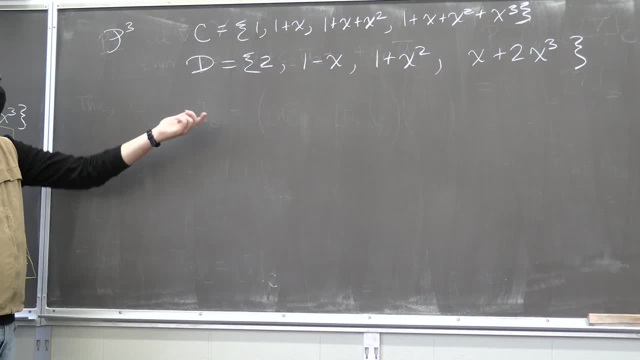 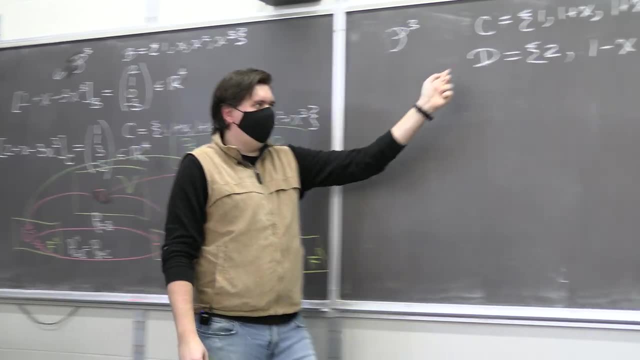 is really a basis. maybe doesn't look like a basis, but the way to convince yourself is that you can get all of these standard guys- one X, X squared and X cubed from these guys and and you can, you can scale it up and you can scale it up, and you can scale it up and you can scale it. 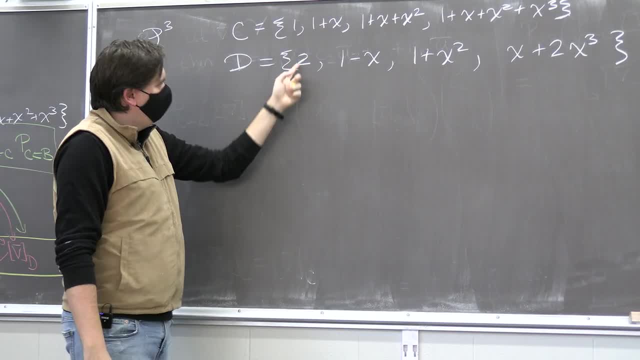 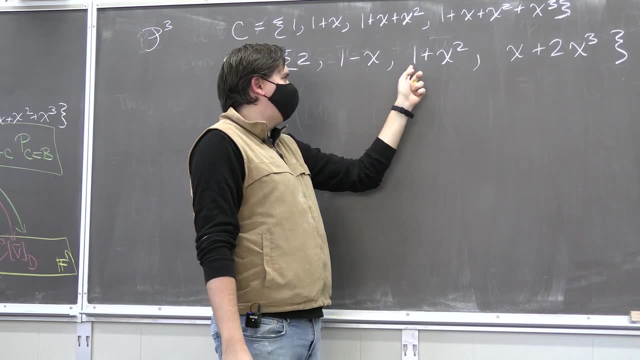 this by a half, you get one. once you have one, you can subtract it from this guy, you get negative X. scale it by a negative one, you get X. now you have one, so you can take away one from this to get x squared. you had an X we got from. 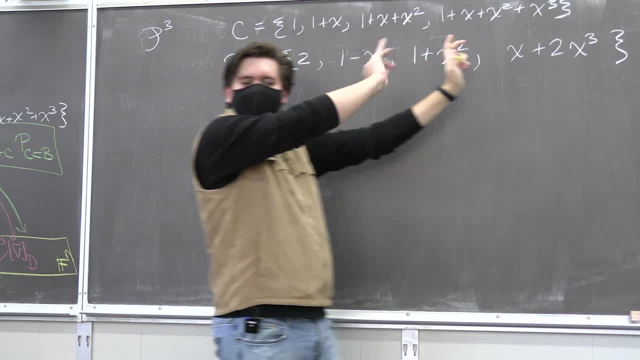 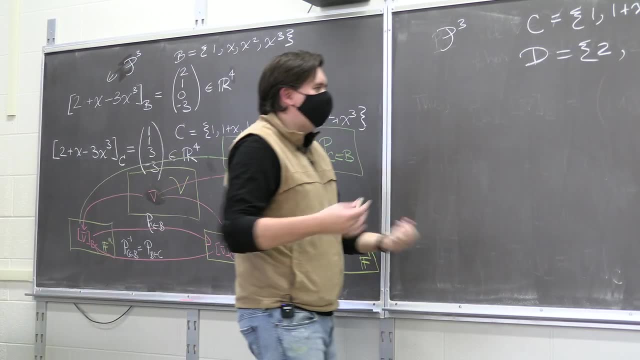 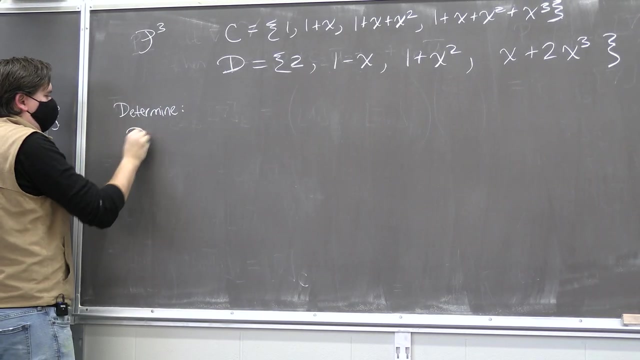 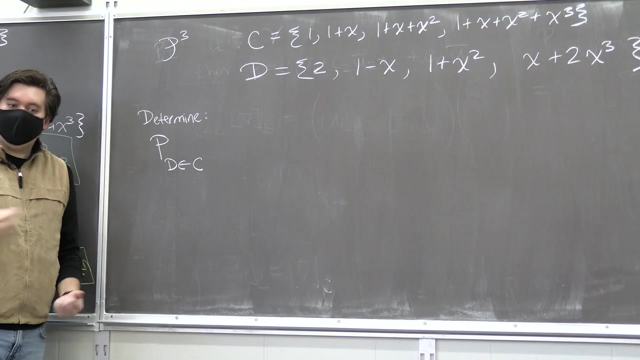 before us take it away from here, and then you can scale by a half right, so you can recover these standard basis from this guy. okay, so let's say I wanted you to calculate insults, the change of basis formula to go like from c to d. so well, one way to do this. 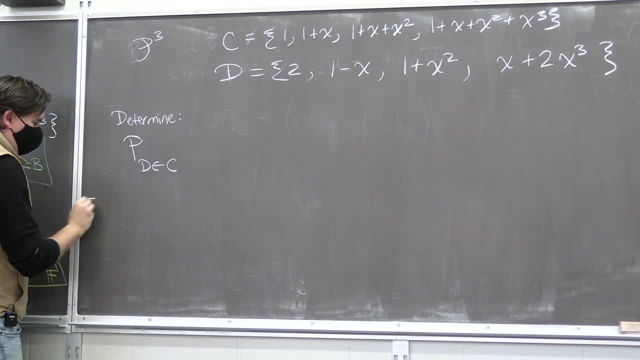 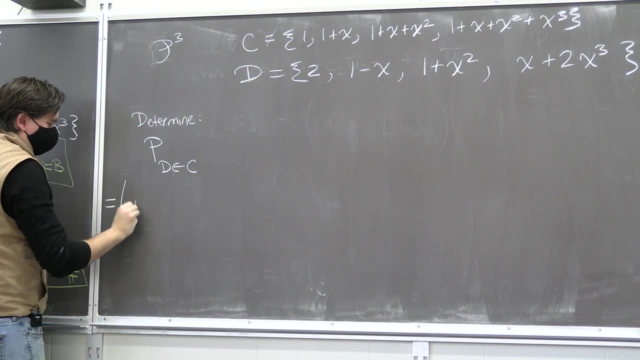 is is you want to take each of these guys and see and express them in terms of the coefficients of guys. indeed, so you like, when I take the first guy one and express that in terms of, in terms of the basis D, you want to take the second. 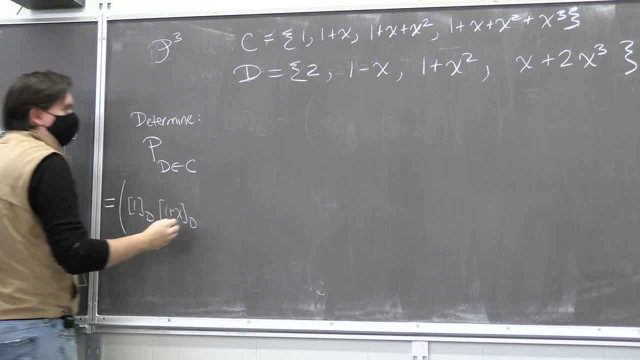 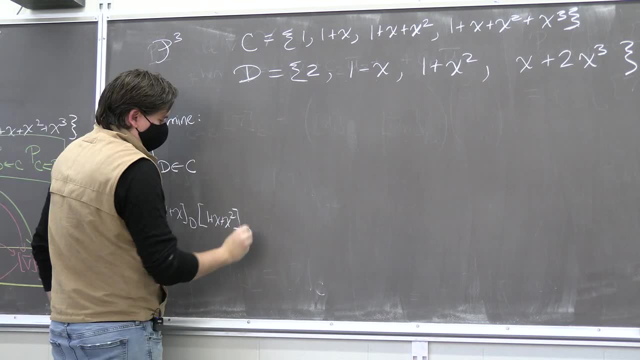 guy enter mm. I get blue. so very som voluco hedge. that kind of silly we don't don't. one plus x. express that in terms of d. take the next one: one plus x plus x squared. express that in terms of d. 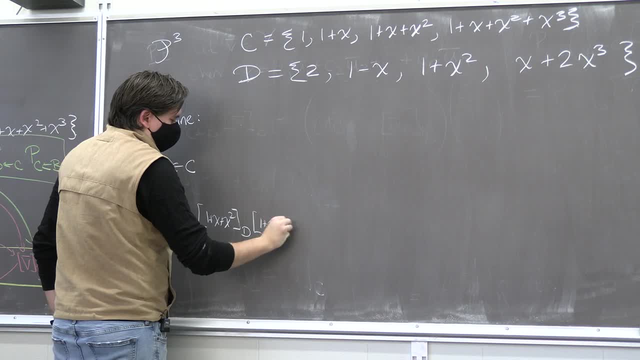 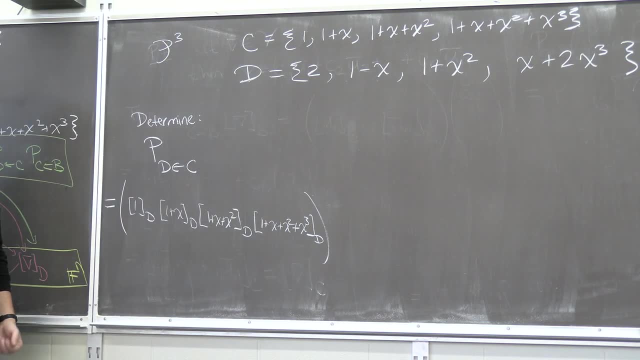 and then take the last one, one plus x, plus x squared, plus x cubed, and express that in terms of d. Now you can do this, but like it sucks, right, The first one's not so bad, right, Like this first column. what's the first column? 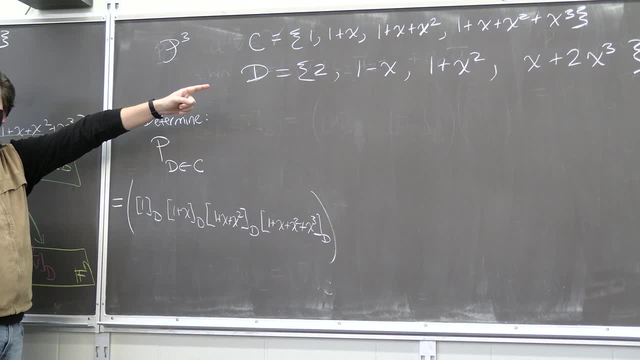 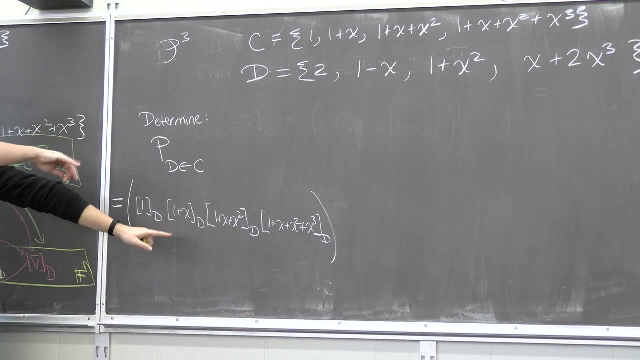 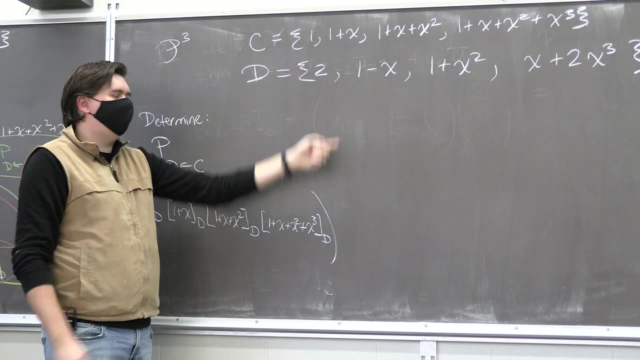 What is one expressed in the second basis? Yeah, half of this and zeros of everything else. So like you can do it, you can do it. I actually don't think it'd be too terrible. but you can imagine, in general, going from some ugly basis to another one. 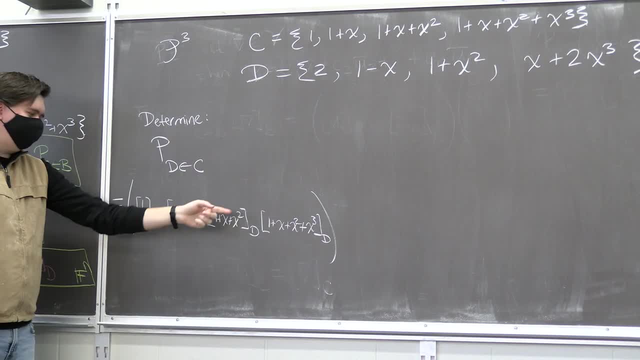 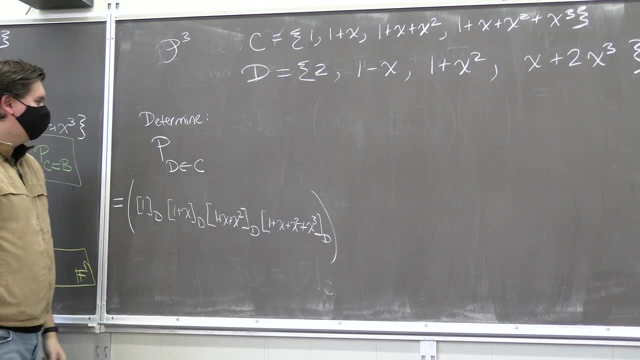 this could be quite a tedious path. You would have four systems of equations you have to solve right, which is kind of gross. So each of these is a linear combination of these other ones. So what can we do instead? Well, this reminds us that, instead, 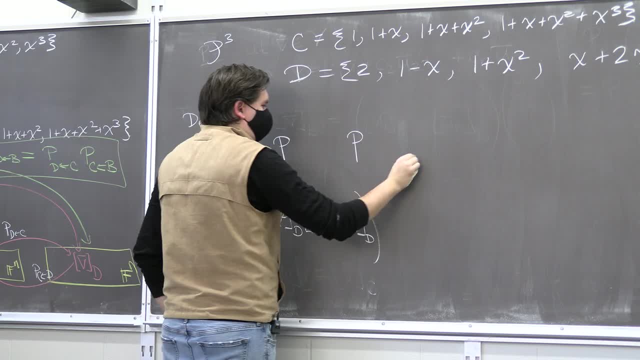 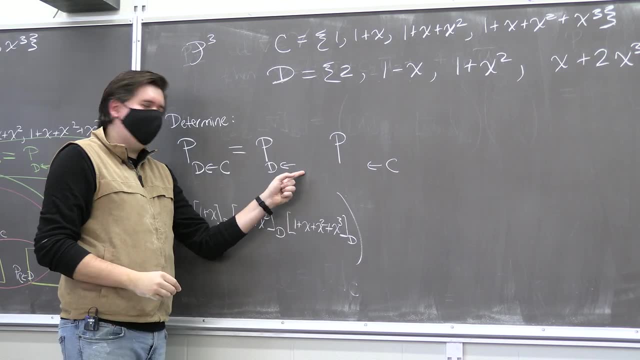 we could think of this as a multiplication of C into something else, and then that other thing into d. So it's like: what should that something else be? Is there something else that's nicer for us to work with? Yeah is like: well, this is b. 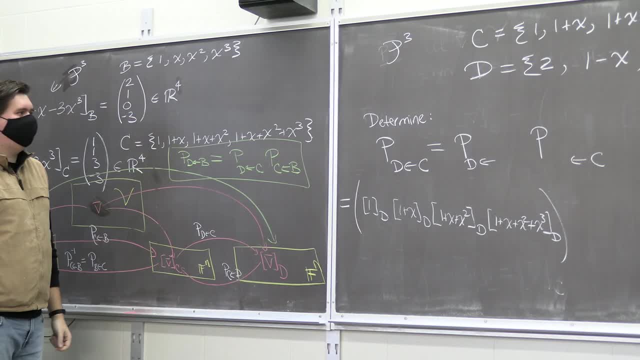 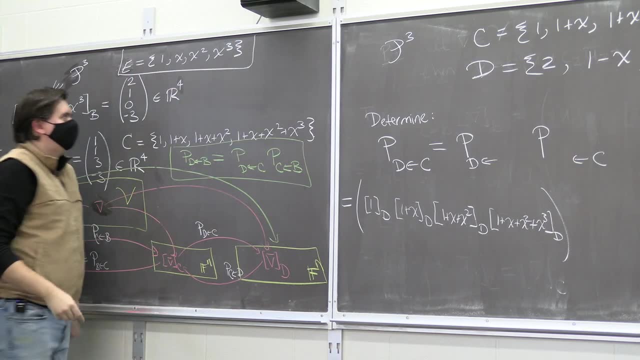 is quite nice for us to work with, Although typically, from the standard basis, it's done at E, so I'm just gonna make a quick change and call this E, just to stress it's a standard basis. It's the one that's nice to work with, okay. 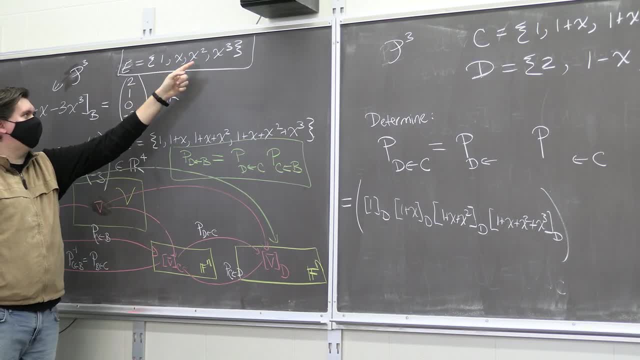 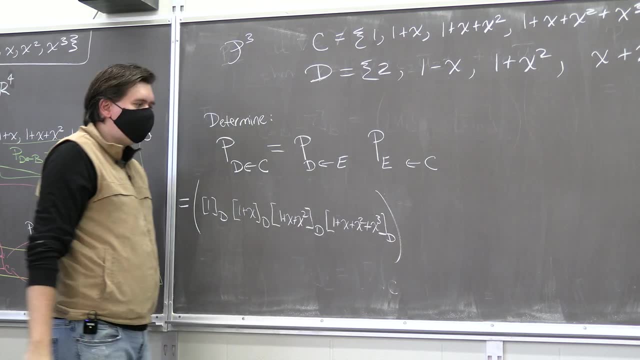 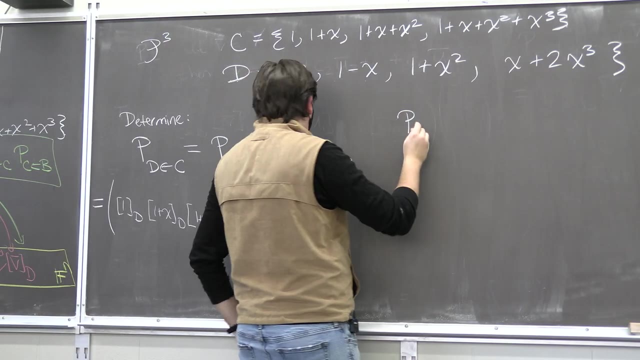 I'm gonna call it E standard basis with just one X, X squared, X cubed. So pass in the middle first through E, And let's just see how nice this is. So let's check out this guy: PEC. 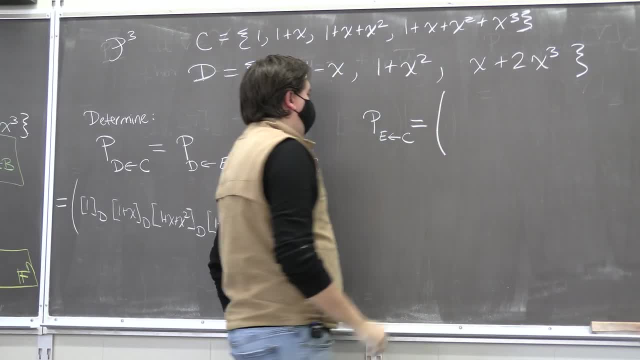 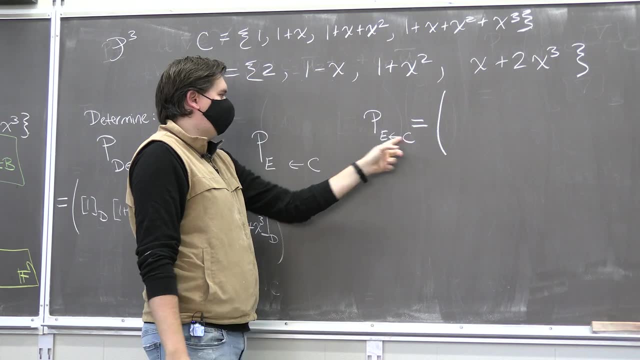 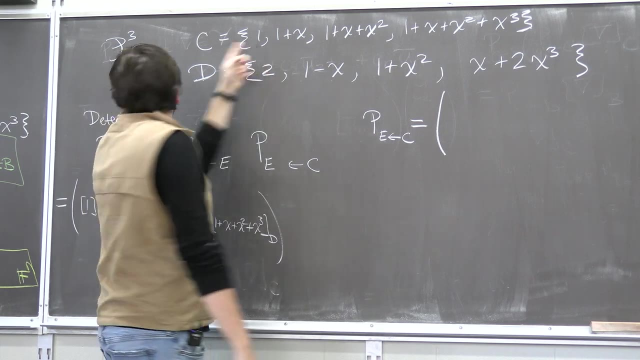 All right, It's saying express. I mean, how do we solve this? We're gonna take each of the vectors of C and express them in terms of the standard basis E, right? So what is this first guy in terms of the standard basis E? 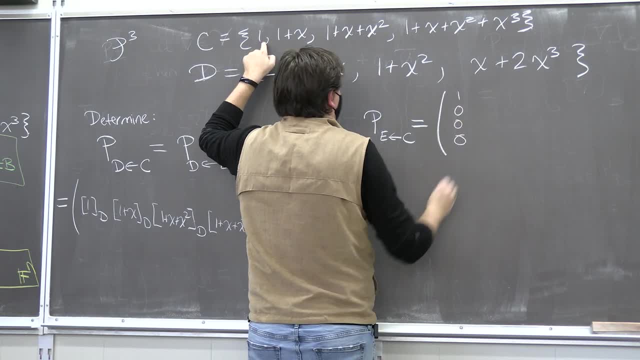 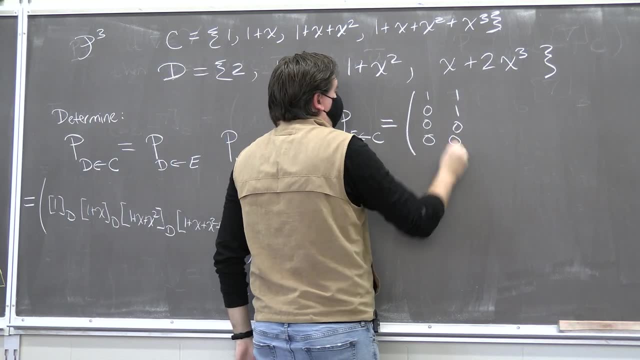 Well, it's just this first guy, again One, the first guy, nothing else. But how about him? What is he? Yeah, one, one, zero, zero. And like how about him? A, two, three, four, five, six, seven, eight. 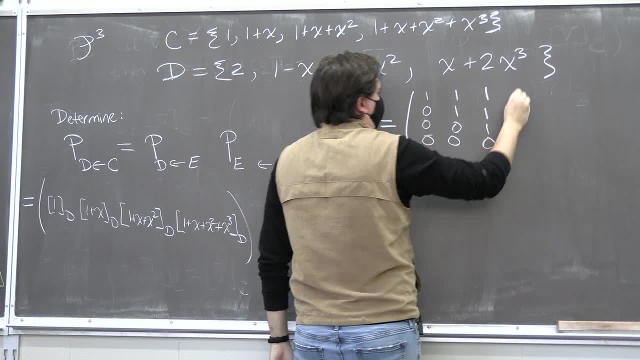 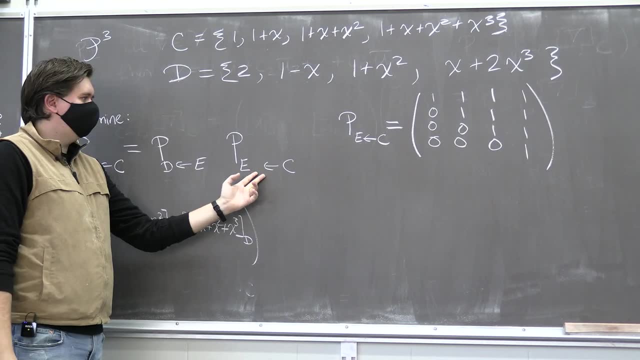 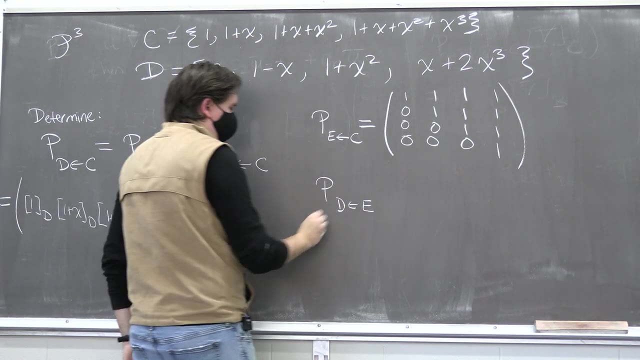 Yeah, it's just the sum of the first three And this guy Just the sum of the first four. Nice, So, like this one was super easy for us to determine How about this guy. How about P, E to D? 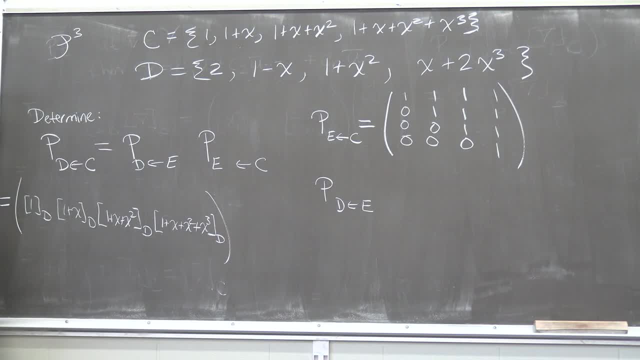 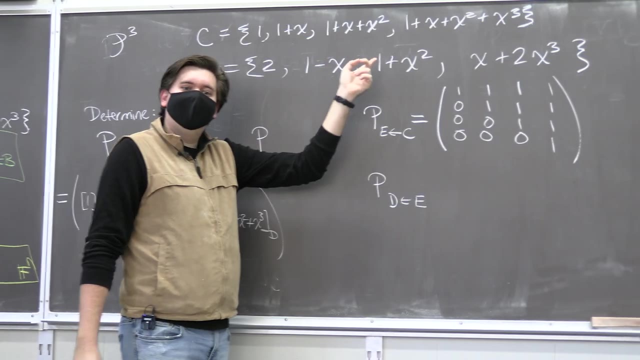 You're like: well, now it's a little bit harder, because now we're trying to take the elements, the vectors that form the standard basis and convert them into this difficult basis. That's a little bit harder. It's like it's much nicer to go the other direction, right? 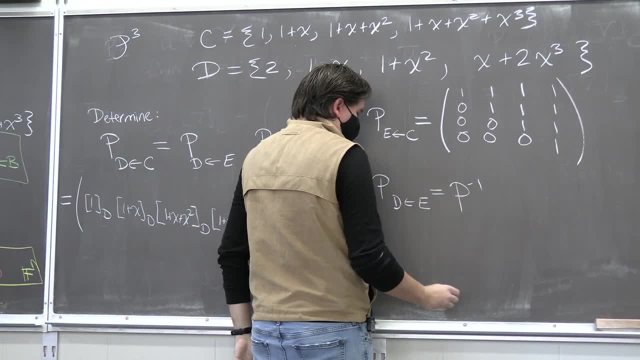 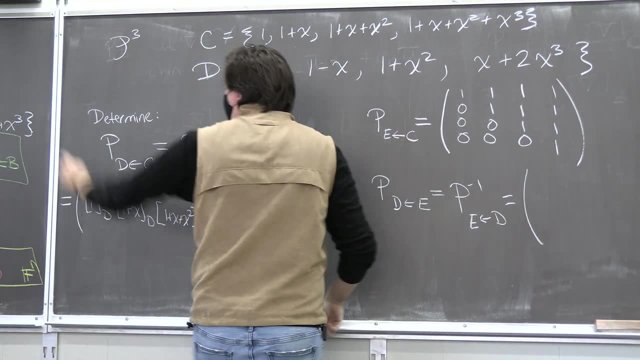 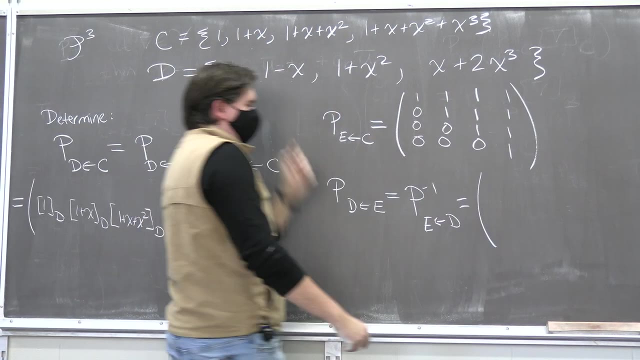 But we can go the other direction, because this is just going to be the inverse of going the other direction. So let's just figure out how you convert d into the standard basis and then we'll take the inverse of that guy. So we've got d. so the first guy is 2, which is just 2 times the first element of your. 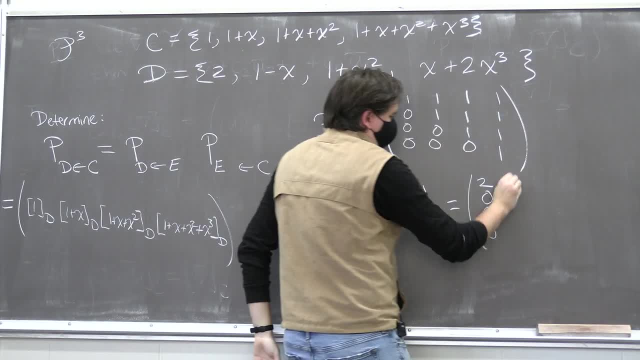 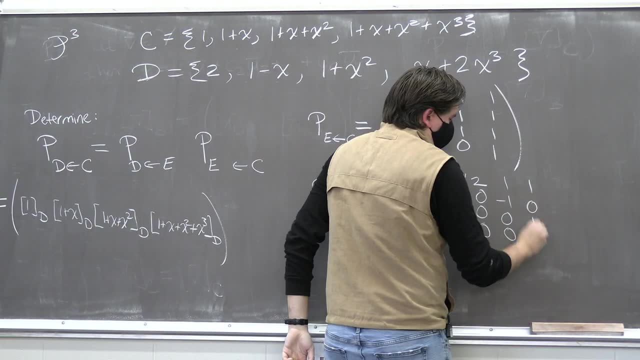 standard basis. The next one was 1 minus x, so that's just 1 minus 1, 0, 0.. The next one is 1 plus x squared, so that's just 1, 0, 1, 0.. 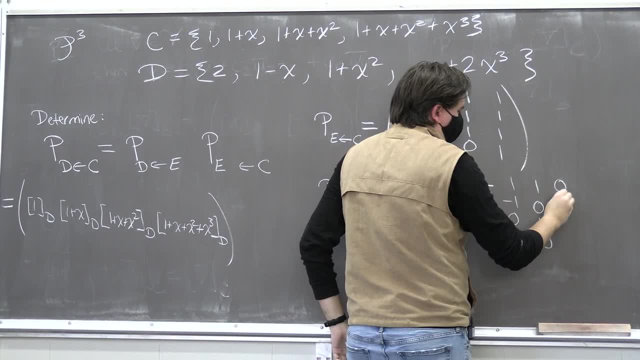 And then it's x plus 2x cubed. so 0 copies of 1, 1 copy of x, 0 copies of x, 0 copies of x, 0 copies of x, 1 copies of x squared and 2 copies of x cubed. 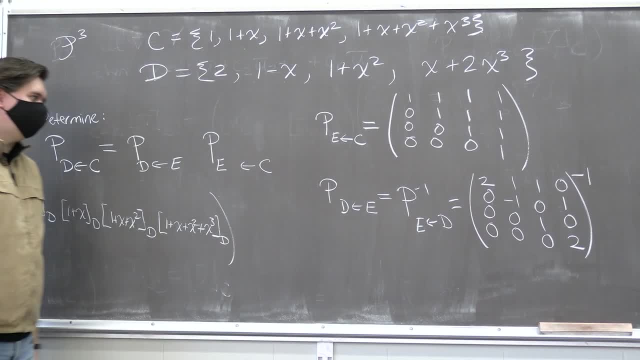 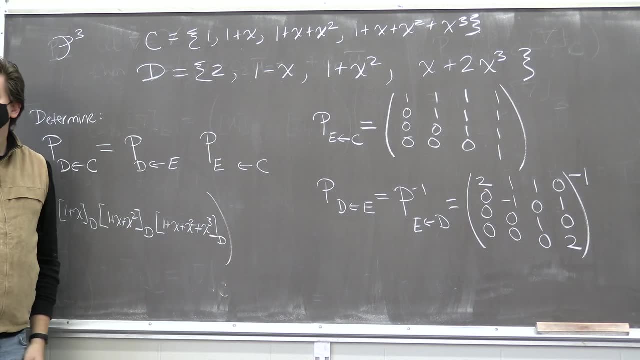 And then we can find the inverse of that matrix. Now, in practice, maybe it's a pain to find the inverse of matrices, but this is a very easy thing to program right. So maybe right now someone should pull up some little calculator tool or website and 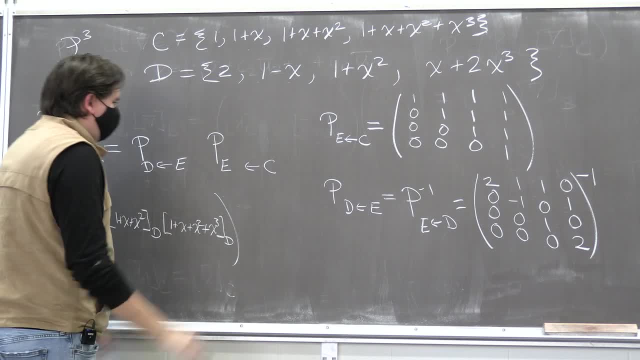 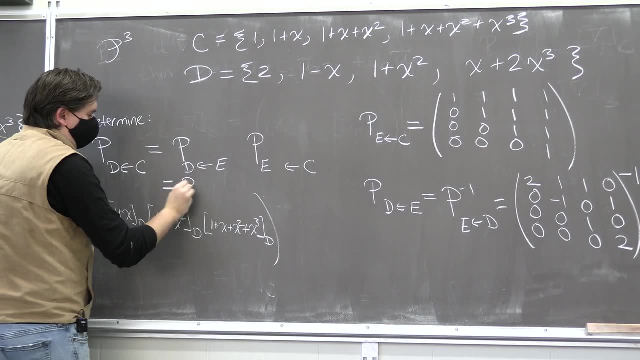 find the inverse of that matrix. But while we do that- I'm just stressing to calculate this Really- the process that's really easy to follow is instead, in practice, you're going to be calculating this guy, You're gonna just think: how do I change things? 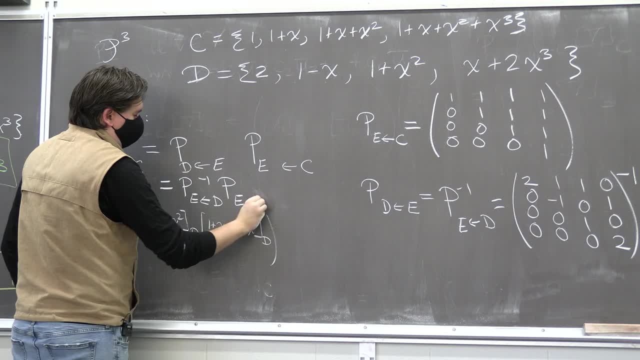 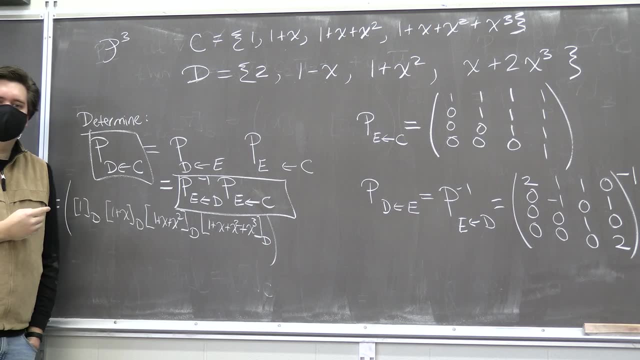 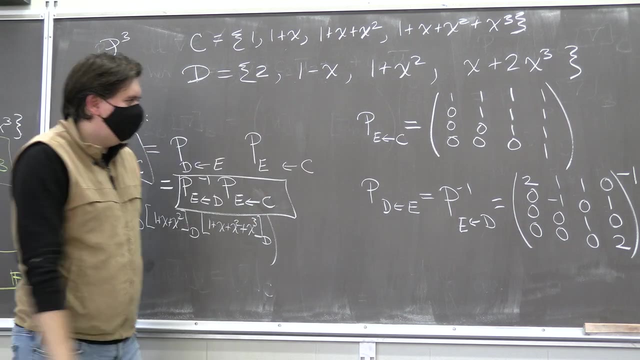 into my standard basis, Because if I know how to change things into my standard basis, then I can change between any two bases. right, Okay, But let's say, do your calculator, because we're gonna check this result in a second. 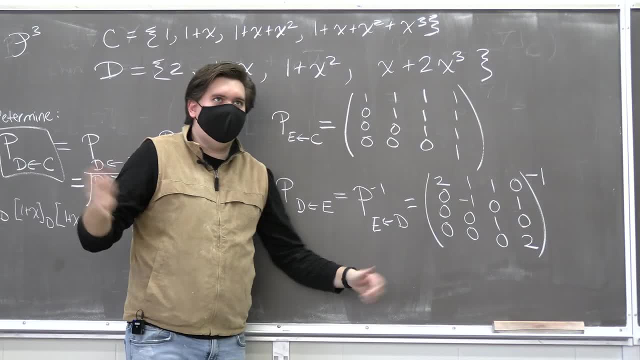 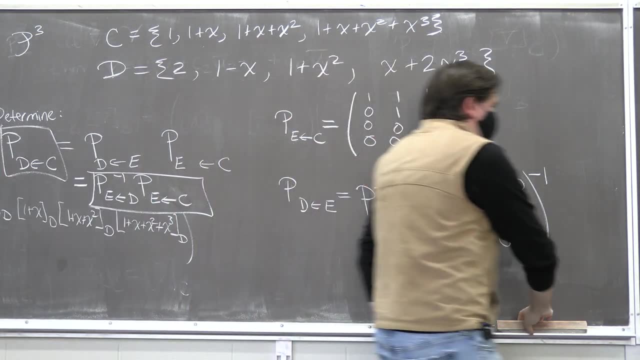 but let's say you don't have any technology. Given the rate the world is going, you can imagine some apocalyptic events, I don't know, nuclear warfare or whatever, or alien visitation that wipes out all technology. This isn't inconceivable at this point. 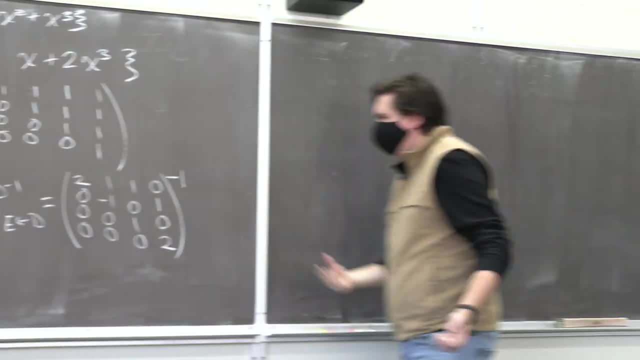 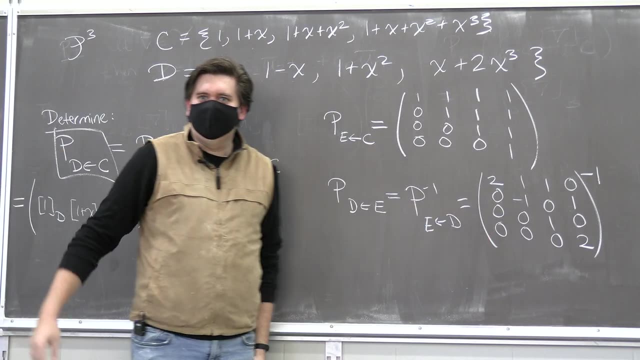 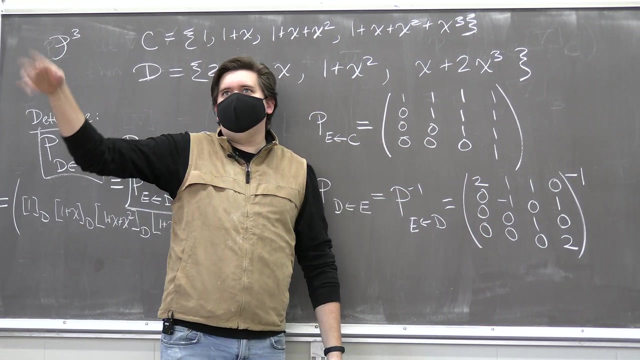 So if you don't have technology and, like the fate of the world depends upon you moving between two bases, so you really need to calculate an inverse of a four by four matrix. very plausible situation. how do you do it? Well, there's some long formula that involves: 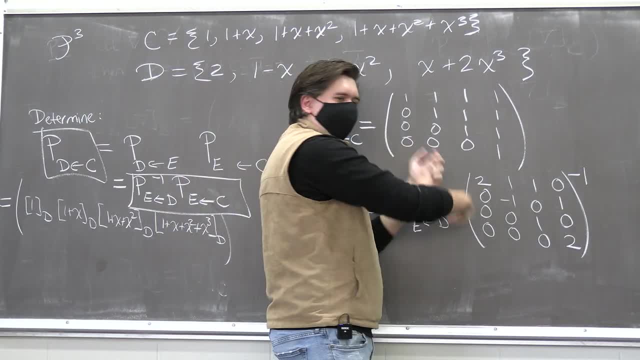 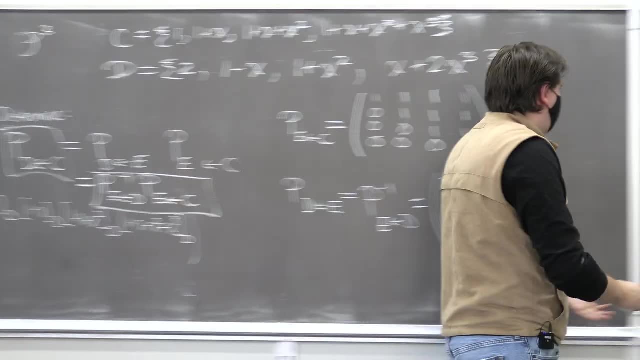 going across some row and expanding and finding, like minors and remember some of this, doing this by hand. That's a pain. what's the better way to do it? The better way to do it is like you know this inverse exists. you know it's gonna work. 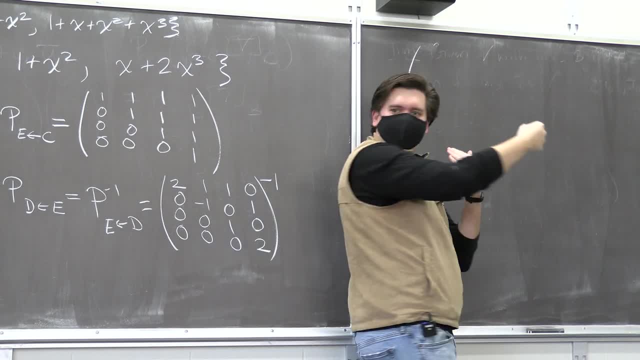 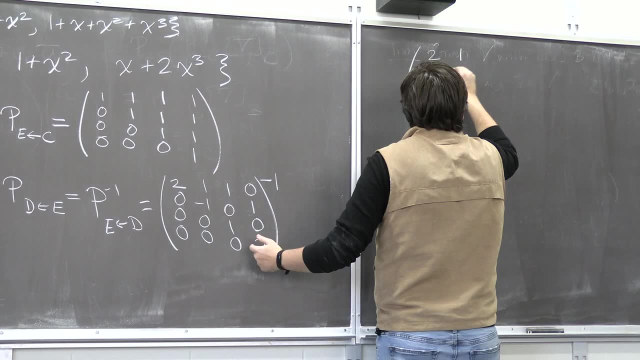 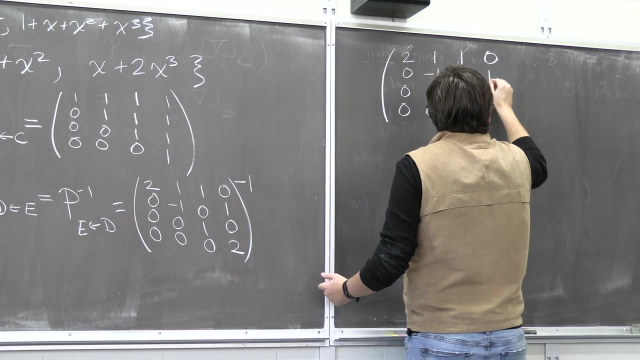 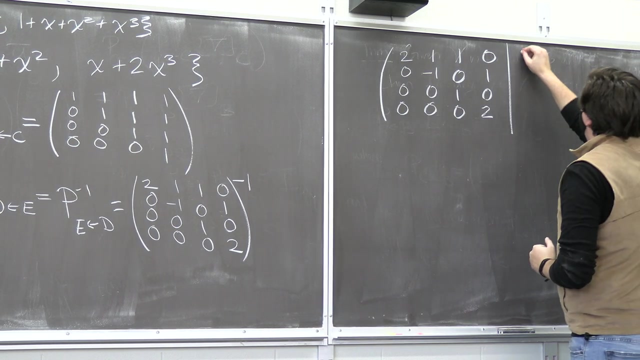 What you can do is you make an augmented matrix. Have you seen this before You make the augmented matrix, where you put the matrix you wanna invert right here, And then we're just gonna draw a line to separate that, and then here we're gonna put the identity matrix. 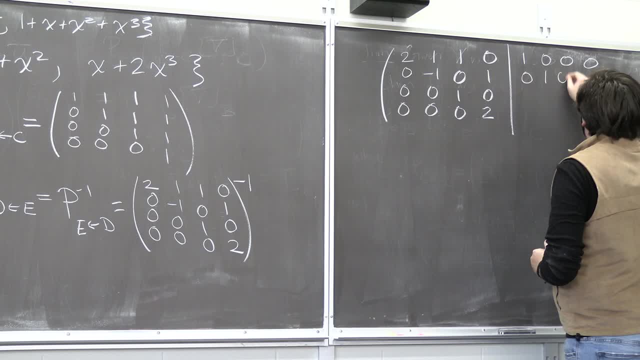 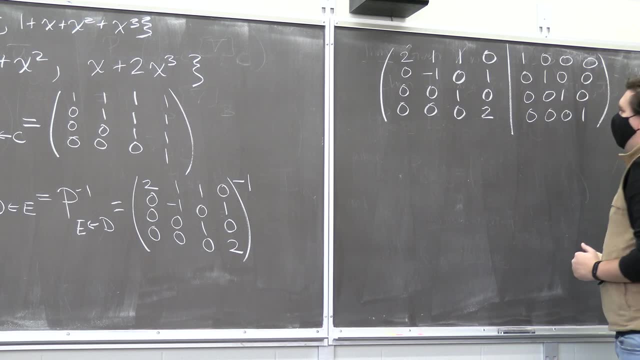 One, zero, zero, zero, zero one, zero, zero, zero, zero one, zero, zero, zero, zero one. And now what we're gonna do is we're gonna use row reduction. do you remember some of this? 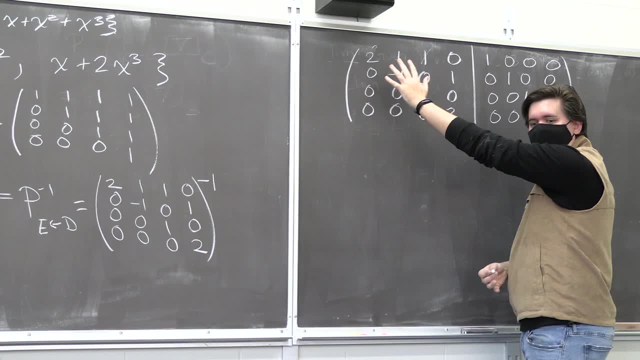 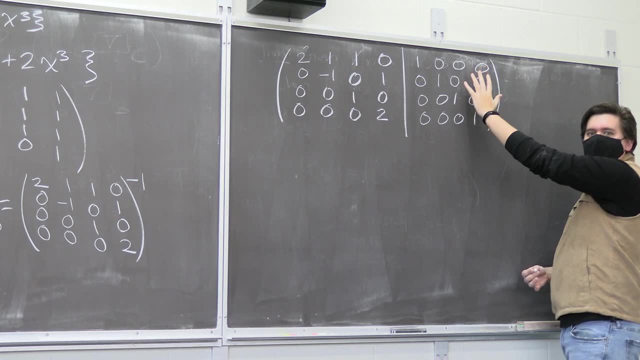 From your first course on algebra, We're gonna row reduce this guy on the left keeping track of the changes on the right and in the end he'll be the identity and he'll be the inverse right. So the procedure is: you begin with some matrix M. 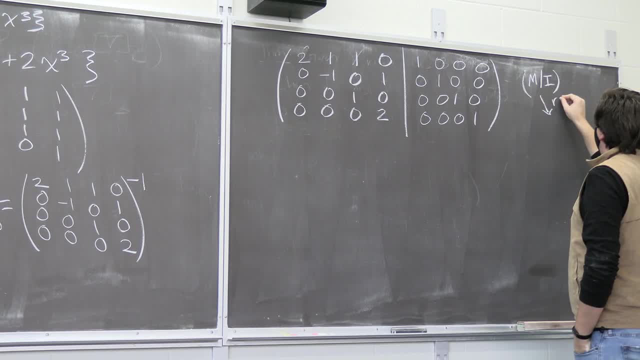 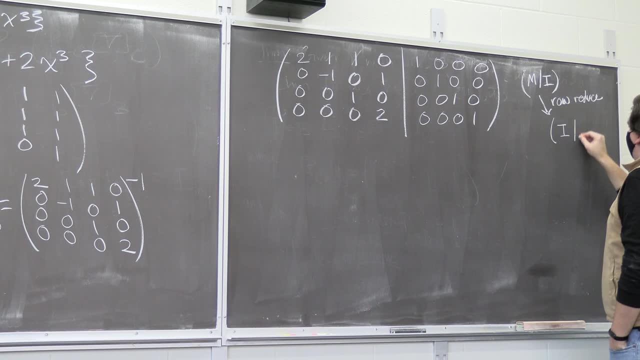 on the right, you put identity, you do row reduction, you row reduce it until you end up with identity on the left and you'll have the inverse matrix on the right, And so it's worth going back remembering how this row reduction works. 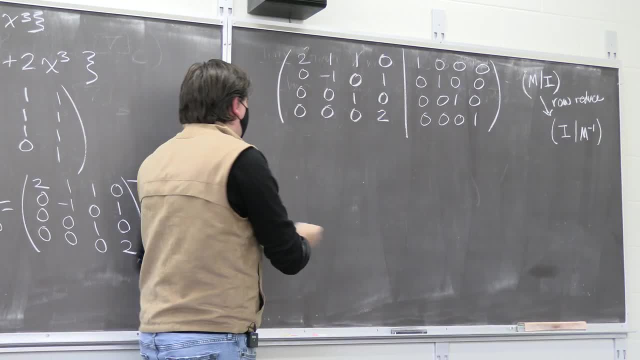 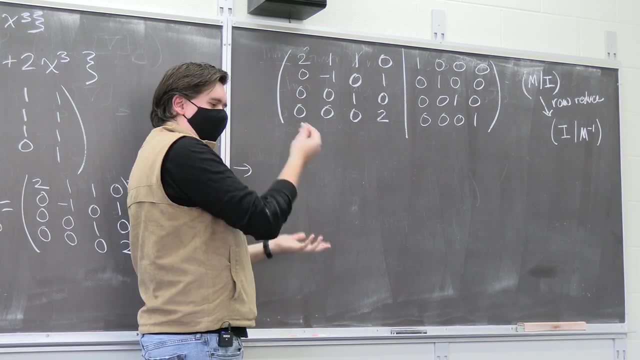 and convince yourself that really is what you end up with. But in practice, I mean, you should remember how this works. It's like we want ones all the way here. we can add rows to other rows and we can multiply by scalars, right? 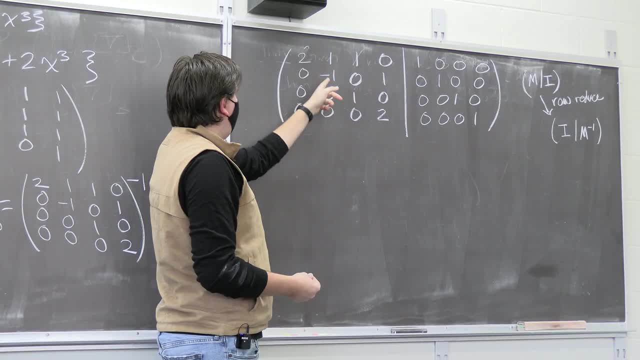 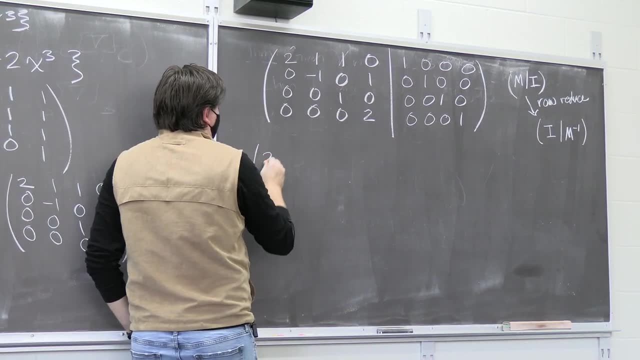 So it's like: okay, I wanna get all these things to be zero, so maybe I should add a copy of the second row to the top row. So if I add a copy of the second row to the top row, he's now two, he becomes zero. 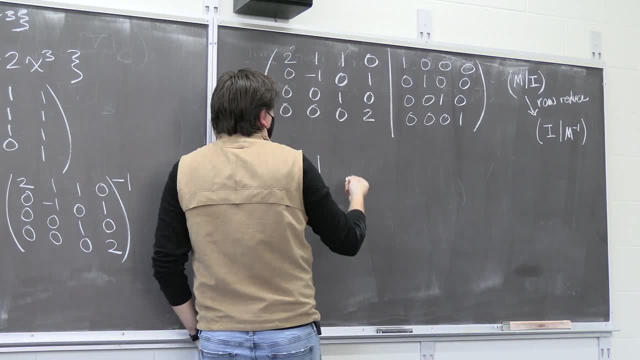 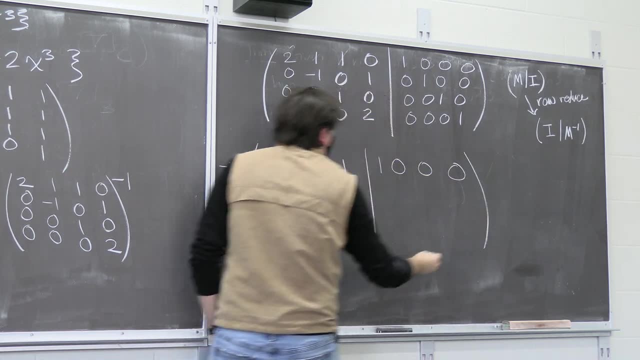 add zero, so he's still one. add one, and he's now one. and add a copy of the second row to the top row. And very good, I had a copy of the one right here, so he's also one. 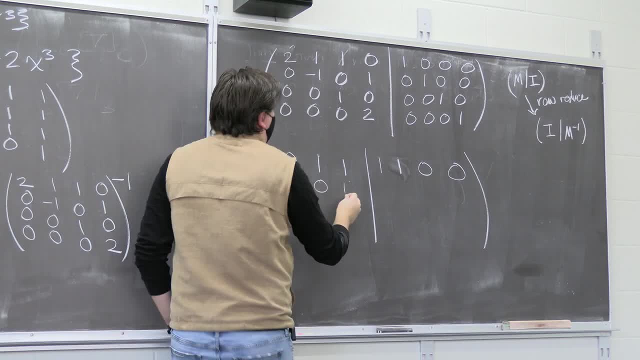 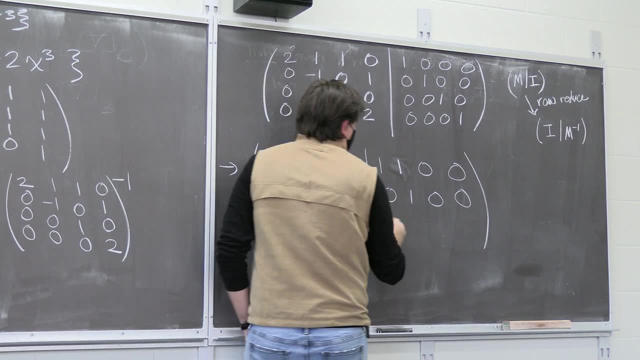 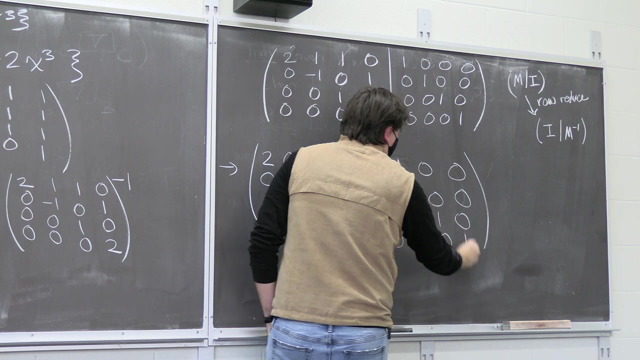 And so in the second row it's still something like this: And then I still have my third row and I still have my last row. Okay, since we're recording this on video, I'm not gonna keep redrawing the matrix. 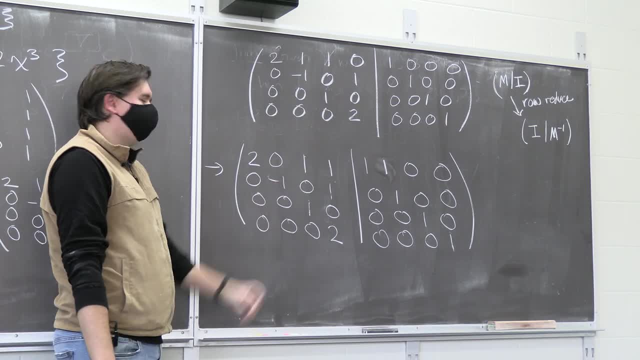 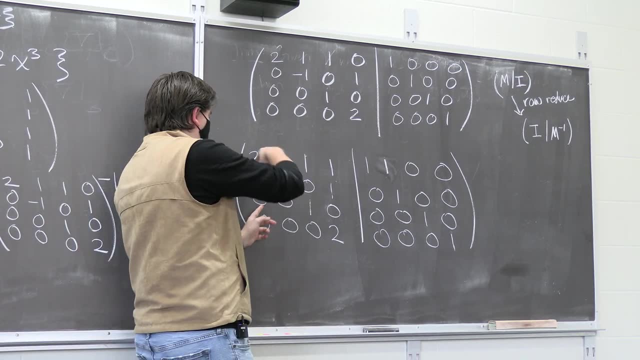 we're just gonna do it together. What do we do now? How do I get rid of this one? Subtract a copy of the third row, right? So I subtract a copy of the third row. I'm subtracting zero doesn't change anything. 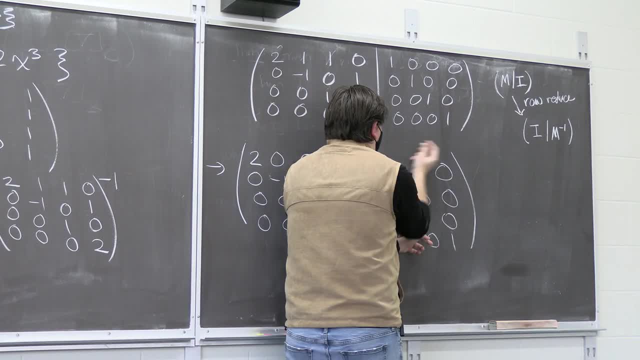 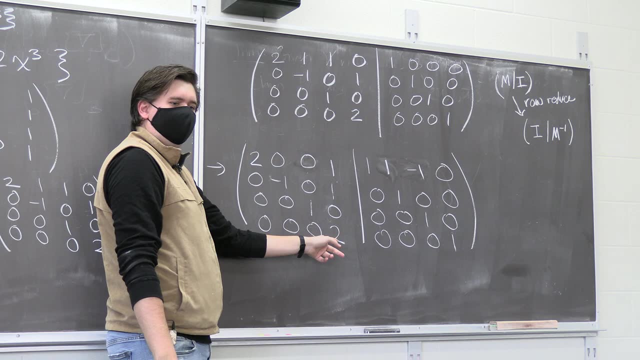 he becomes zero. he's still good, but I'm subtracting that one, so this becomes negative one. Okay, what do I need to do next? Well, I wanna get rid of these ones. let's first make this into a one, so we can clear them out. 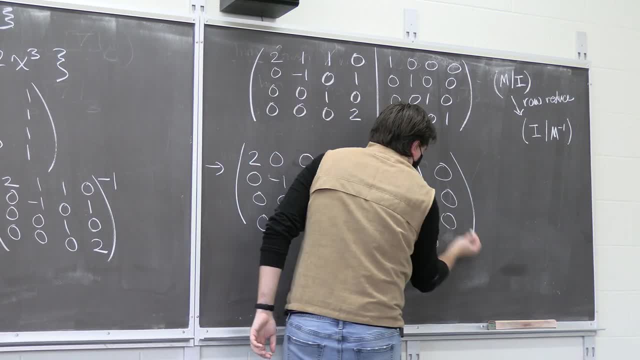 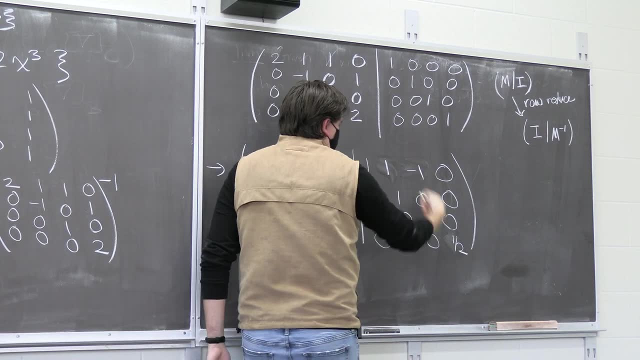 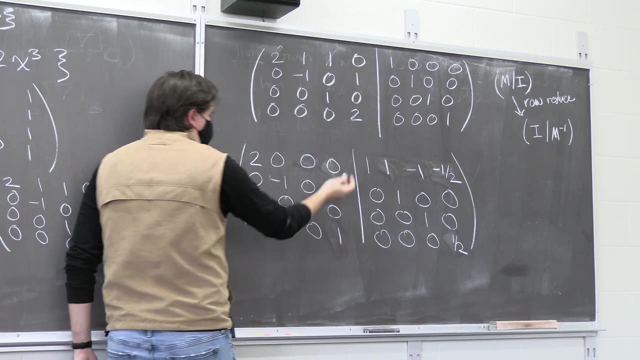 So I'm gonna multiply the bottom row by a half. Now I'm gonna subtract the bottom row from the top row so that becomes zero. these are all zeros, but subtracting that one half makes that minus one half. I'm gonna subtract the bottom row from the second row. 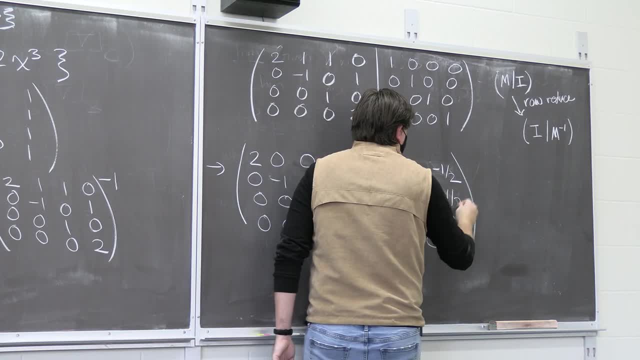 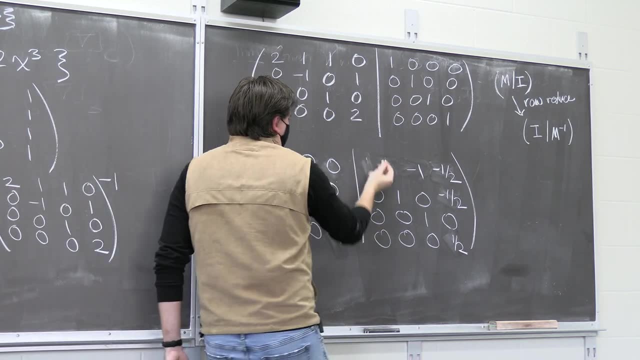 so that's zero, and subtracting one half gives me a negative one half. And now I can multiply the top row by one half to scale that down to one. so this becomes a half, this becomes a half, This becomes a negative half. 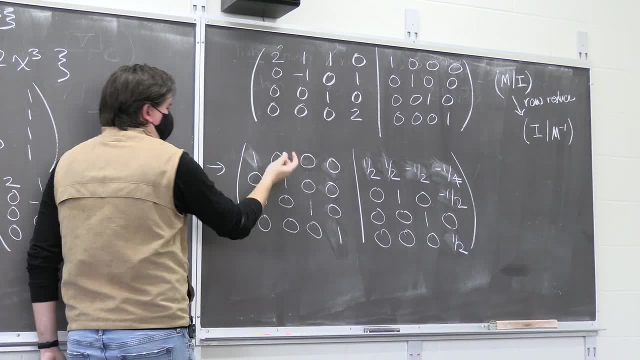 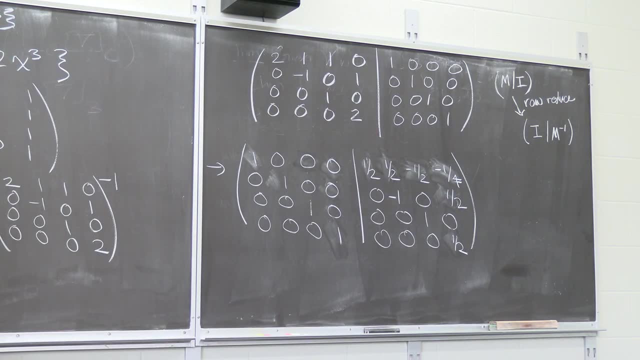 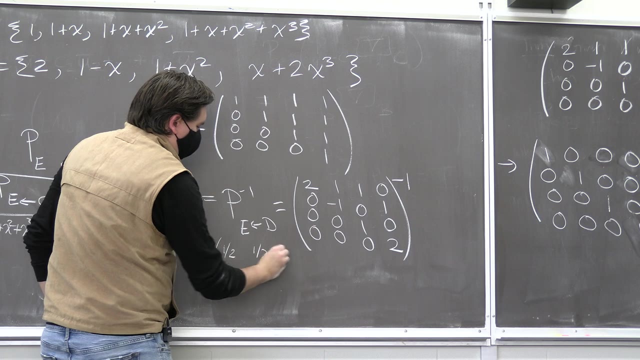 and this becomes a negative fourth. And I'll scale the second row by negative one to make this him. So what is the inverse of that matrix? The inverse of the matrix is just the guy on the right. It's one half, one half negative, one half. 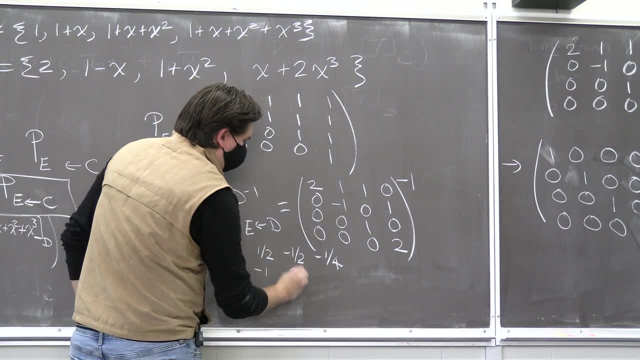 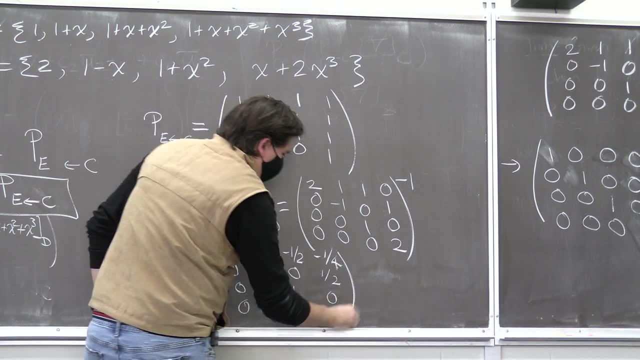 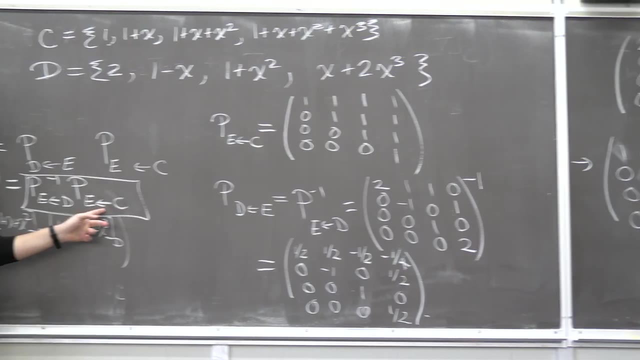 negative, one fourth zero negative, one zero positive, one half zero, zero, one half zero, zero, one half. And the claim is: if you multiply this matrix by this matrix, you recover the change of basis matrix. We can check it really fast. 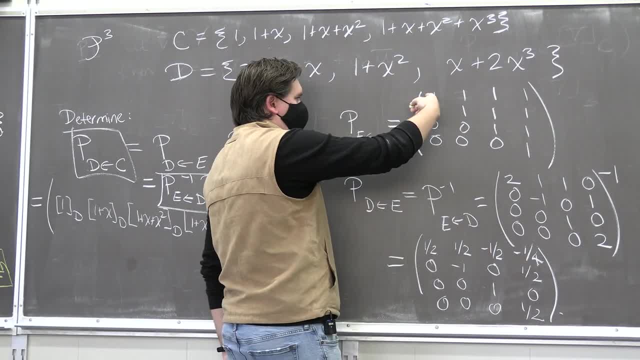 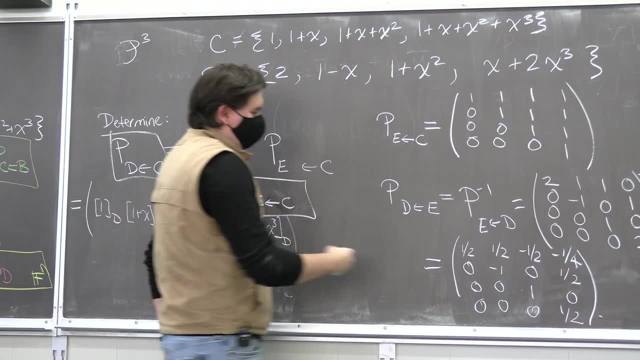 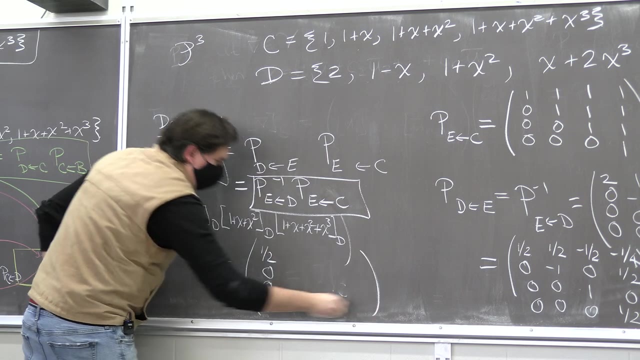 but let's just multiply the first row by the first column. What do we get? First row by first column- we get one half. And if you multiply the second, third or fourth, fourth row by the first column, you get all zeros, which agrees with what we said. the first column: 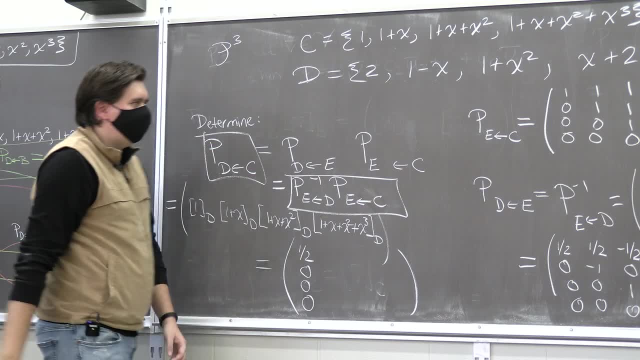 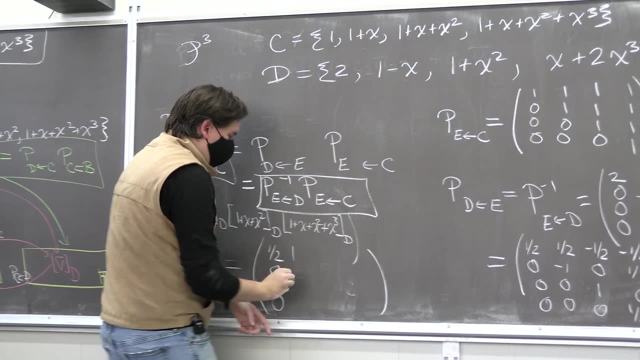 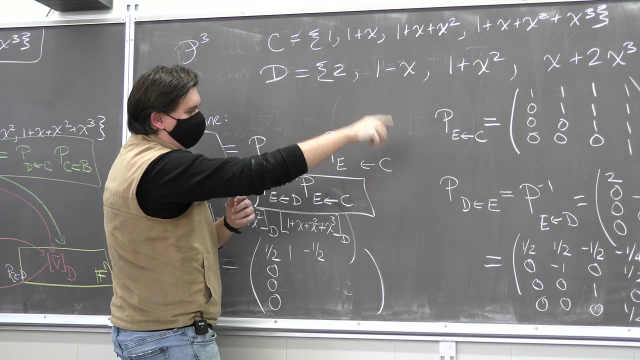 should be right. You can continue to multiply this out if you want to. I feel this like obsessive need to do it really fast. So, multiplying out the second one, we get one. The next guy gives us negative one half. The next one gives us positive one. fourth, Going down to the second row now. 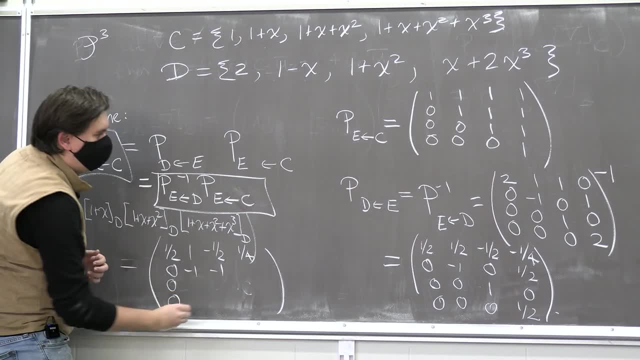 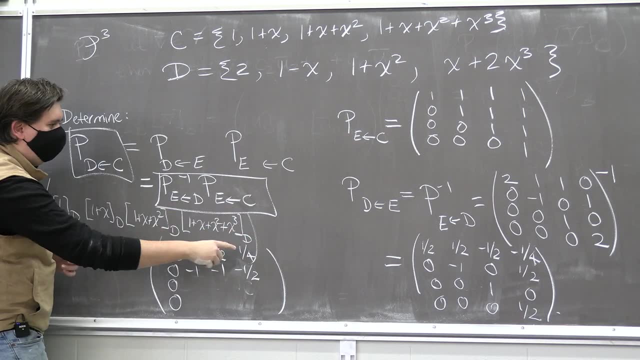 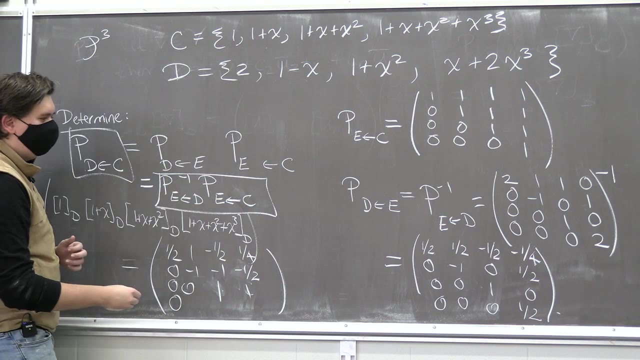 I'm getting negative one, negative one. Help me out if I make a mistake. Negative one: half Going down to the third row: we have zero, zero, one, zero, zero, one one. Going down to the last row: we have zero, zero, zero. 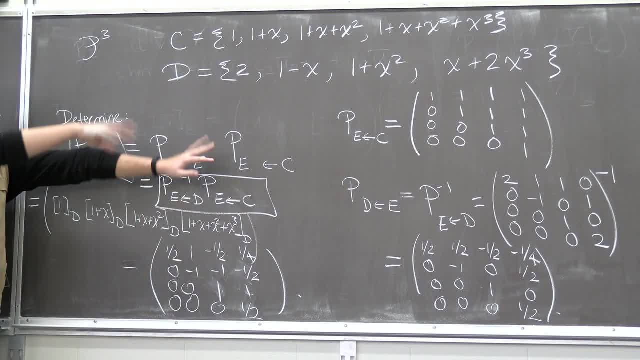 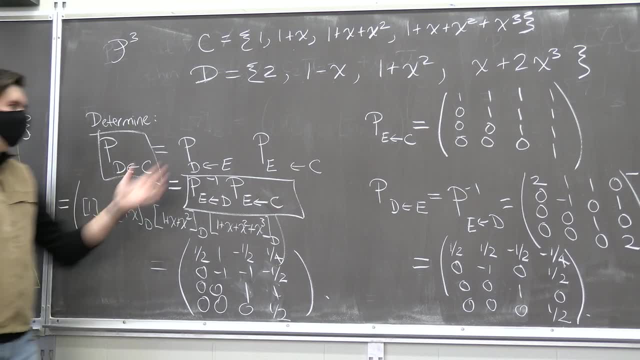 Zero, zero, one half. Very likely there's a mistake in there, but you can do the multiplication yourself and verify. But there you go. Maybe it would have been quicker to do the systematic equations, but here's a general procedure And these things are very computationally inexpensive. 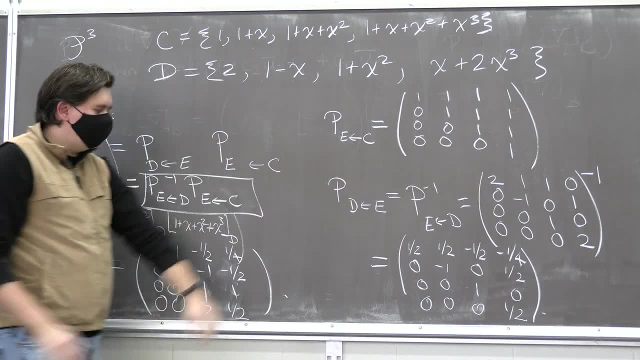 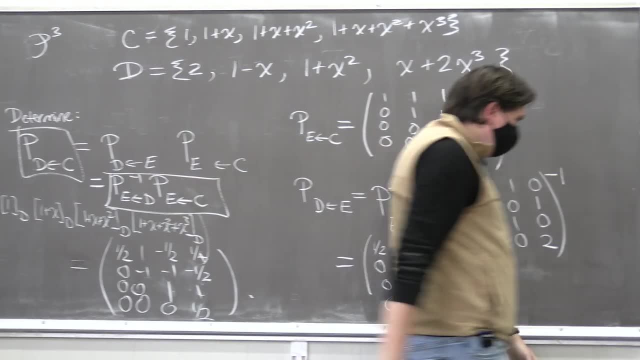 to find matrices and their inverses. So in practice you could program a computer to do something like this very easily. We'll stop there for today. Thank you.